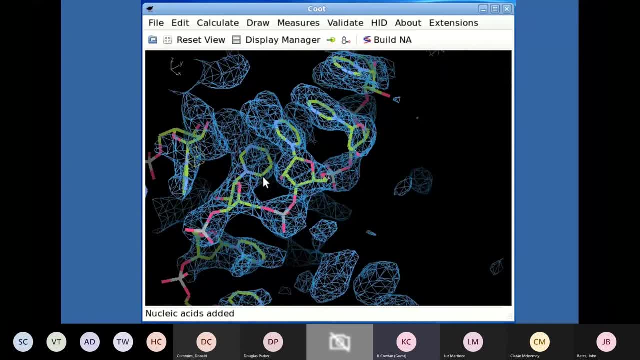 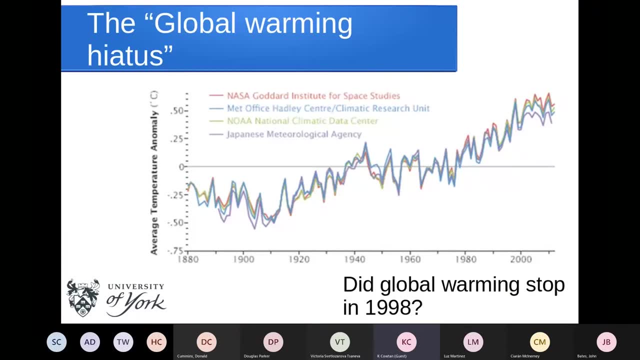 field also turn out to be relevant to other topics, And I tend to get like many autistic people. I get special interests And I became very interested in the global warming hiatus, Okay, Which was this period from around 1998 to 2013,, when there was a great deal of attention. 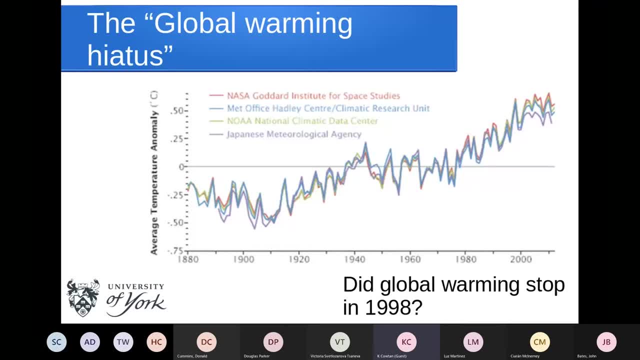 in the media and also in the scientific literature to the question of whether global warming had stopped. So here's a picture from that period. I don't know if you see my mouse- If it's like Zoom, then you do- Where we can see that, depending on which record you were. 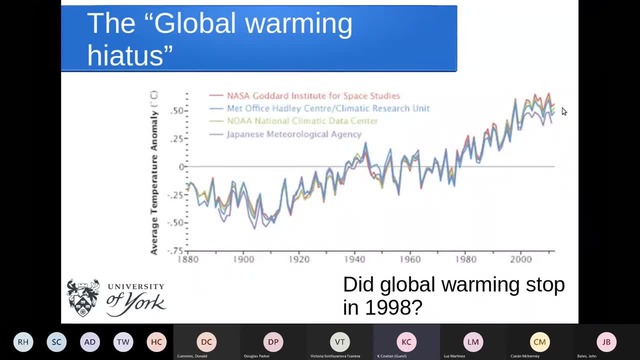 looking at It looks, to a greater or lesser extent that there has been a change in the rate of warming, that it had slowed down during that period. Now, of course, if you looked at the media attention and, in particular, discussion from sources which had particularly strong political views, they were drawing a lot of conclusions. 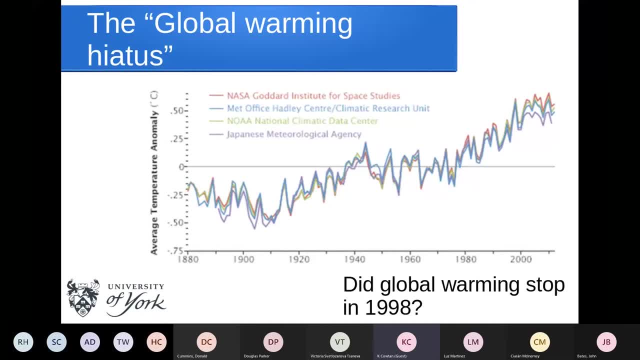 from this. Okay, They were drawing a lot of conclusions about whether we needed to do anything about global warming anymore, or whether the problem had gone away, And having to do things corporately is something that, of course, presses political buttons, and so suddenly they developed an 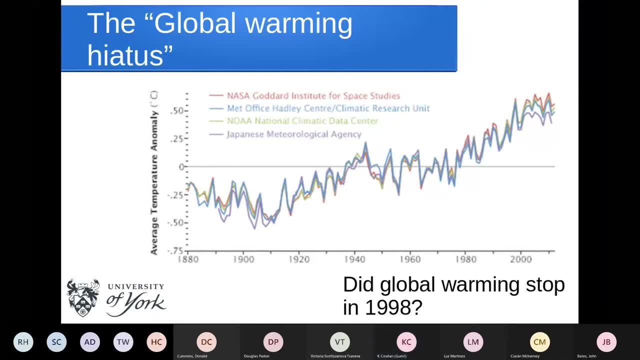 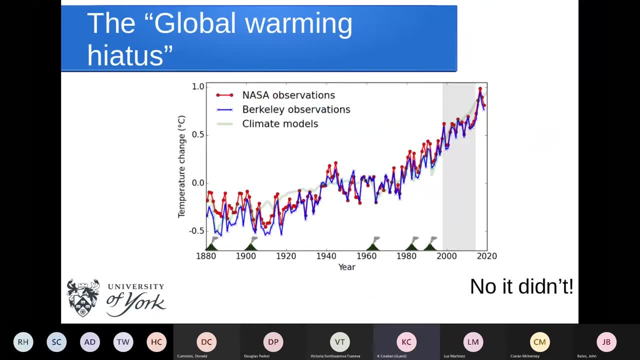 interest in commenting on the science. But did global warming stop in 1998 for a while? Well, of course, if we add a few extra years of data, then it becomes very obvious that no, it didn't. But could we have known that at the time with more confidence? 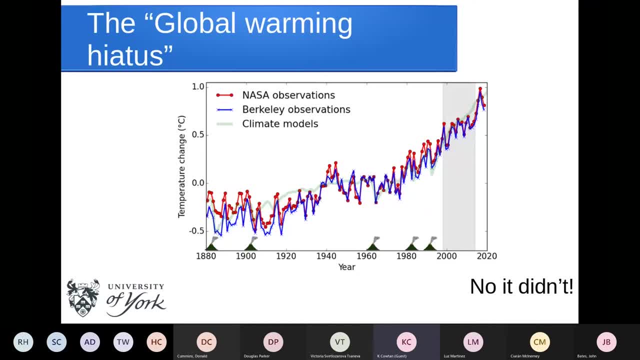 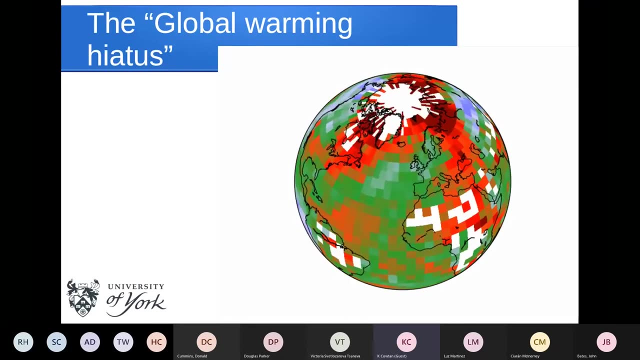 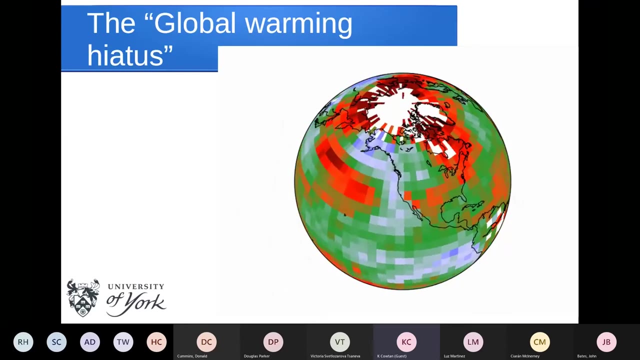 So I became interested in this problem because of a particularly prominent feature of the data which stood out to me, which I'll show in this animation, which shows a temperature trends in different parts of the planet. And this is the observational coverage of the Met Office data set And you can see the colors represent trends. warm colors are faster. 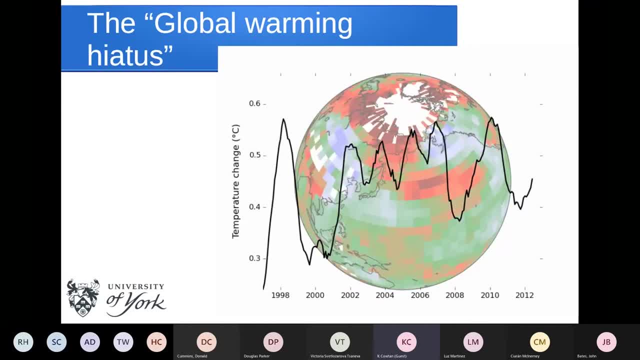 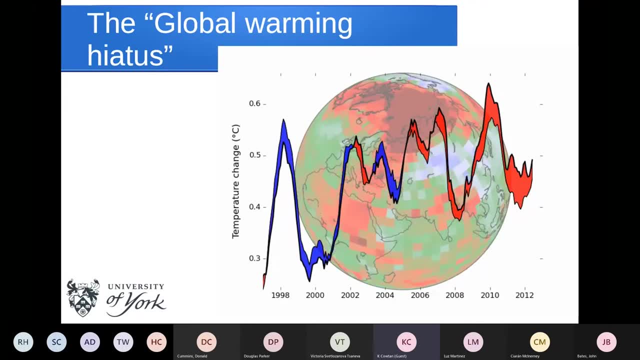 warming And you can see that the coverage of the Arctic is poor and also that the Arctic is the fastest warming region of the planet And there are other regions with poor data coverage which, as it happens over that period, are also faster warming. 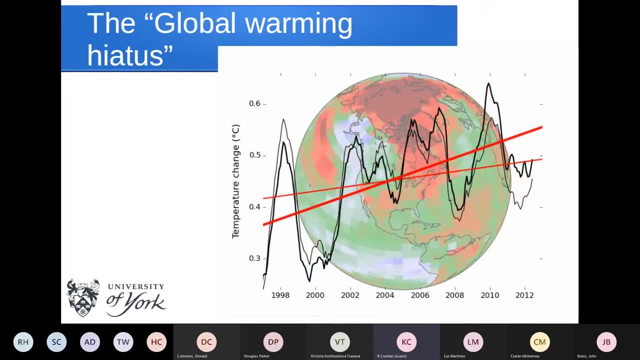 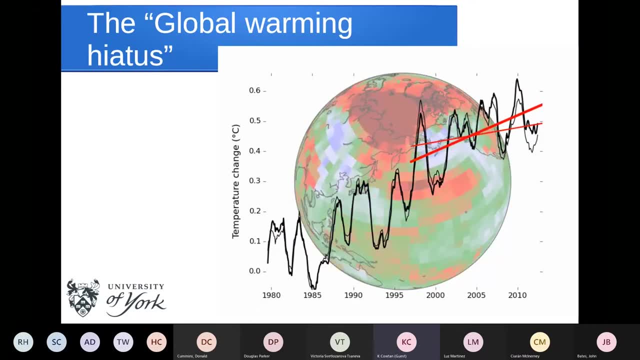 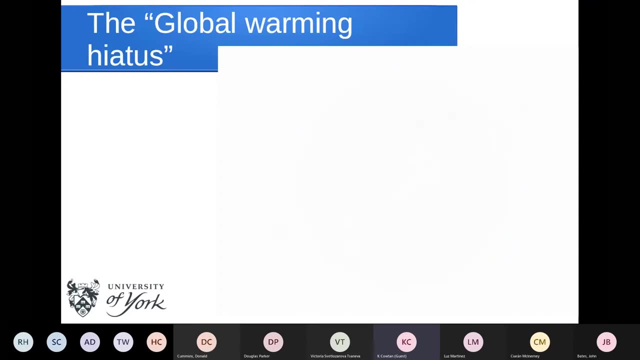 And so I did some initial work on that area which was creaking, which is a form of Gaussian process modeling, to infill the gaps in the data and see what that did to the trends, And we found that a lot of this supposed slowdown in warming went away. 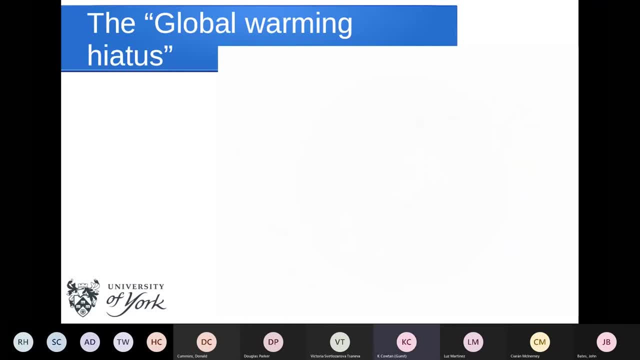 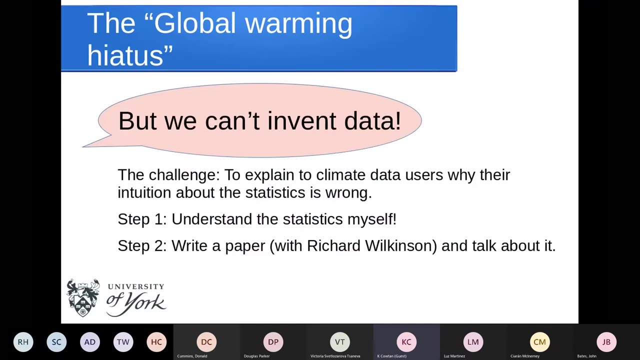 So that became my first climate paper, the first excursion out of crystallography. But the response from the climate science community was interesting. So some very senior figures said, and many more junior ones said we can't invent data. That was their interpretation of this approach of infilling the missing regions. Now this: 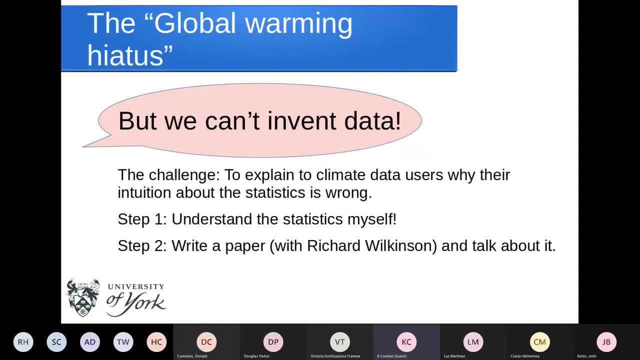 seemed to me to be problematic. I'm using this as a statistic. I'm using this as a statistic And the statistics that we knew was wrong because of this rule of not inventing data which they had raised seemed to be a problem. 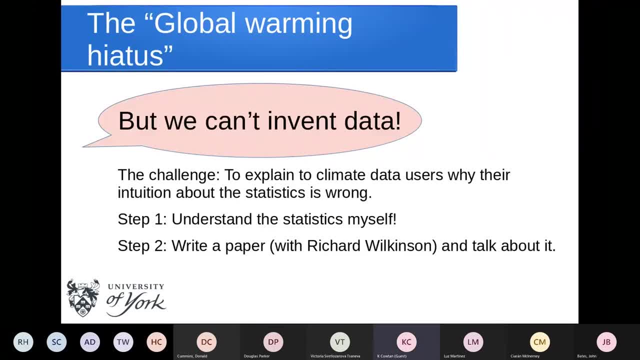 So the challenge for me was then to explain to climate data users why their intuition about statistics was wrong, And the first step was therefore to understand the statistics myself And then go on to write a paper for which I put on a real statistician who could fix. 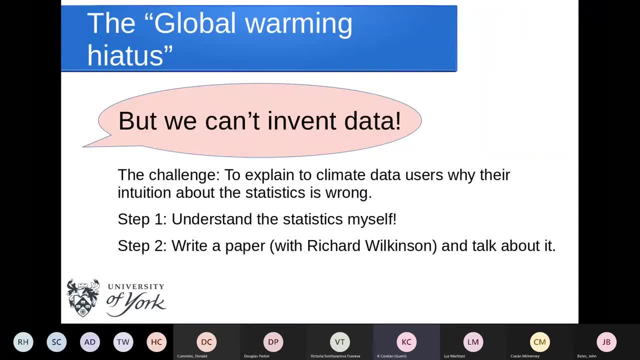 some of my errors, Richard Wilkinson, who's now at Nottingham, and then talk about it, And what I'm going to show you in the following slides is the talk I gave. There's also a version of it on YouTube And they took it to a few sites around the UK. 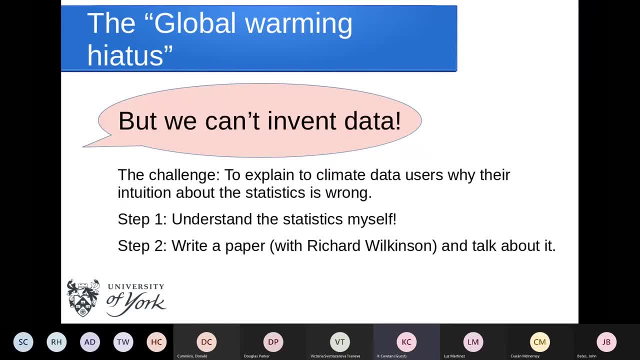 Now the problem here is an interesting one. We know from dealing with science denial that correcting misconceptions is much harder than teaching people new things in the first place, And this is really a problem of correcting misconceptions. So this talk was very much built around the idea of using simple concepts that people 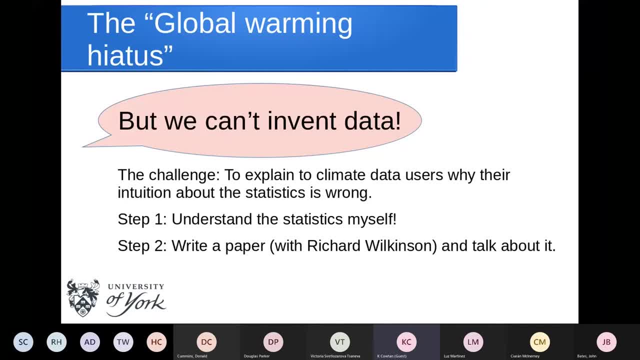 already knew, to show them how their intuition could lead them in the wrong direction. So it's a problem of science communication to scientists and also of misconception-based learning. So this is the kind of talk I gave. So what is there to know? 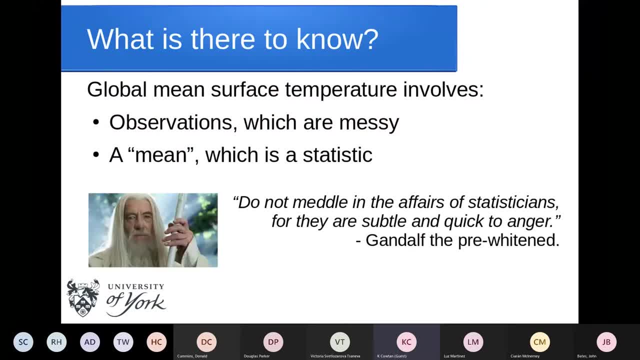 What's our starting point? Global media, And it's a very interesting topic And it's a problem, of course, because we know that there are many, many different ways to measure global warming, And we'll talk about that in a bit. But first of all, there are two main factors that I think we should look at. 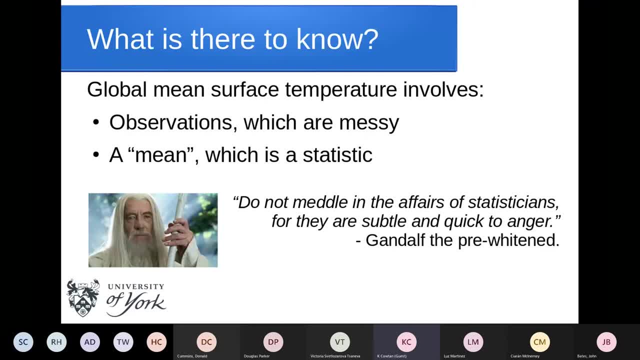 The first is the global mean surface temperature. So this is a metric which we're looking at because it's a commonly used measure of global warming and is used to draw inferences about what we need to do in terms of political or social action. 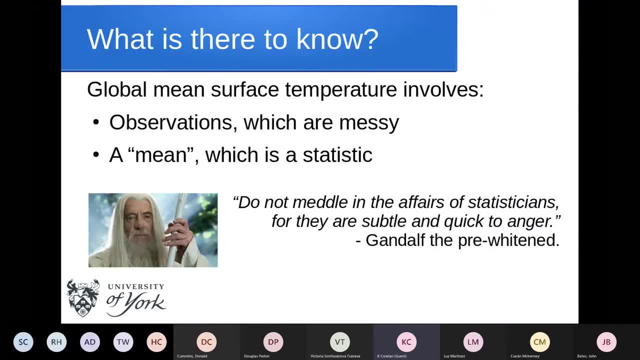 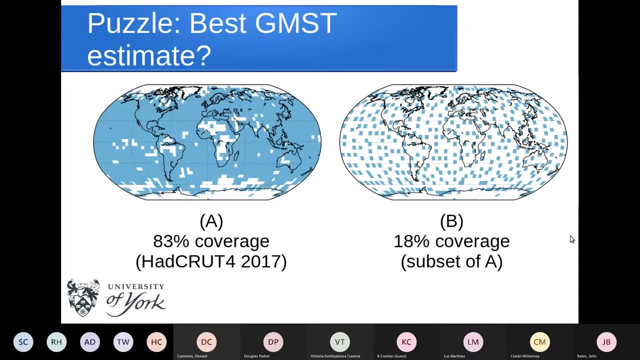 Now this involves observations which, as in any field of science, are messy, And it also involves a mean. It's in the title: Global mean surface temperature- statistical humor. you can probably do better, So what I'd like to do now is start with a puzzle. 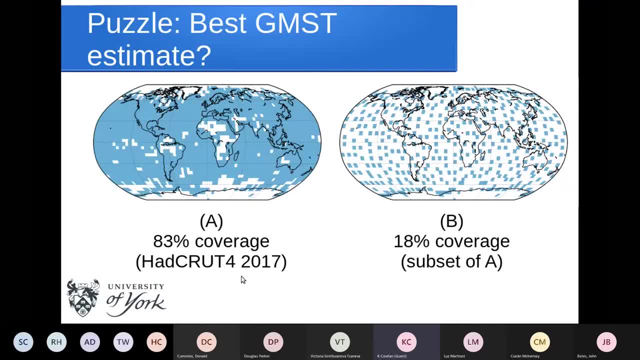 So one of the data sets we use for assessing global mean surface temperature is a data set from the UK Met Office called HADCRU T4. And there's a shaded region in the picture on the left shows you the data coverage in 2017.. I can't remember which month, probably January. 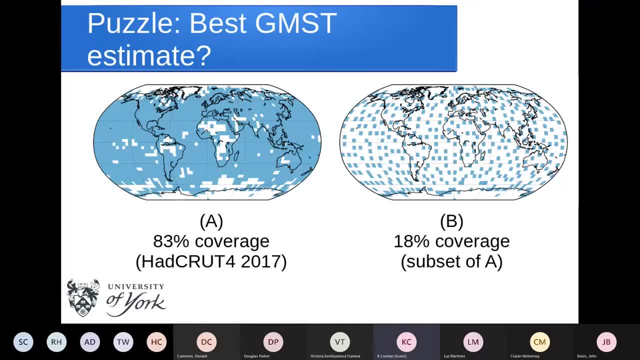 And it's covering about 83% of the planet And it's a gridded data set in five degree boxes. Now my question for you is: if we are simply to calculate an area weighted average of all the regions where we have observations, then do we get a? 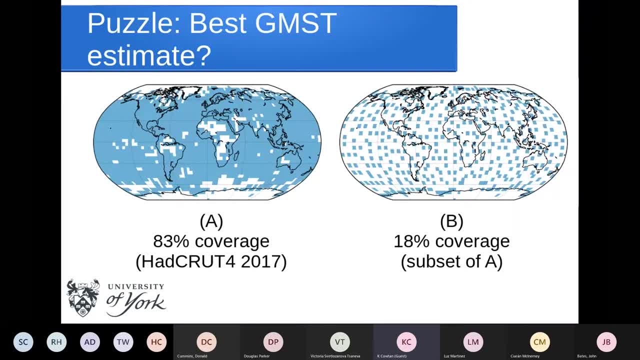 better estimate of the true global mean surface temperature from using just the shaded regions on the left, with 83% coverage, or by using the shaded regions on the right, where we only have 18% coverage and it's a subset of the coverage on the left. 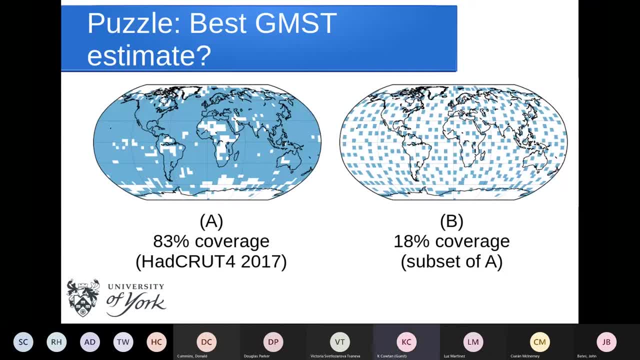 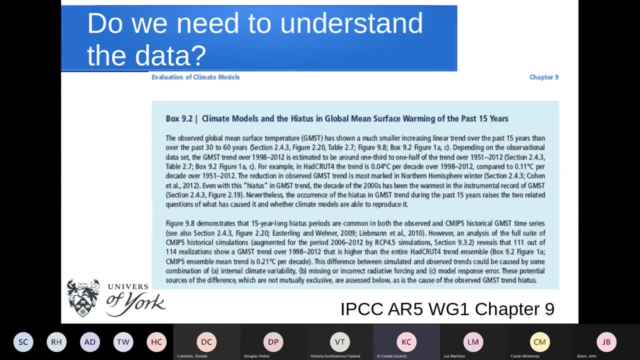 So there's a question. if you really want, you can type answers in the chat, but you've probably spotted That there is a bit of a trick going on here, But we'll come back to the question a bit later. So this period, this hiatus, period of warming, got a lot of attention in the media. 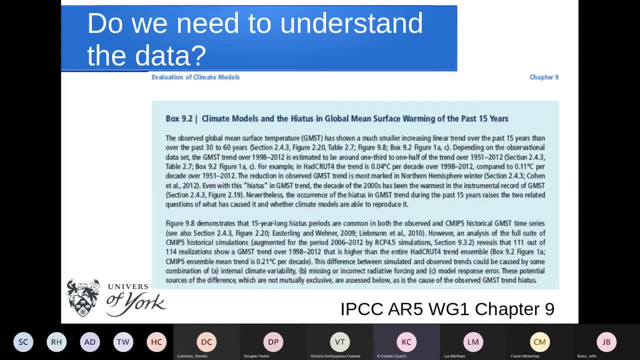 but also in scientific literature. There were many papers published on it, but also in the IPCC assessment reports, So this is from The fifth assessment report. there's a box in chapter nine and another one in chapter two on this supposed hiatus in warming, And I'd like to highlight a few things. 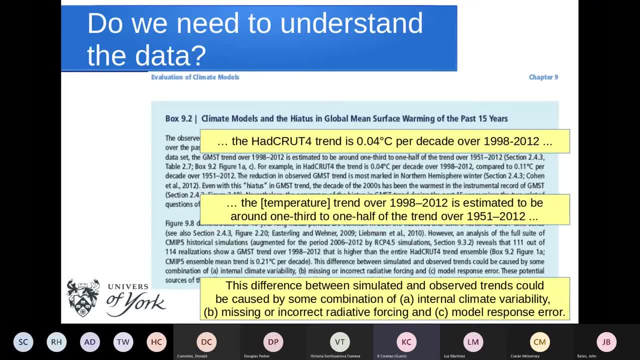 that this box says. The trend in the HADCREW T4 data set is 0.04 Celsius per decade over the period 1998 to 2012.. And that's estimated to be a third to a half of the long term trend. 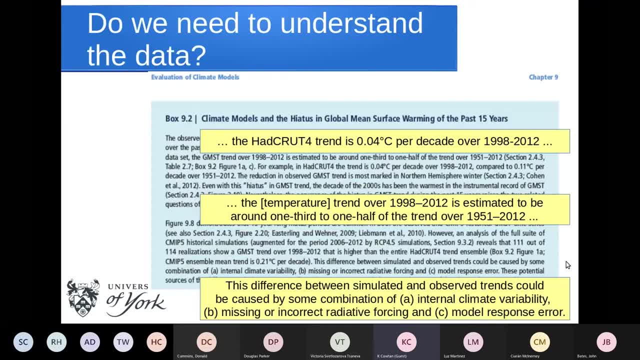 And then it goes on to give us some explanations, possible explanations for this observation, And it suggests that this could be down to internal climate variability, in other words, weather. It could be problems in the numbers, the atmospheric compositions which were being fed into climate models. 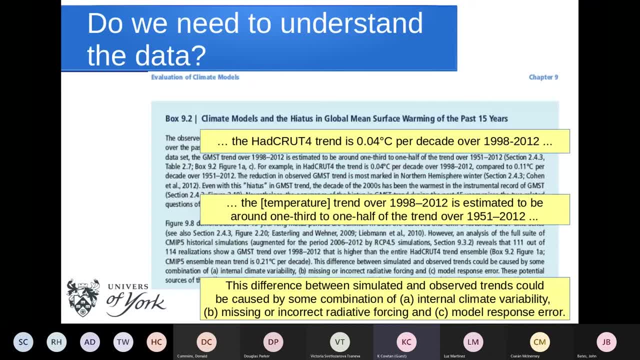 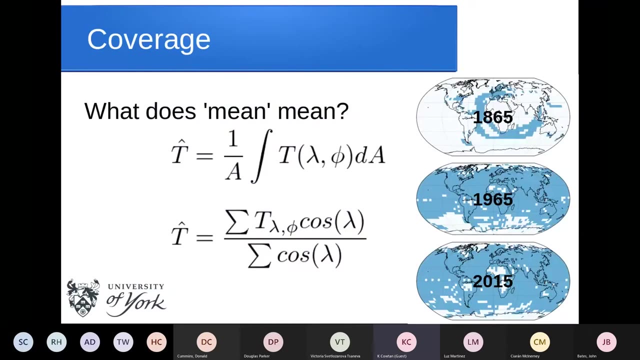 or an error in the models. It could be problems in the environmental response to those influences. Now the interesting thing that's missing here is anything to do with problems in the data. So that's interesting and kind of relevant. So let's go back to basics. What does mean? mean in this context? 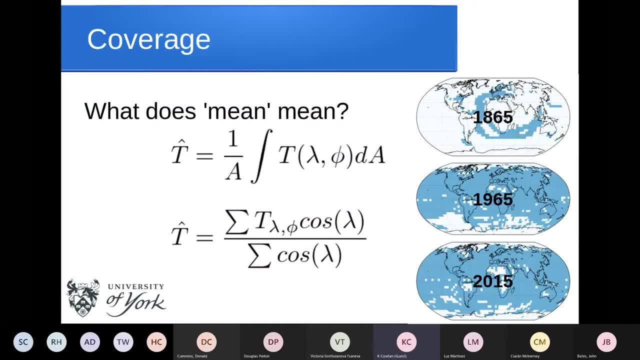 So I think if I were to give you a little bit of an idea of what it means in this context, So I think if I were to give you a little bit of an idea of what it means in this context, if you were to do the phrase global mean to surface temperature, then most of you would immediately interpret it as something like this: 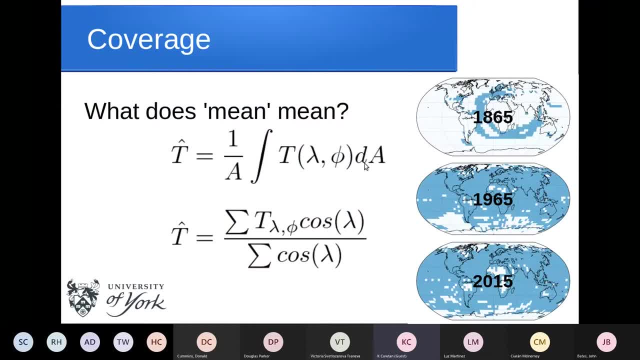 The integral of temperature over longitude and latitude integrated over area, And to form an average we divide by the surface area of the Earth. Now, because we're dealing with gridded data sets, then this becomes a summation of the temperature in each grid box. 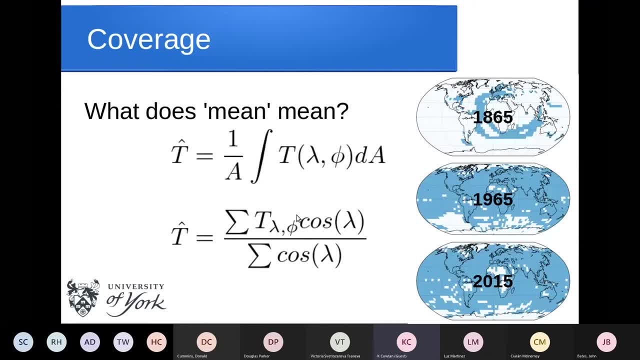 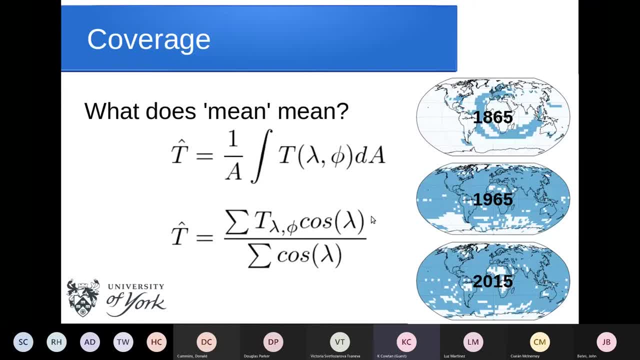 Climate scientists refer to this as a cosine weighted mean And it just gives you the effect of an area integral, with the area of each grid box included, And you can see some examples of the data coverage for different periods in the 19th century. 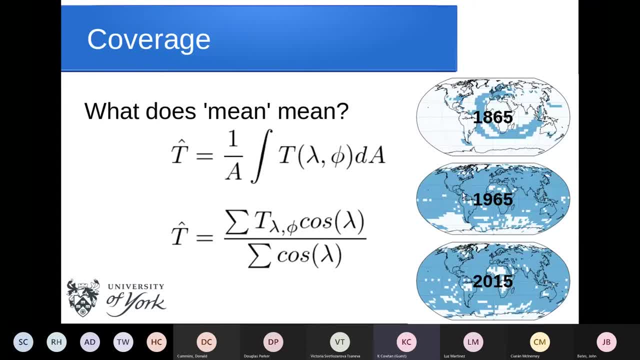 It's rather limited. By the time you get to post-World War II, we've got reasonable coverage. And once we get to post-World War II, we've got reasonable coverage. And once we get to post-World War II, we've got reasonable coverage. 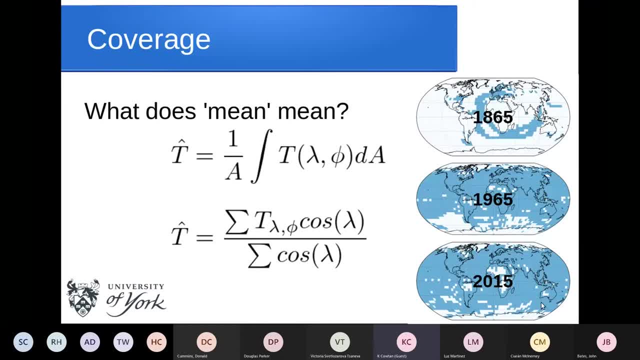 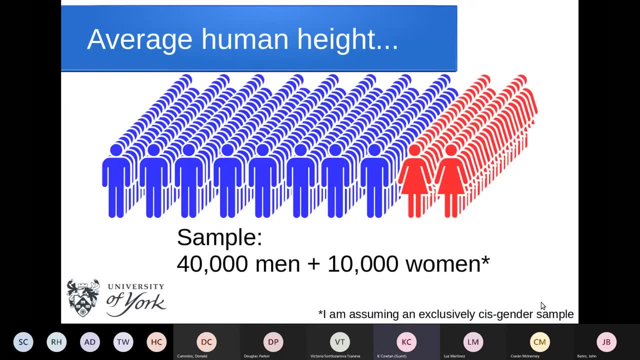 And once we get to post-World War II, we've got reasonable coverage. If you want to be like that robot boys drifting around the oceans, then it's quite good, OK, So now I want to talk a little bit about this concept of mean and how it isn't always as simple as we think. 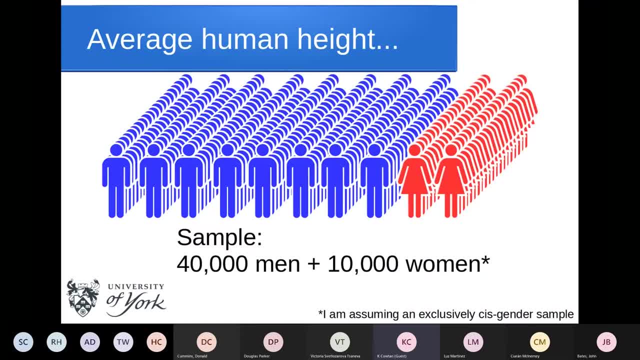 So now I want to talk a little bit about this concept of mean and how it isn't always as simple as we think. So suppose we want to calculate the average height of human beings, So we could take a sample and measure how tall they are. 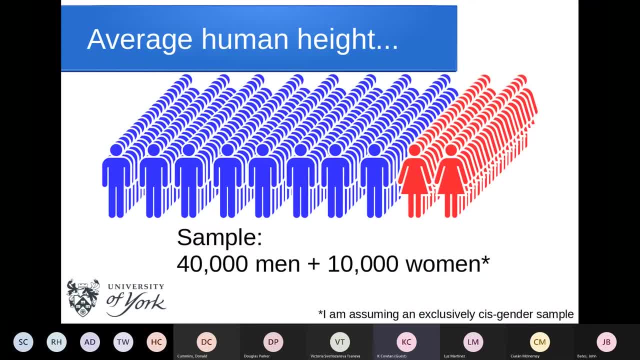 So here we've got a sample. Here we've got a sample sample with 40,000 men and 10,000 women, And I think most of you will be able to see that if we use this sample and take a simple average of the heights, then we might get a misleading. 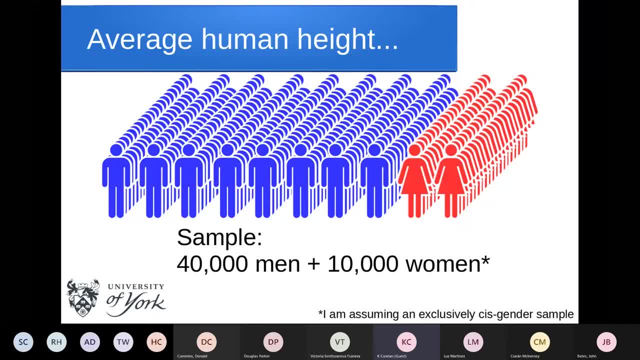 answer: because cis men are, on the whole, a little bit taller than cis women. So what could we do? Well, one very simple thing we can do is throw away a lot of observations. So if we throw away 30,000 observations of men, so we've got a representative sample. 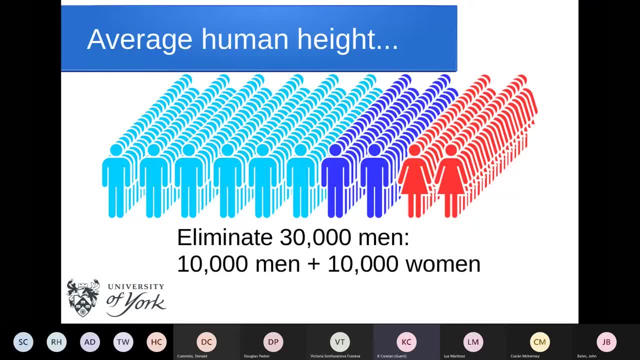 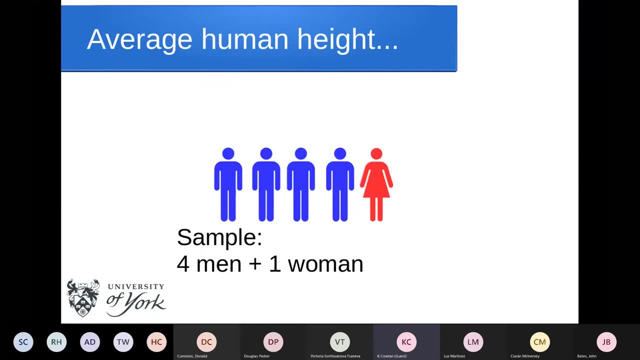 of 10,000 men and 10,000 women. then we'll actually get a better estimate of how tall people are in this case. Okay, that, I hope, is simple and obvious. Now, a slightly more tricky case: what if we have a very small sample of four men and one woman? 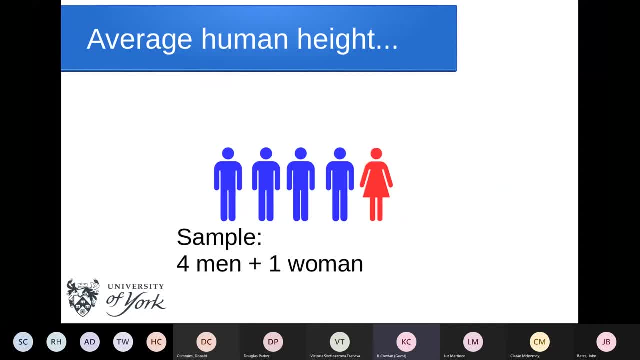 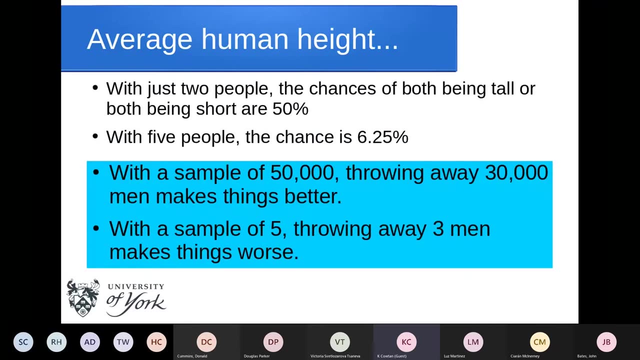 So in this case, would we be better off getting rid of three observations? So we have one man and one woman. Well, the problem is, this might actually give us a worse solution, because with just two people, the chances of both being tall or both being short are now 50%, Whereas with five. 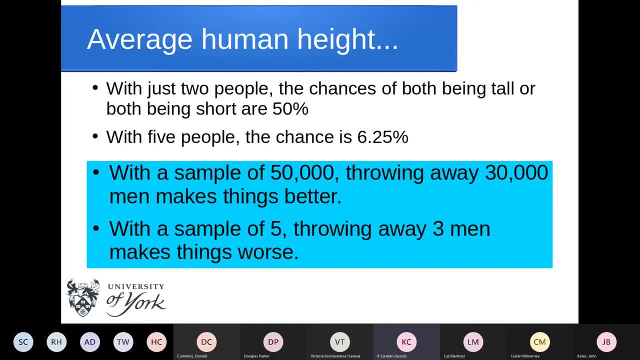 people, the chance is comparatively smaller. So with a sample of 50,000, observations, throwing away 30,000 makes things better. clearly, With a sample of five, throwing away three observations, it's far less clear that that's a good thing to do and might. 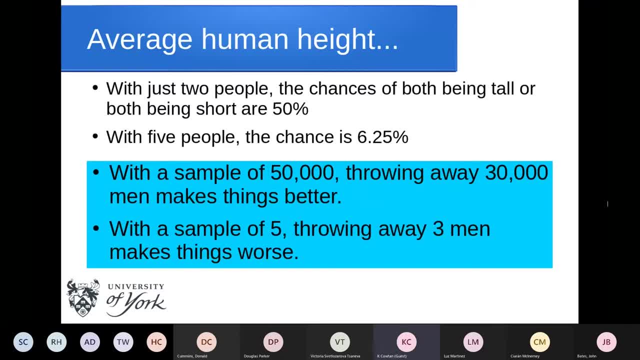 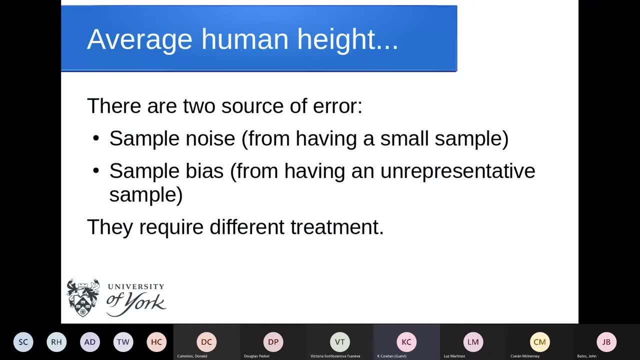 make things worse. So what's going on here? There are two sources of error here. One is sample noise, from having a small sample, and the other is sample bias, from having an unrepresentative sample, And both lead to a difference between the number we 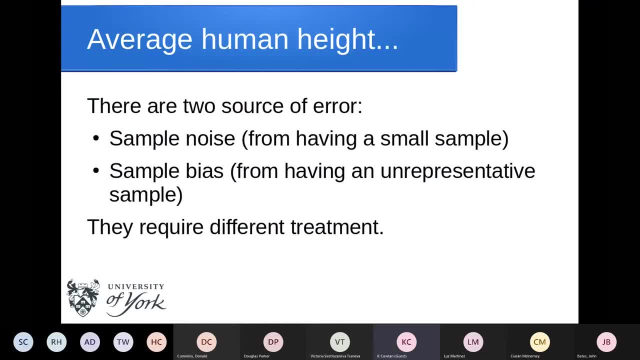 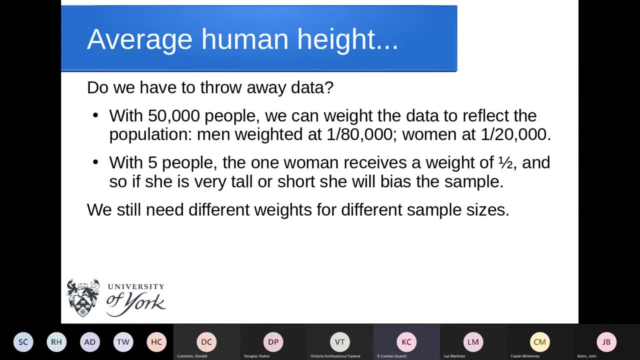 get from our mean and the true mean of the entire population, And these require different treatment. Now I've suggested throwing away data. That's not the only approach. We could instead weight the data to reflect the point of view, And we could also throw away the data from the. 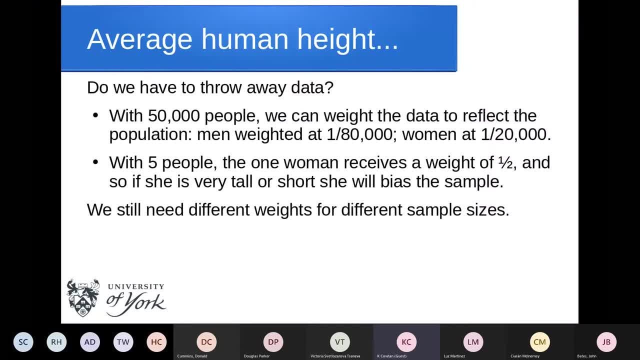 population. So if you weight the men at one over 80,000 and the women at one over 20,000, then you can include all of the observations, but the different weighting will mean that the mean that you get is representative. This doesn't make the problem go away With five people. 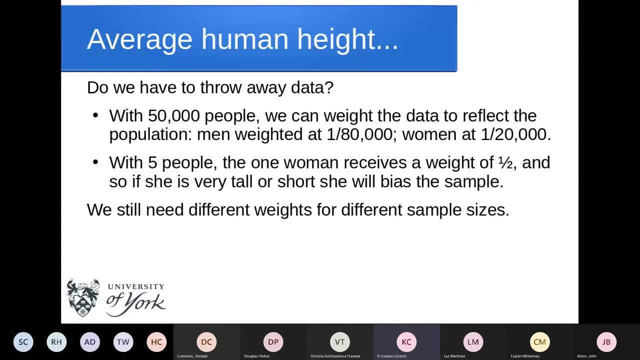 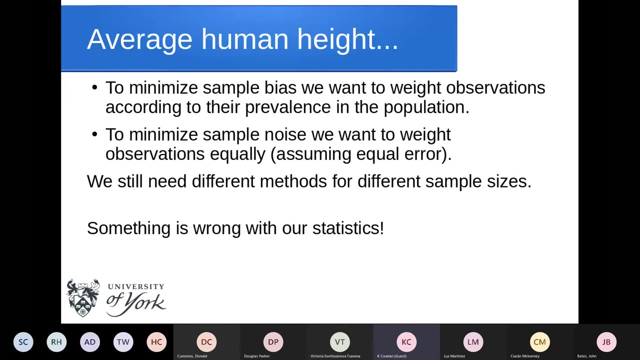 the one woman in the sample receives a weight of a half. So if she's unusually tall or short she will still bias the sample. So using weights doesn't completely solve the problem. It may help a little bit. So we need different weighting schemes for different sample sizes. So to minimize sample bias we want to weight. 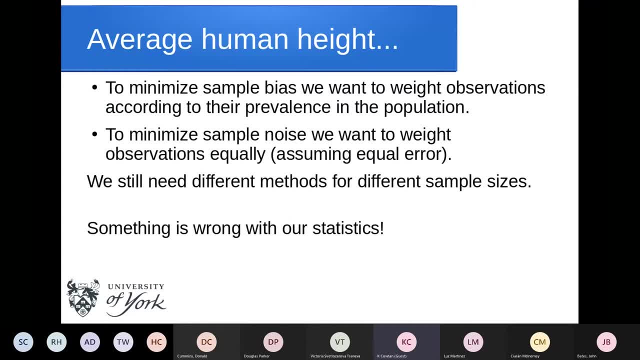 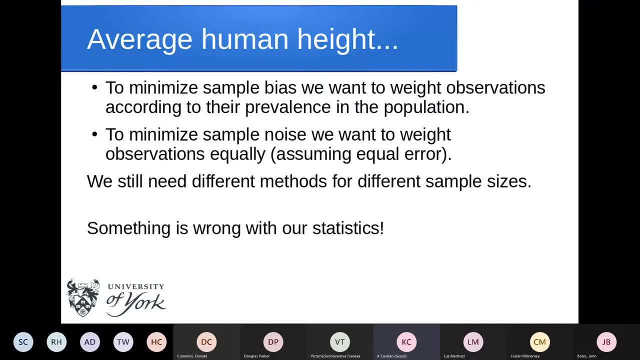 Different statistical method for different sample sizes, And that suggests to me that our understanding of what is meant by taking the mean of a sample is wrong. Okay, So what are we going to do about this? Well, what we need is a method of calculating an. 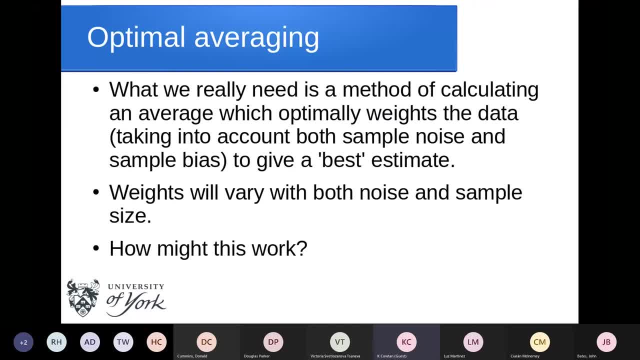 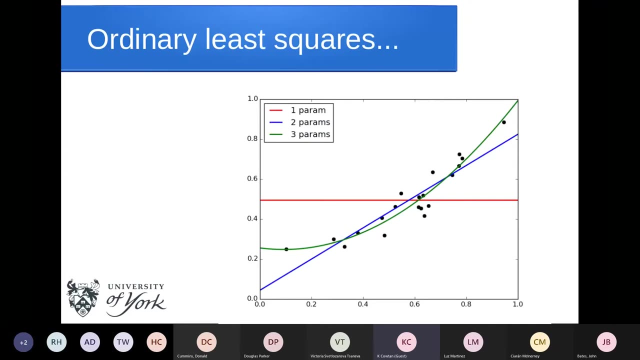 average which optimally weights the data, taking into account both sample noise and sample bias, in order to give a best estimate, And the weights will then vary both with the noise and sample size. So how might this work? So there is a technique which every scientist will be familiar. 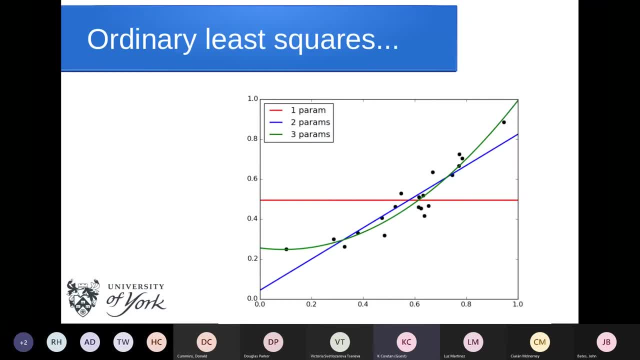 with which is ordinary least squares. So we most commonly use this to fit a straight line through data, a set of data points where we're essentially fitting a straight line through, a set of data points Where we're essentially fitting a model with two parameters. But we can fit more complex or less. 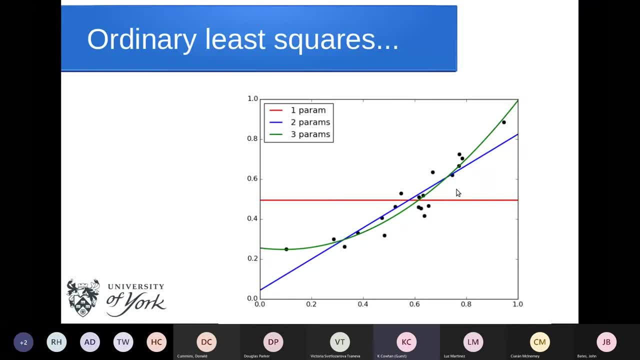 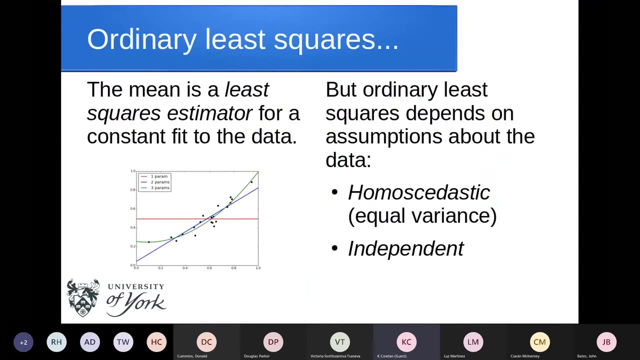 complex models. Here I've fitted a quadratic which has three parameters. I've also fitted a constant which has just one parameter. Now, fitting a constant by least squares is an uncommon thing to do, but it turns out to be mathematically identical to calculating the mean in the case of. 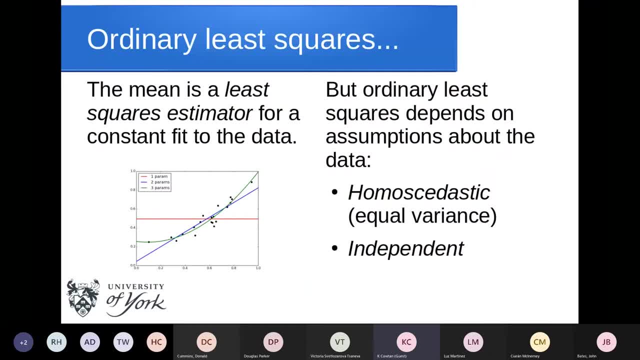 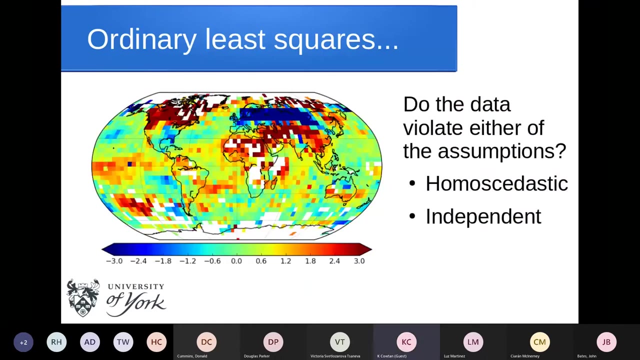 equal variance of the observations. The mean is a least squares estimator of a constant fit to the data, But ordinary least squares depends on assumptions about the data: Firstly, that the observations have equal variance And secondly, that they're independent. Now are these assumptions? 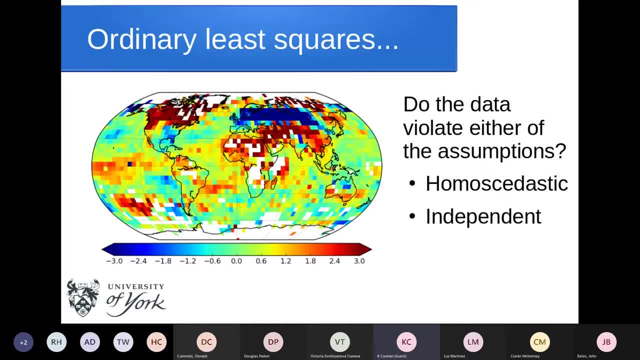 plausible in our case of averaging temperature data? I don't think so. I don't think so either. Now, I haven't mentioned these are temperature data anomalies. They're deviations from seasonal norms, So we've got a little bit of variation. But if we look at this month of data, then you 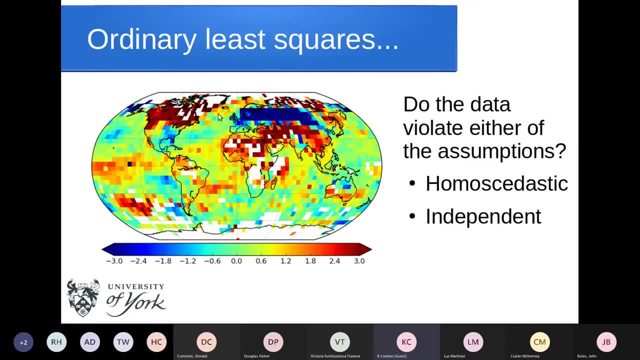 can see that there are regions of extended higher or lower temperatures, So it's clearly not complete independence, And we also see that land areas show a bit more variability. It's perhaps a bit noisier, So the assumption of equal variance is probably not very good either. 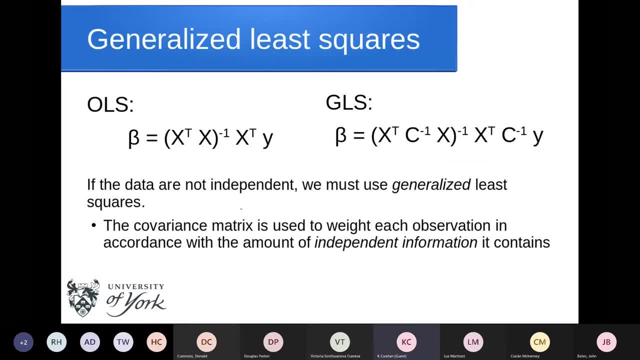 Okay, So how do we deal with this Now? you may remember from early statistics classes that there is an alternative and more complex approach, called generalized least squares, And the equations differ from ordinary least squares in that we insert a constant. And that's what we're going to do: We're going to insert a constant. 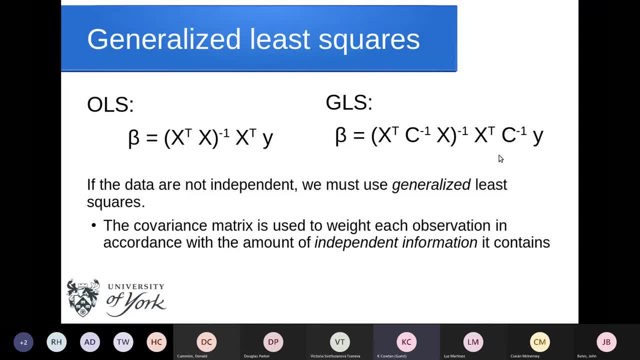 We're going to insert an additional matrix in the equation that we solve for the parameters of the model, And this is a covariance matrix. It tells us about the variability of each observation and how it co-varies with other observations. In other words, it contains implicitly: 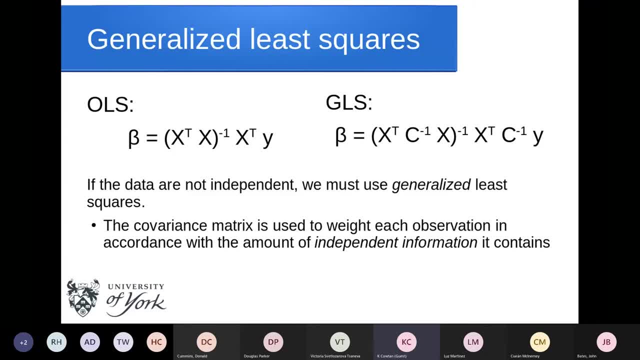 information about how much independent information each observation contains. So we've seen that we can use ordinary least squares to calculate a mean. It's a model with one parameter, But we can also use generalized least squares for the same problem in the case where the observations are not independent. So what happens when we do this? Well, 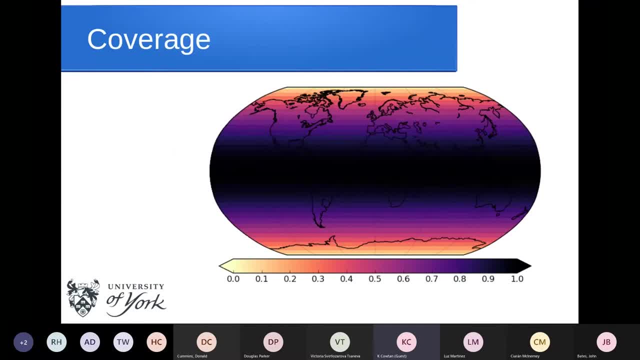 here's a very simple case. Suppose we have complete coverage of the planet. So here's our gridded data set with complete coverage And I've used generalized least squares to calculate the weight to be given to each grid box, each observation in our data set, just using the covariance matrix, where we have a very simple. 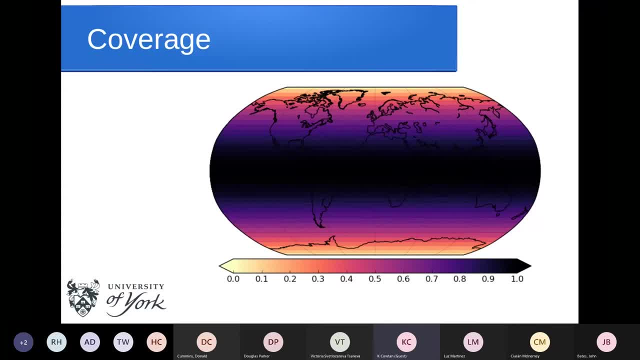 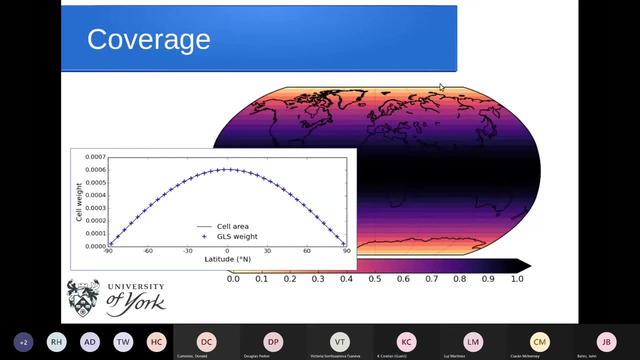 model of how covariance drops off with distance. And what happens is that generalized least squares decides for us that observations at the equator have to have a larger weight than observations at the pole. And if we plot how those weights vary, they show this cosine shape. What's happened? 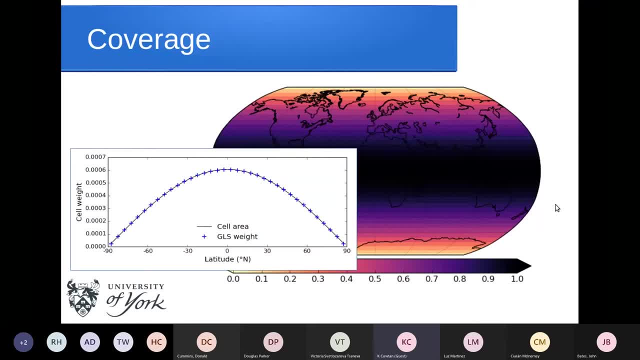 is that generalized least squares has deduced cosine weighting Area, weighting of the grid boxes, without being told explicitly anything about the grid box areas. It's just inferred that from how close the grid boxes are together, and therefore what the associated covariance is between those observations, would be So that's an interesting result. The 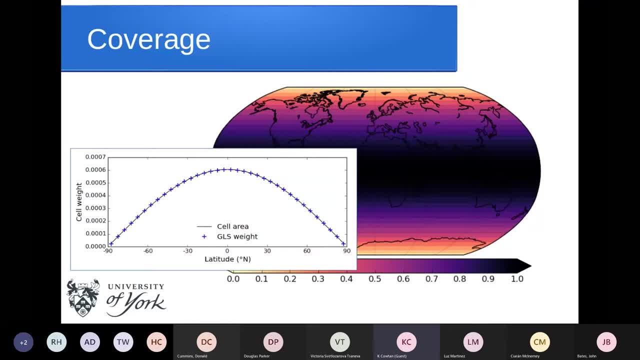 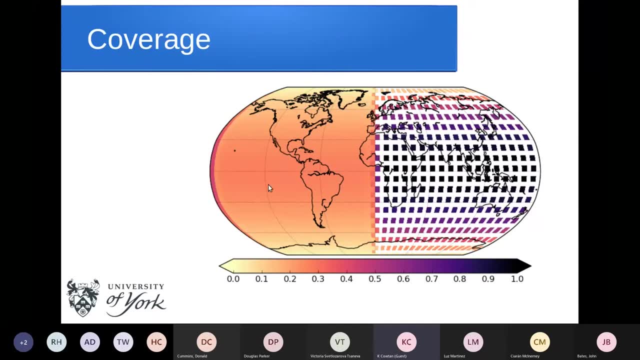 mathematics gives us something for free that we didn't put into it. Here's a more interesting case. So now I've got complete observational coverage of the Western Hemisphere, But in the Eastern Hemisphere I've only got a quarter of the number of observations. I've thrown away three points out. 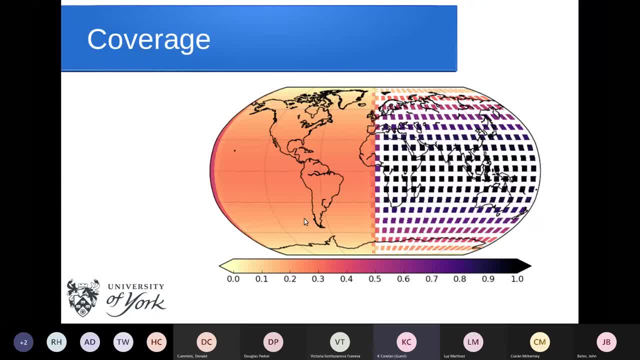 of every four And this shows the weights that's going to be given to each grid box in the data set, And you can see we still have the cosine weighting in the Western Hemisphere and also of observations in the Eastern Hemisphere, And so now I've got a quarter of the number of observations. 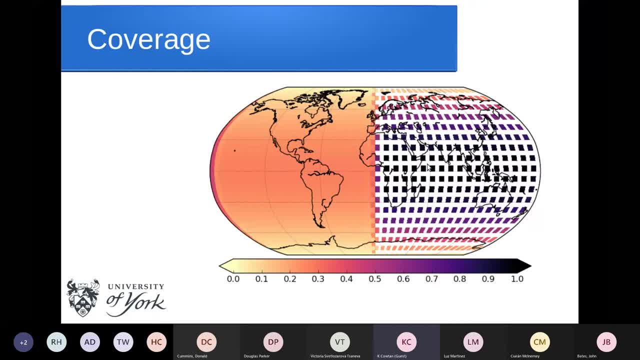 that's going to be given to each grid box in the Eastern Hemisphere, But they have been up weighted by about a factor of four. If we didn't do this, then I just calculated a simple area weighted average. then we'd get a temperature which was 80% the temperature of the Western Hemisphere and 20% the temperature of the Eastern Hemisphere. 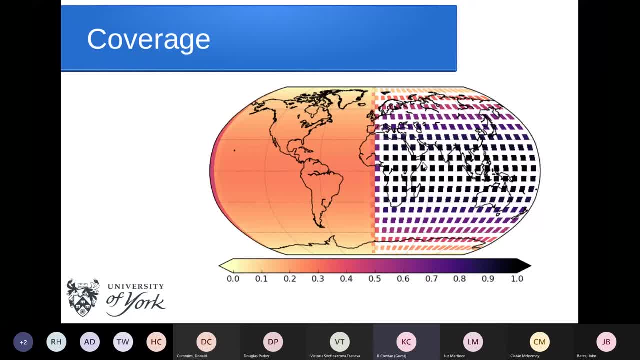 But by introducing the generalized least squares for determining the weights, we have got a grazing average which is equal to the Hemosphira's equal weight. So let's look at a more extreme case Now. suppose we have full coverage of the Western. 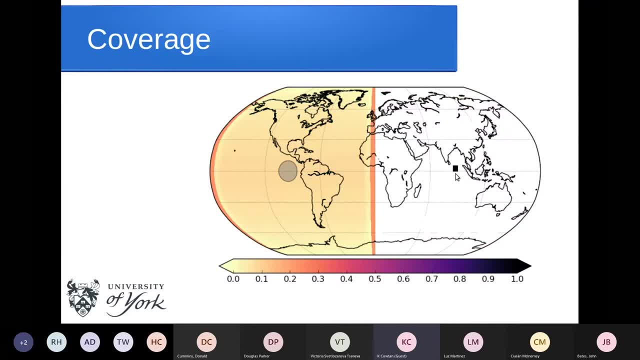 Hemisphere and just one isolated observation in the Eastern Hemisphere. Now again, this observation gets up weighted, but it's certainly not up weighted to the same value as the whole of the Western Hemisphere. In fact, if we calculate what area of observations would be required to give the same weight as this single observation in the Eastern Hemisphere, 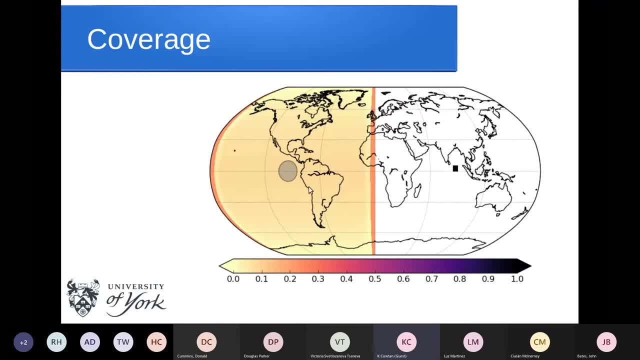 it's actually given by this circle here, which has a radius of about 1,000 kilometers, which is about the e-folding distance over which covariance drops off the area, the distant length over which temperatures are a good predictor for neighboring temperatures. 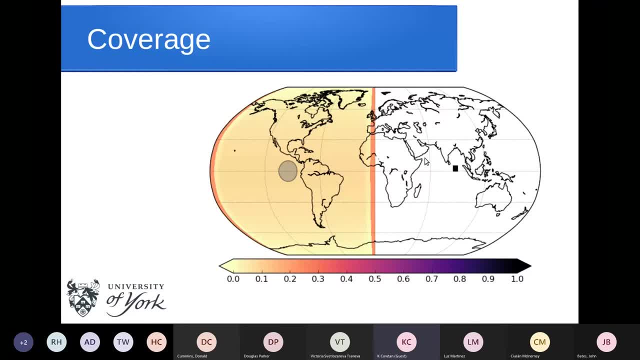 So that's another interesting result. This one observation can't tell us about an entire missing hemisphere of observations, but it can tell us about an area around it, and it has been up-weighted in accordance with the area about which it is actually informative. 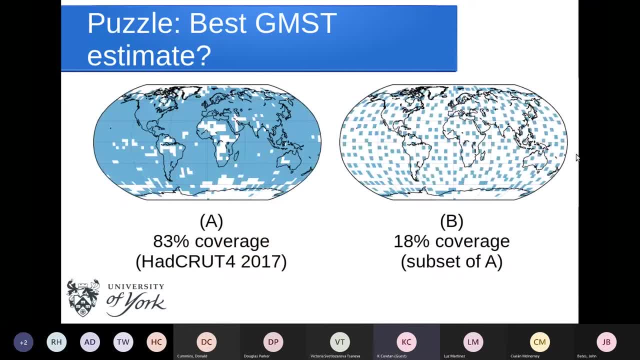 So okay, so that's lots of nice theoretical cases. That kind of brings us back to the puzzle I suggested at the beginning- and we're now really in a position to this: What would give us the best estimate of global mean surface temperature, the coverage on the left or the coverage on the right? 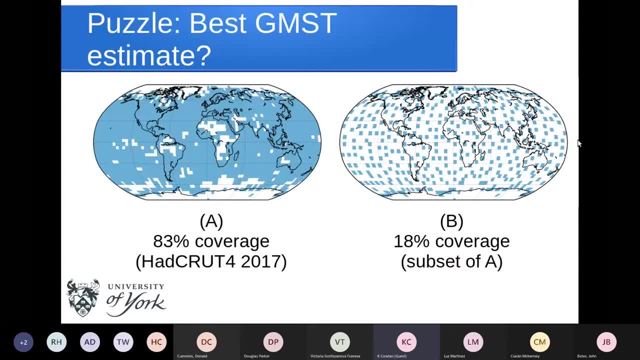 So to work this out, we can do some calculations, We can use simulated data- In this case it's going to be from a weather model which produces plausible temperature fields covering the whole planet, And what we're going to do is reduce the 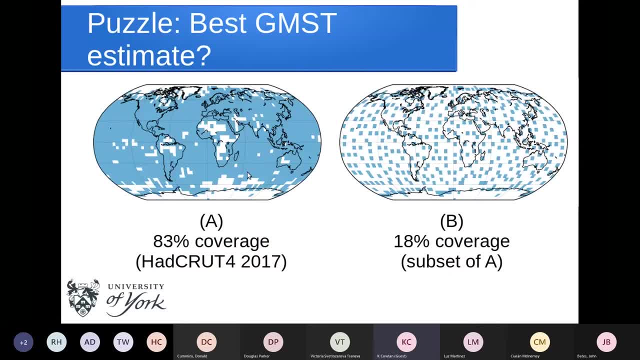 coverage to one of each of these cases and calculate both the true temperature for each month of data and what we would get from an area-weighted mean with reduced coverage. So what I'm going to do is determine the error in those estimates by doing lots of different. 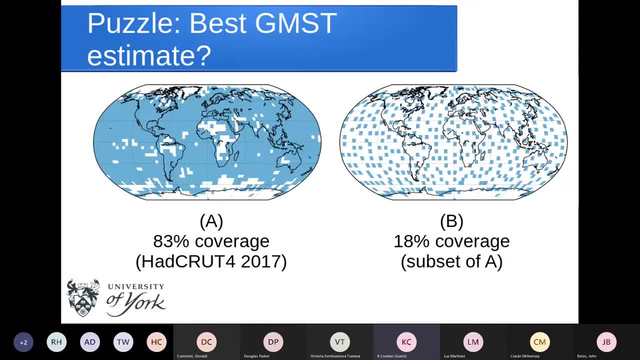 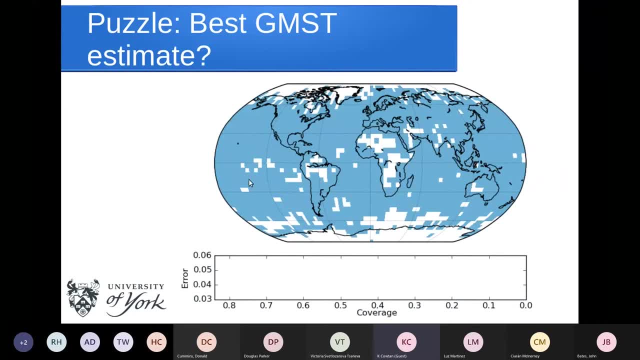 months and see how far off we are when we use limited coverage. So what I'm going to do is a little animation of doing this, and what I'm going to do is start with the HADCRA-T4 coverage, the 2017 coverage, and then I'm going to throw away grid cells, one at a time, always picking the. 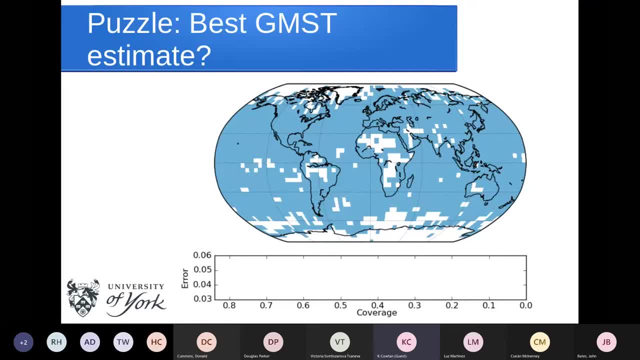 one which would receive the lowest weight in generalized least squares, the one which it says contains the least information. And we'll see what happens when we do that, And I'm going to plot error in the graph at the bottom and there'll be two lines. The lower line will be in the case. 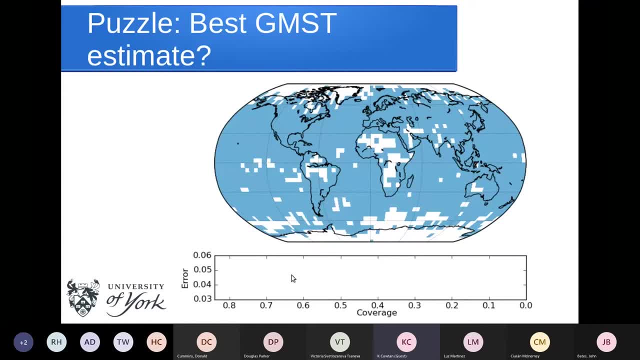 where the grid boxes contain zero error, where the temperature estimates in the grid boxes are perfect, and another line which will show the case where there are errors in the observation. So I'll start the animation now. So first, when we start throwing away grid boxes, nothing happens. 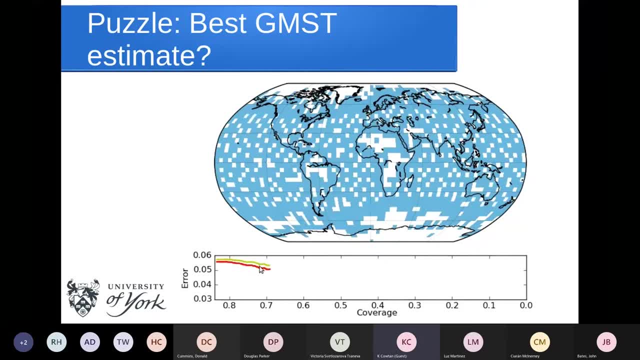 And then the error starts reducing, and we can see that with systematically throwing away observations in the regions which are most densely observed. we're not throwing away observations around the edges yet, And as we throw away more, then the errors actually go down. 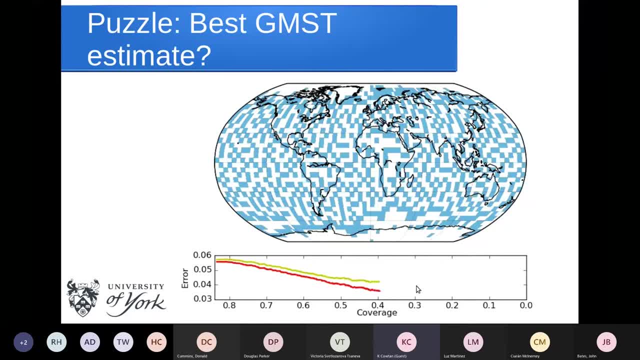 both in the edges and in the curves- The error-free case and in the case where we have errors in the observations. Eventually it reaches the point where the noise in the data begins to significantly impact the resulting mean. So the upper curve starts turning upwards And then gradually we reach the point. 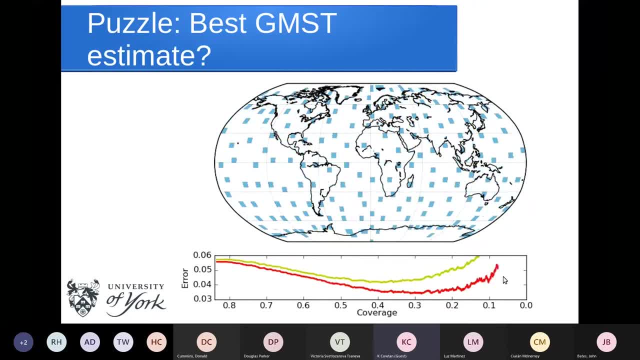 where the lower curve turns upwards, because we simply don't have enough observations to represent the whole surface of the planet anymore. So that's interesting And that allows us to answer the question I posed at the beginning, which was the best estimator of global mean surface temperature. 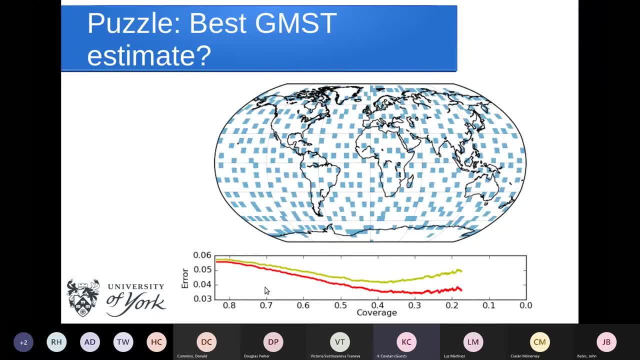 My original data set with 83% coverage or this one with 17% coverage, And you can see, both in the error-free case and the case with errors, the reduced coverage gives us the better answer Because in this case it is more representative, even though we have fewer observations. 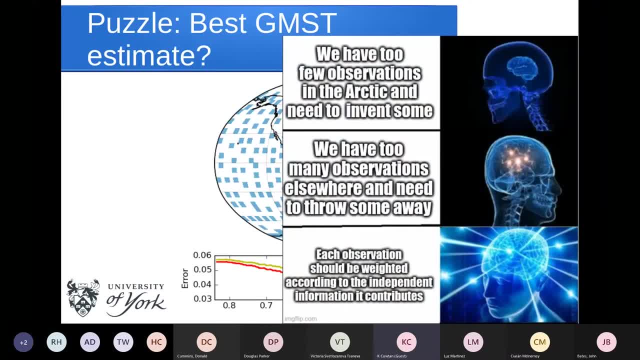 OK, so what's going on here? I think for me, one of the things that I do with a piece of mathematics is that I attach a narrative to it which helps me to think about the mathematics And that allows me to draw quick inferences about what a calculation might do or whether it might be useful, without actually having to do a simulation. 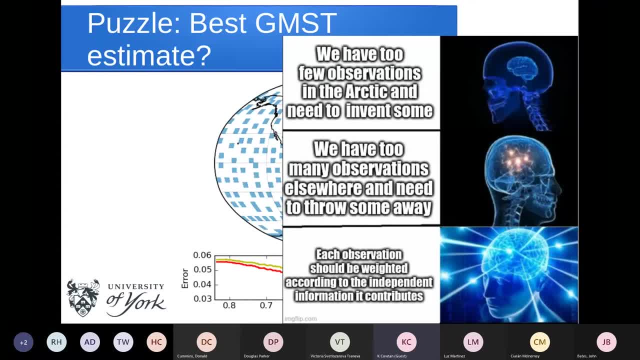 And that can be really helpful if the narrative I have attached to a piece of mathematics is appropriate for the particular problem. But it can be unhelpful if the narrative is incorrect, If it doesn't apply to the case. So here are three narratives that we might really apply to the concept of taking a global mean with incomplete coverage. 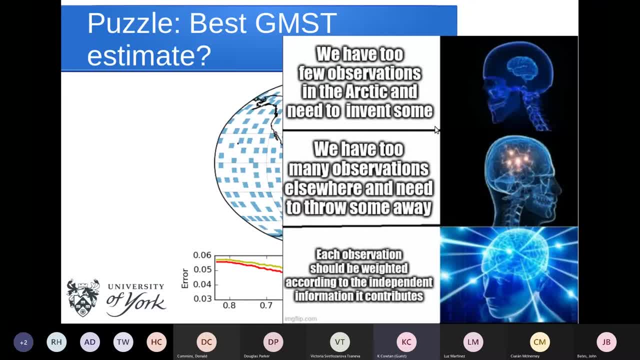 So if we interpret this as having too few observations in the Arctic and needing to invent some, then our other scientific intuition about inventing observations rebels against that And And we say, oh no, that that must be wrong. If we say we have too many observations elsewhere and need to throw some away, then perhaps that's in some ways a better framing. 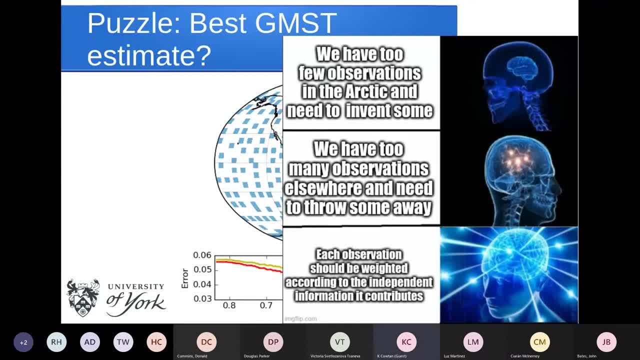 It does bring in the concept of having a more representative sample of the population, But in this case, had we started with a narrative saying each observation should be weighted According to the independent information it contributes, then I think we would have ended up with with a better intuition as to how to to calculate a mean in this case. 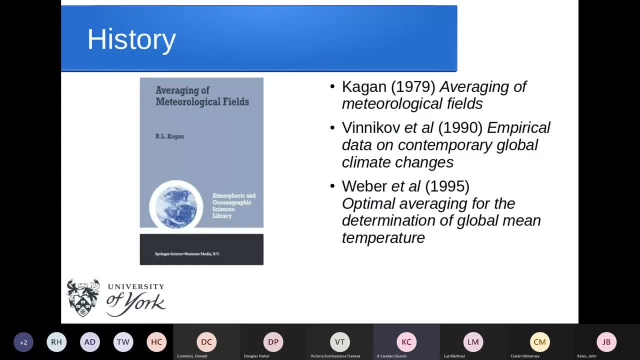 Now, none of this is new or clever. This was already published in a much more sophisticated analysis by Rufim Kagan In Moscow in 1979, he published this book in Russian, which was eventually translated. One of his colleagues, Finnikov, then moved to America and some of the work was was continued at NOAA but didn't was not sufficiently influential to be widely adopted in the IPCC report, although it received some attention. 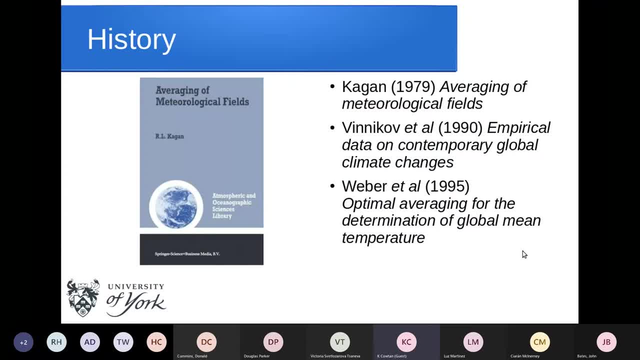 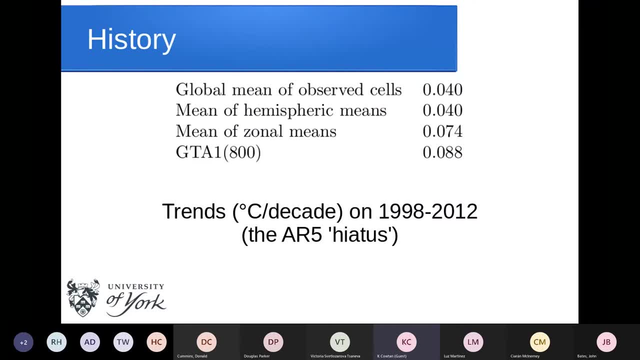 But hopefully now This is is being more widely recognized. Now, what difference does it make? just to show that it does make a significant difference, We had this number reported in the IPCC assessment report of of four hundredths of a Celsius per decade. 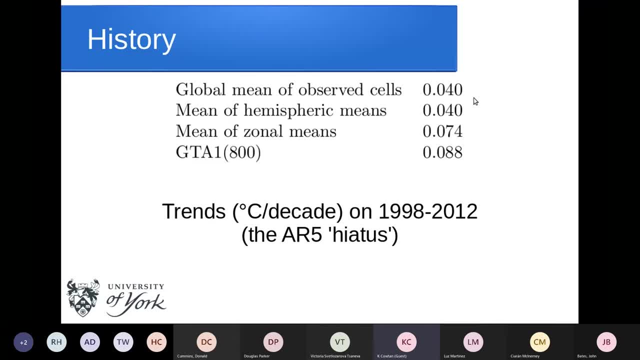 And and that there are a few crude methods which have been used to to to try and address the coverage problem. If I use this, This generalize the least squares approach, then we end up with a figure which is is more than double that, and that that's a significant difference in in the trend. 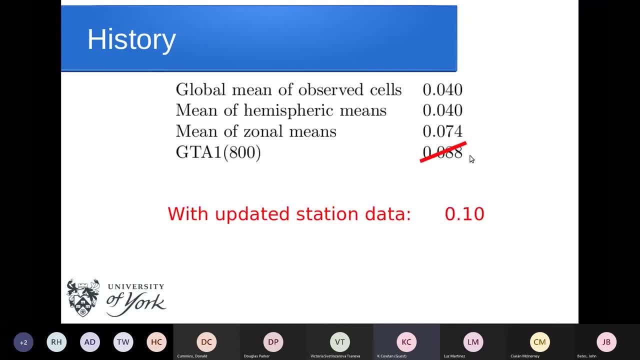 There are other factors as well. So, for example, this: the data on which this trend calculation was based included some stations which were present for the first half of the hiatus period But missing for the second By half, And, and, and. that's what created an additional data bias, including those made a difference. 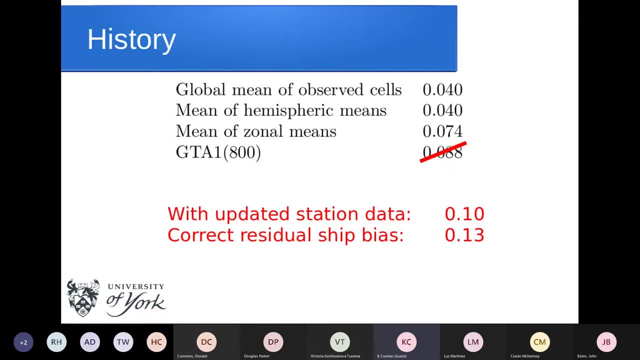 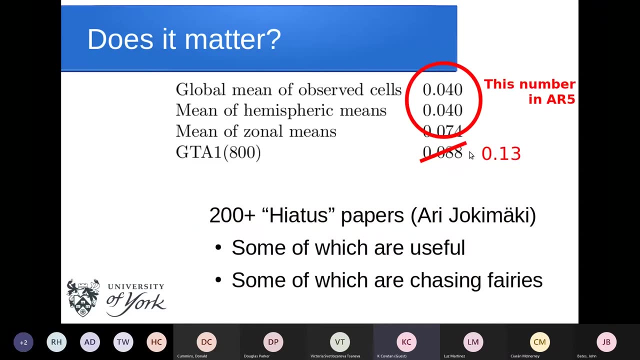 And there was also a a change in the way temperatures we may measured in the shipping fleets, So the seas surface temperatures also contained a bias which influenced the result. So we end up with with a number which is very different. I think current consensus would be much closer to a number like this, based on modern, modern data sets. 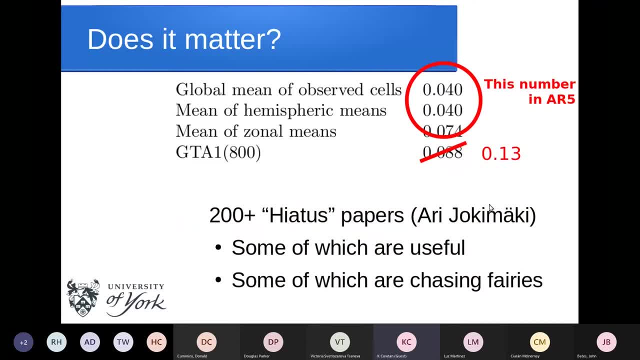 Which is very different from others. Great, thank you the number that was in the original report. Nonetheless, there have been at least 200 papers. I think our catalogue's up to about 300 now. This was a piece of literature review done. 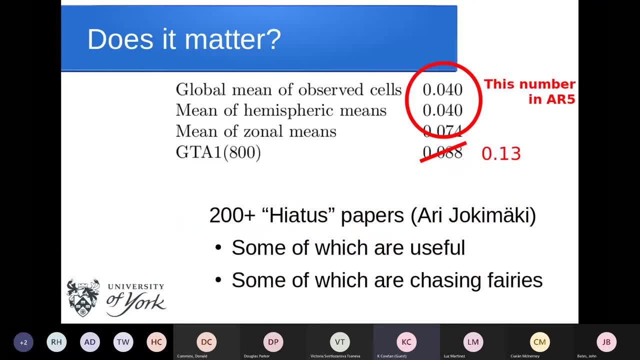 by a colleague, Ari Yoki Maki, Two or 300 papers studying this phenomena, which in large part arose from problems in the data. There were some useful things which came out of that, but many of them were really barking up the wrong tree. 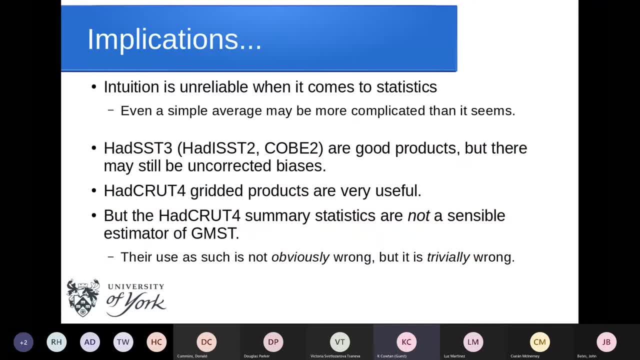 Okay, what are the implications? Intuition is unreliable when it comes to statistics. Even a simple average may be more complicated than it seems. Because this was for a climate audience, I was introduced some commentary on the data products. I work with the Met Office team. 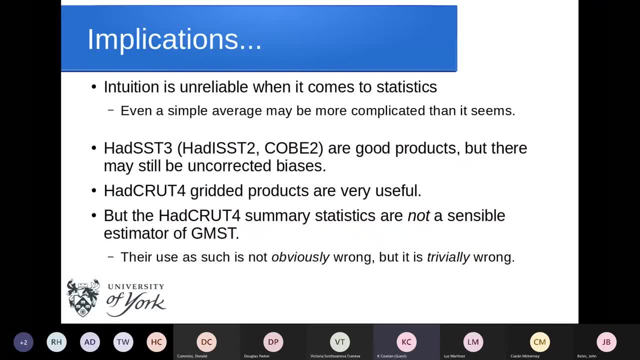 and I'm working on the next generation data set And there are places where their data and their data analysis are world leading. But using simple summary statistics on those data sets can certainly be misleading And I'm suggesting that the simple area may not be obviously wrong. 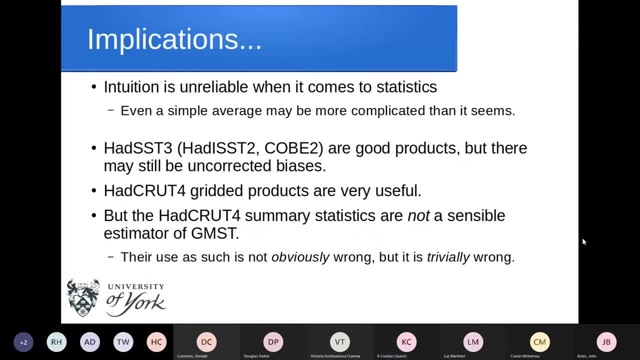 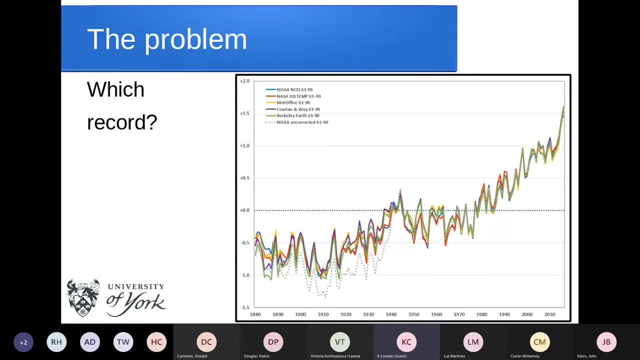 but it is trivially wrong in this case. One other thing which maybe is worth introducing, although it's not directly connected with what I've been talking about, is the fact that we have many different versions of the temperature record from a different provider. 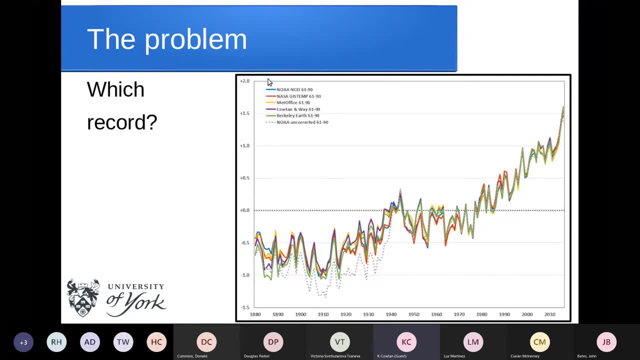 Two US government agencies, the UK Met Office- there's one which I produce and there's this one from Berkeley Earth- And it's interesting to ask why people pick one record over the other. How good is their criteria for deciding which data set can answer their research question? 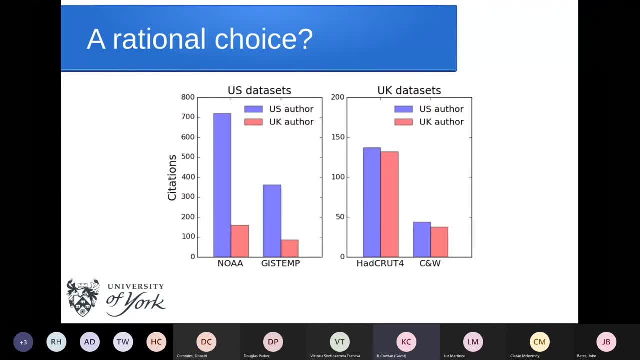 Well, I did a little survey of which data sets different authors use And, interestingly, if you compare US authors and UK authors, US authors are proportionally much more likely to use a US data set and UK authors are proportionally a lot more likely to use a UK data set. And there may be 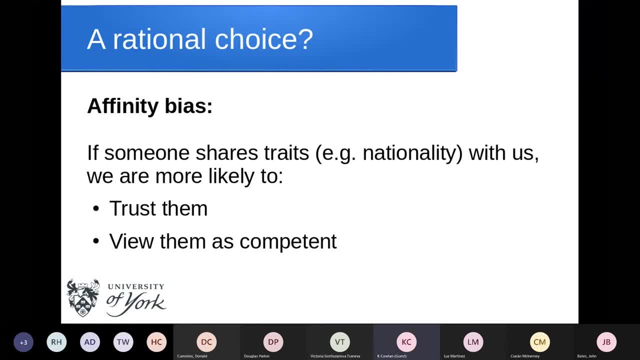 in some cases, rational reasons for this, for example, access to expertise, But it would also be surprising if there weren't an element of affinity bias. So if someone shares traits with us, we're more likely to trust them and view them as competent. So I think that this plays a role. 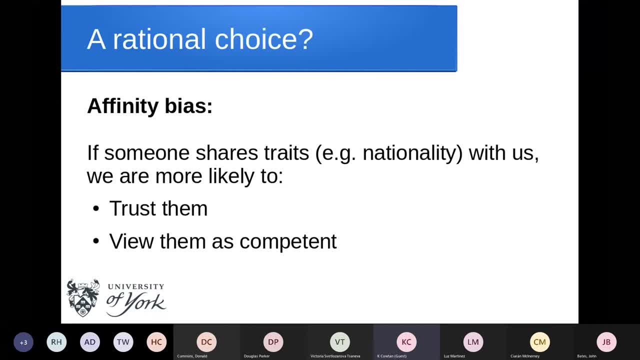 And the reason I need to look for this is that I've seen exactly the same thing in people choosing which software to use in X-ray crystallography, So I think we can't neglect these social factors when understanding why people use data. Okay, so that's really an unsolved problem. 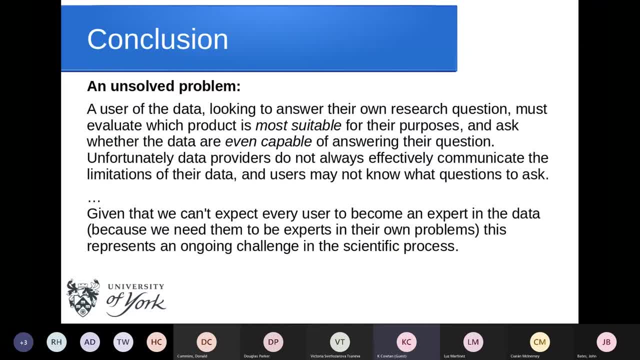 A user of data looking to answer their own research question has to evaluate different data products and ask whether the data are capable of answering their research question. And as data providers, we don't always effectively communicate the limitations of our data and users may not ask what questions to ask And we can't expect every user to become an expert in. 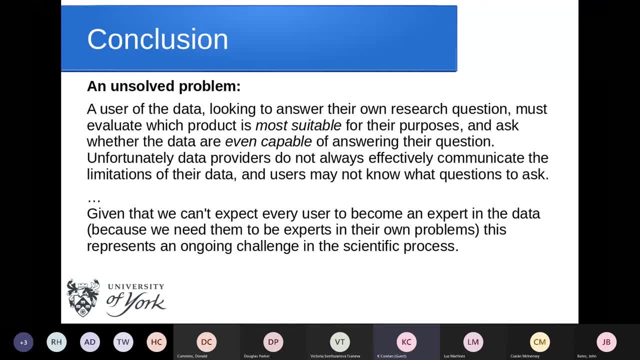 the data because they need to be experts in their own problems. All of us only have so much head space, So this is an ongoing challenge in the scientific process. It's a challenge in crystallography and it's a challenge in climate science and, I imagine, in statistics as well. 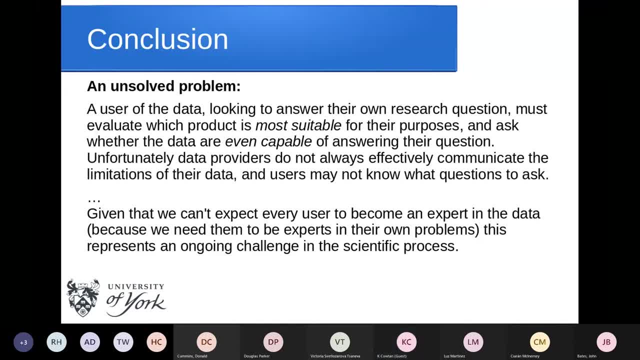 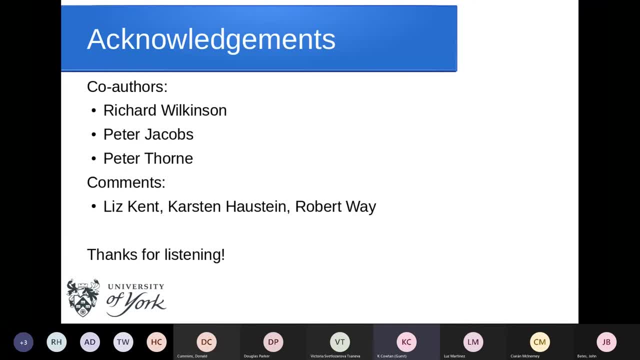 And I don't have a solution to that one. Okay, so that's all I wanted to talk about. The co-authors on the statistical paper on this were Richard Wilkinson, Peter Jacobs and Peter Thorne, And I also have very useful comments from Liz Kent, Karsten Haastein. 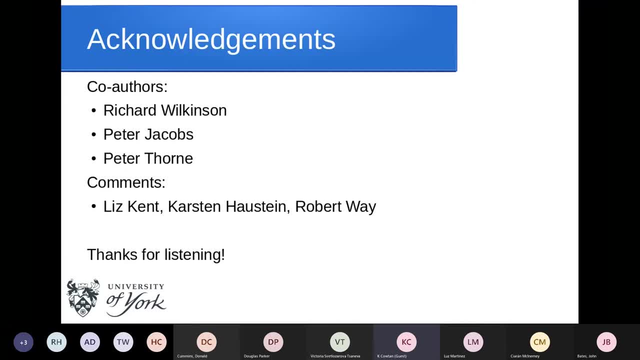 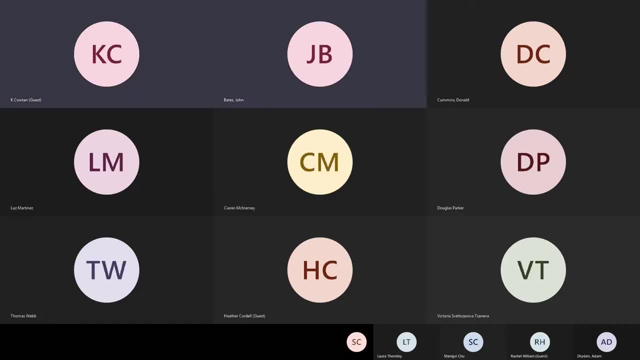 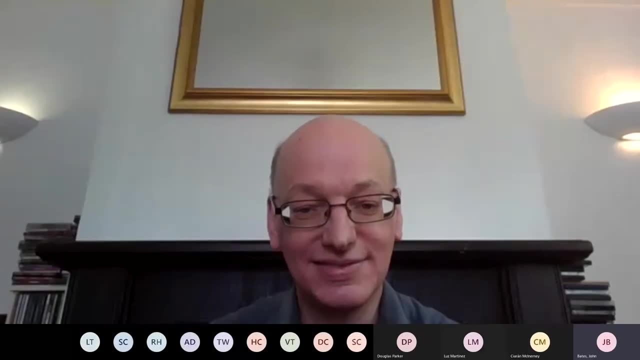 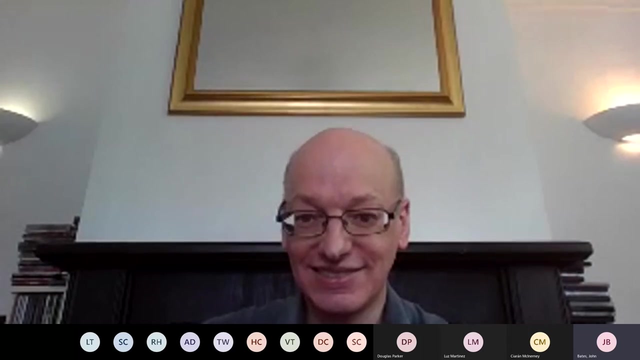 and Robert Way, And thank you everyone for listening and for inviting me. Brilliant, Thank you very much. Thank you, Kevin. Someone else already worked out how to do the sort of an instant applause icon, which is great. I'll just sort of pause to invite others to enter any comments in the chat. 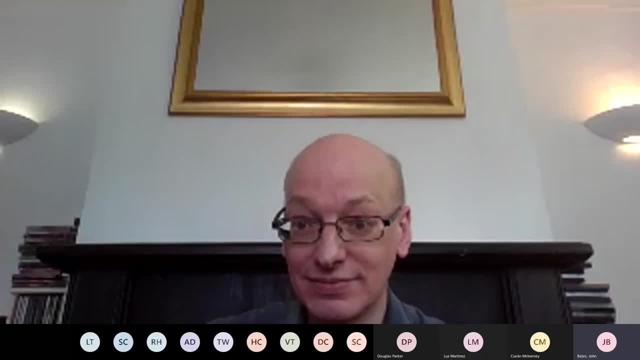 bar on the right-hand side if they have any questions or comments. One thing that struck me right at the beginning of your talk: that you presented data in a different way than the one that we've had so far, And I think you were suggesting that actually the increased 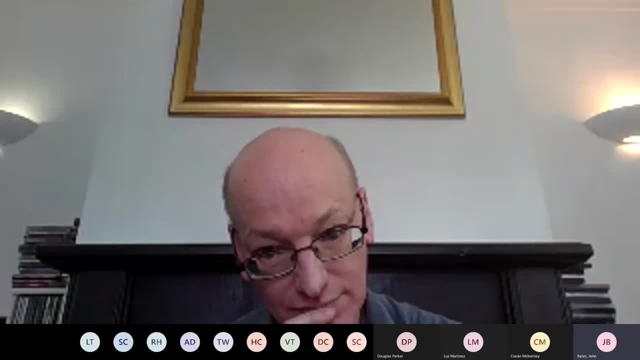 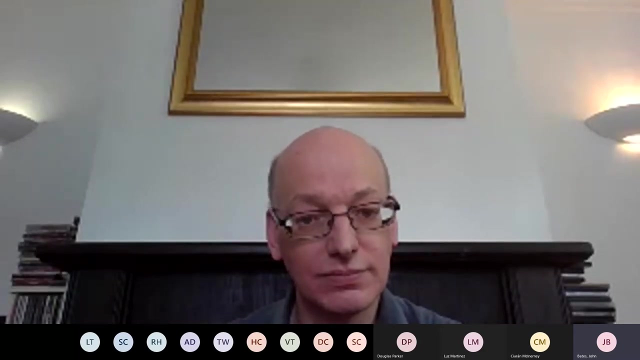 temperature might have been higher in that period than was generally thought. But it was the climate data experts that were challenging you, rather than the naysayers and the sceptics, And were you surprised by that? So I initially got involved in the problem because of you know. 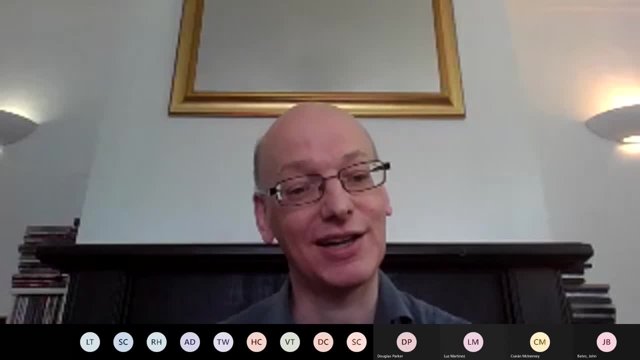 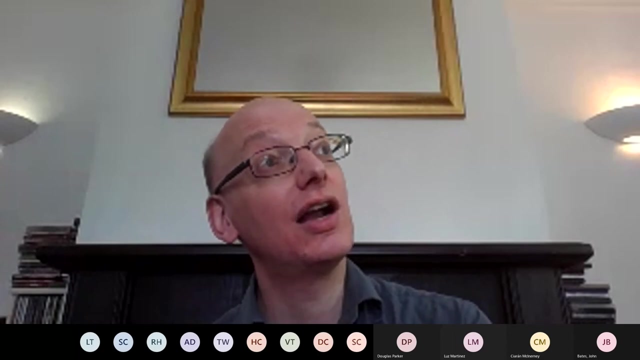 um, uh uh, science denial, um, uh, trying to address the issues there, um, but um, the resistance from within the community was, uh, it was, in some respects, surprising and in some respects, not surprising. so, um, people in the climate science community had been very badly burned from their initially. 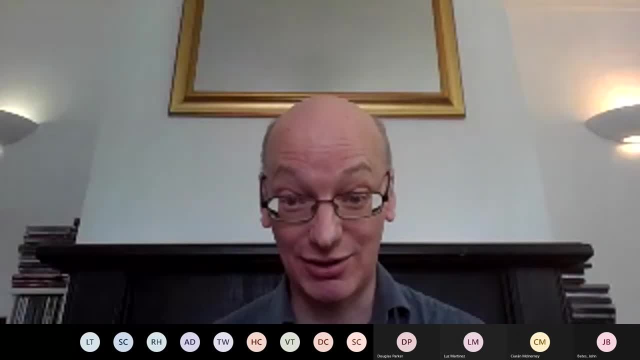 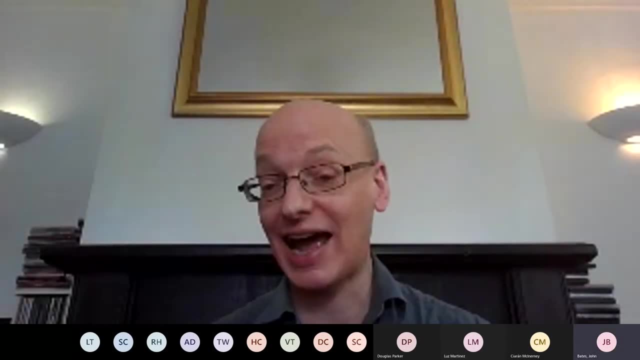 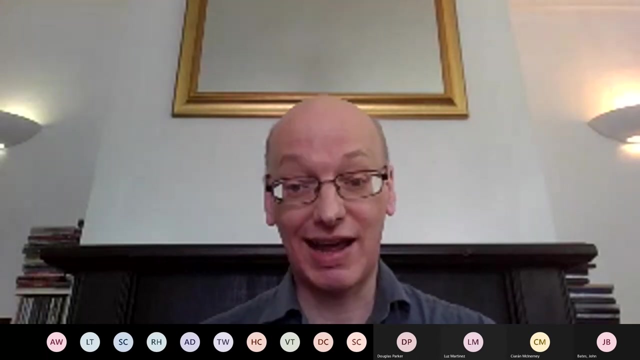 initial attempts to engage with, with climate science, with, well, with science deniers in general. um so, uh, and as a result, i, i think a reaction to that had, uh, become very, very conservative in in their interpretations. um so, so i, i, i think that that that has impacted people particularly in this country. um, 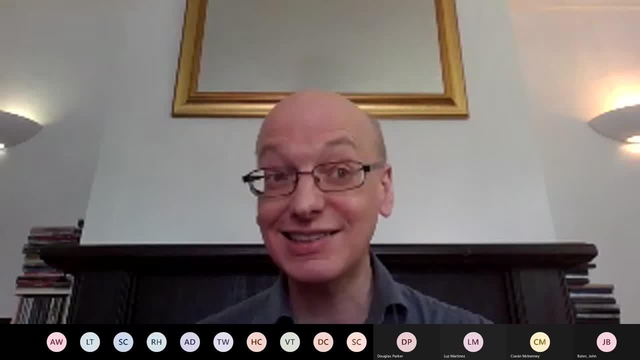 and in america, um, so in that sense i am not particularly surprised. yeah, great, yeah, and then make it make sense, yeah, i think, yeah, people want to be very, very sure of their grand. i i guess making making that case um, um, i think i welcome any questions from um and anyone else. there's one sort of technical thing. 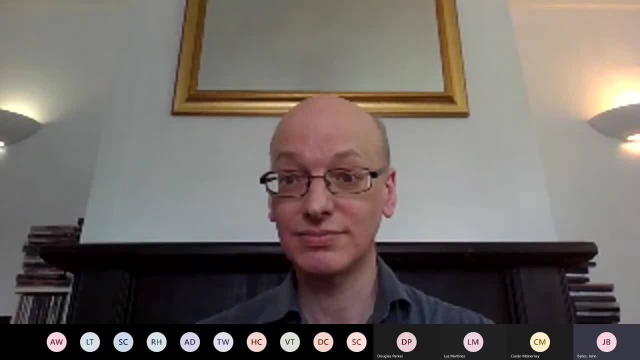 that, and i'm not not sure if i'm just maybe starting out from a depth on the technical bits of this. so so my understanding is you talked about sort of estimating the average temperature at a point in time and that obviously has knock on consequences for the, the, the trend um. 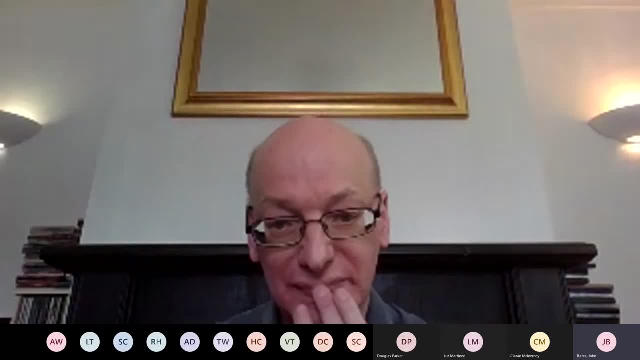 i just wonder whether are there any systematic reasons why, if there's an error in measuring the average temperature, that that error would vary over time and and then feed into the you know and give you a different answer for the trend to turn something sense as a question. uh, oh, there are. 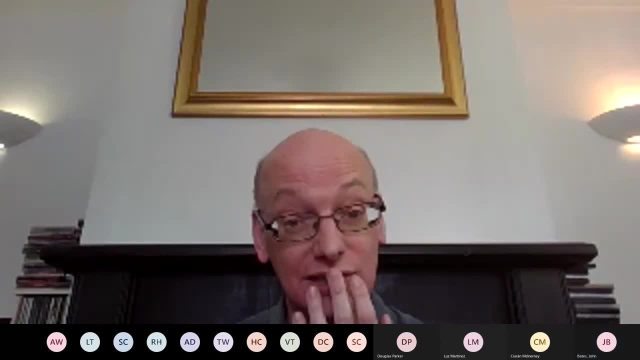 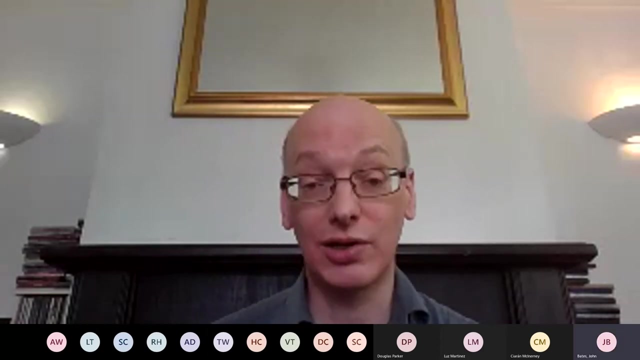 there are lots of systematic errors. the the biggest ones are in ceaseless temperatures, so transitions in observation types from buckets to engine room, intakes, um, and, and also variation in in location of weather stations and and how they're screened. so there are lots of systematic biases, uh, all of which need to be handled, and and the whole process is very, very 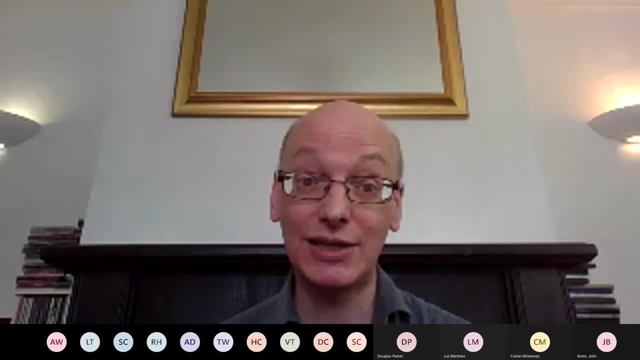 complex uh, but given that most of these observations were made for meteorology purposes and no one had any idea that they would be uh trying to um answer climate questions with these uh observations, um so uh, and- and some of them are still not understood- the the change in readings from ships. 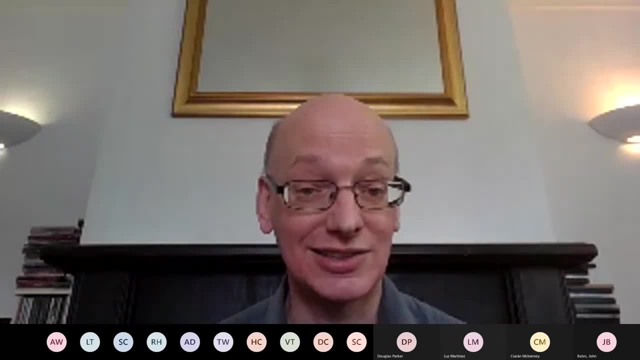 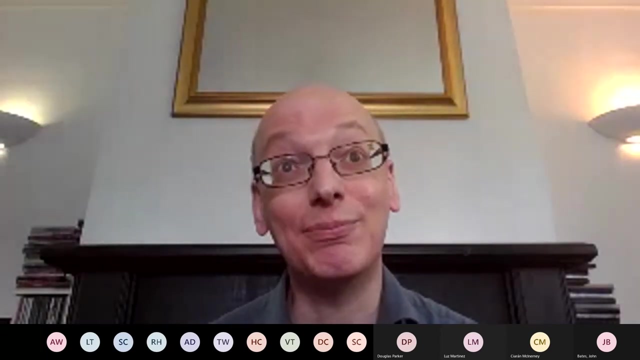 are running from about 2008. uh, last time i i looked at that problem, it wasn't understood. we published a paper showing that it was there, but but we don't really know where it comes from. um, so, um, uh, does that answer your question or are we going somewhere else with it? 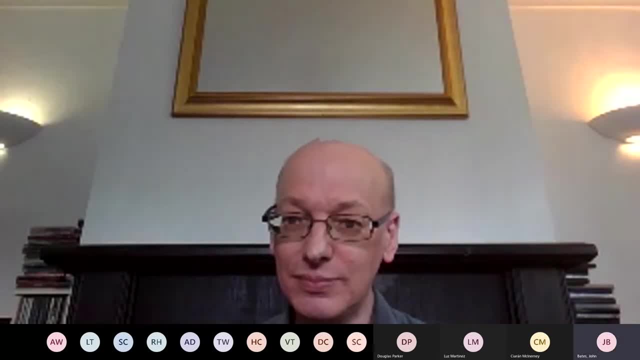 no, no, i think i think it does. yeah, yeah, yeah, that's, that's very, really helpful if there's a, it's um, there's 좀 from douglas about uh comment on the use of numerical model analysis in this kind of global mean. so, uh, yes, we, we have. 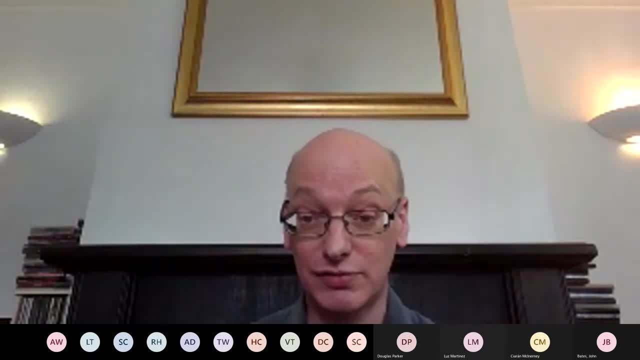 the simple observational data sets, uh, which are what i've been talking about, and, um, there are also call these data sets called weather model reanalyses, where you drive a weather model with either all the observations. you have much more diverse ranges of observations that we use in the 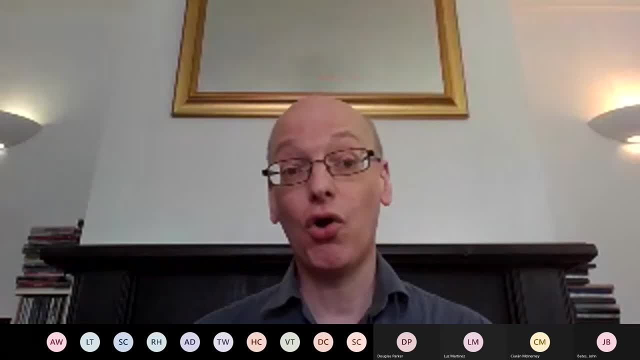 products I've been talking about, including satellite data- or from more limited ranges of data, types of data where you're aiming for uniformity. So there are some data reanalyses which just work from pressure data- pressure and wind rather- So we make lots of use of them. but I think there's a kind of social convention that the historical records are the longest and therefore are most trusted. Whether that's a valid perception is for me an open question. I'm not sure that the simple observation records are better than the reanalyses records. 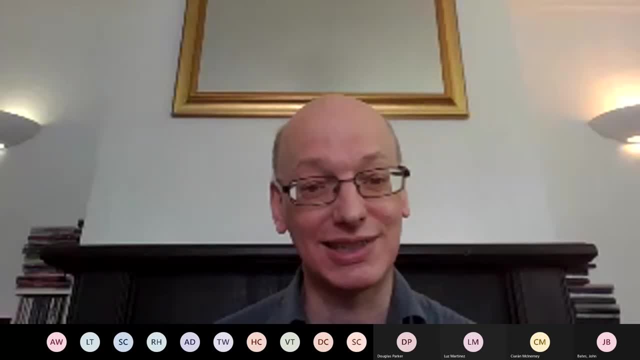 but they have different problems. People prefer simple data sets over complex ones, so that might be the explanation for why that's the case. But yes, I make a great deal of use of reanalysis data, but it is less useful in the communications context. 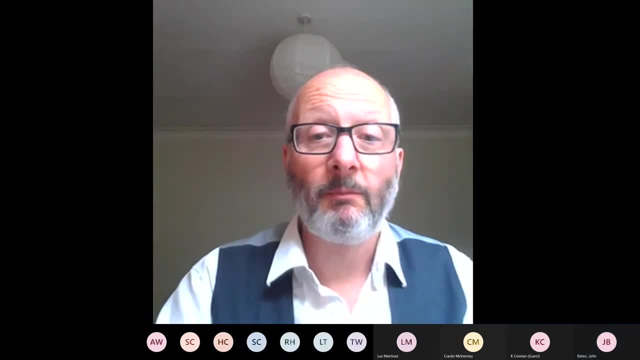 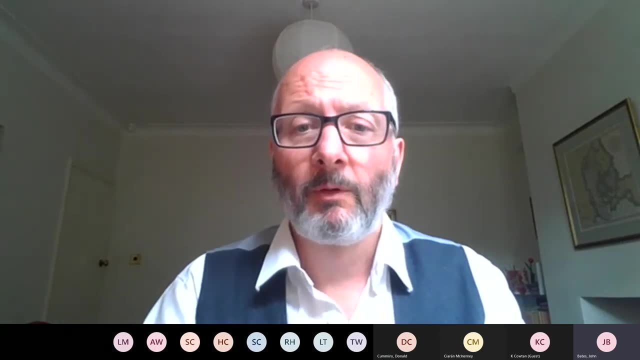 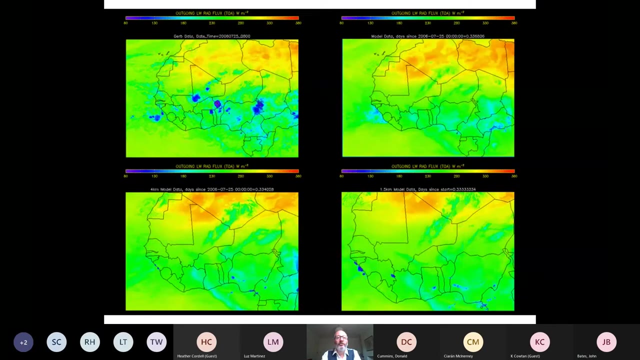 Can I hand over to you Professor Douglas Parker, who will talk to us about analysing and predicting African rainfall. Okay, thank you, John. I thought I would just start with this animation of clouds over Africa. So the top left panel here is observations and the others are models. So the observations. 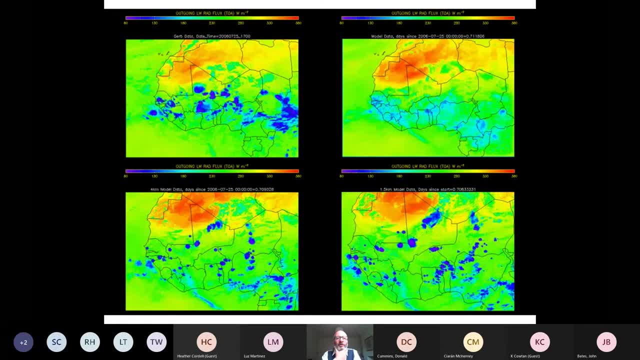 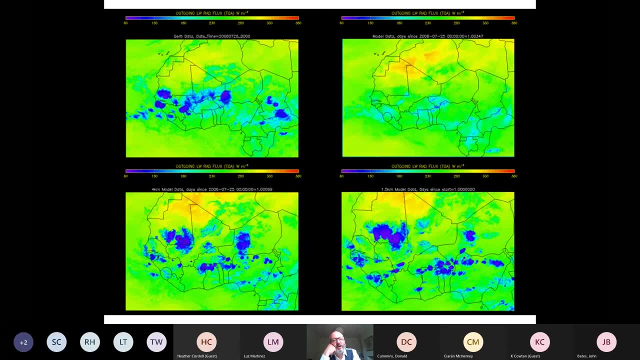 at the top left are satellite temperature measurements and they're coloured so that blue is cold. So the blue are the very, very, and the blue and the purple are very cold thunderstorms. I'm talking about African rainfall, but I'll focus on West Africa, which is 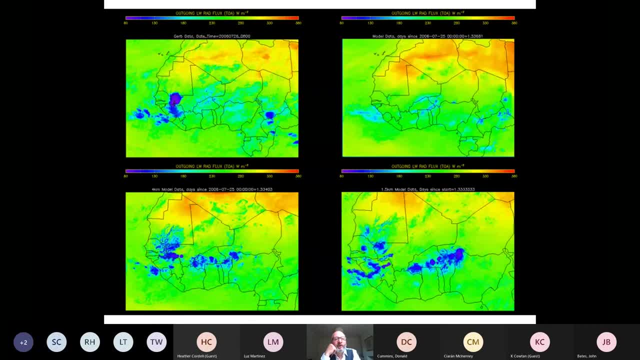 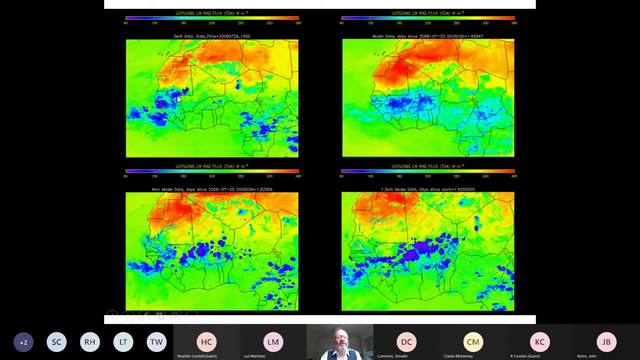 where we've done a lot of work. So you can see a few characteristics of these storms. Firstly, they are: if you know the geography of Africa, some of these are really big. If you see that one that's now decaying over the West, that whole envelope is thousands of kilometres across. 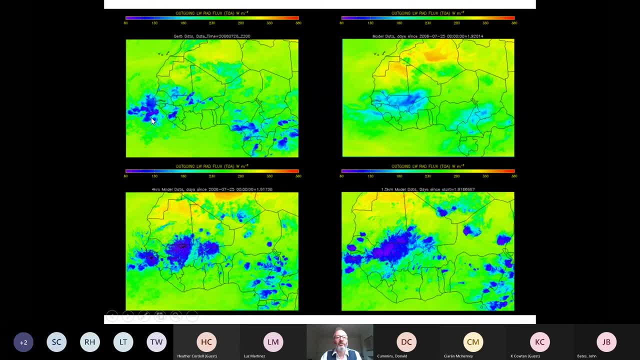 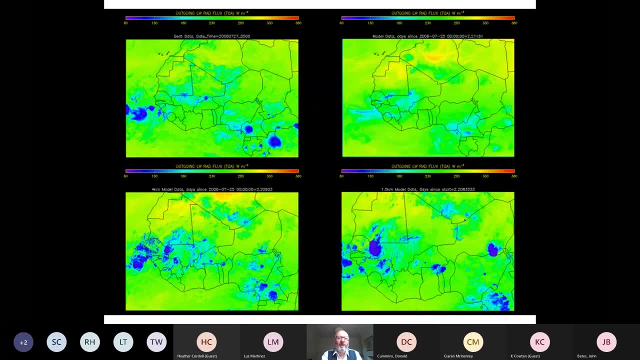 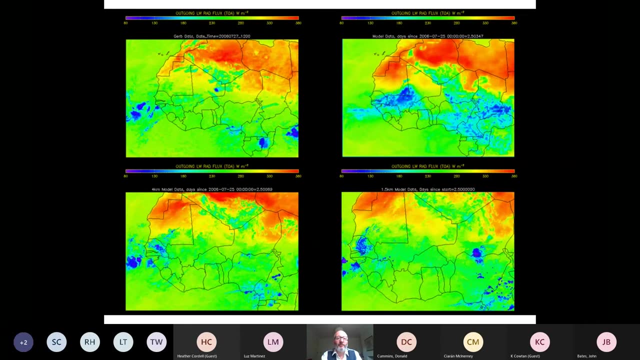 and they're really intense systems. They're going off the West Coast. That system is really intense When it gets really purple and very cold tops. that's a really intense thunderstorm, probably 15 kilometres high In altitude and very active, very heavy rain, a lot of lightning, intense winds at the surface. 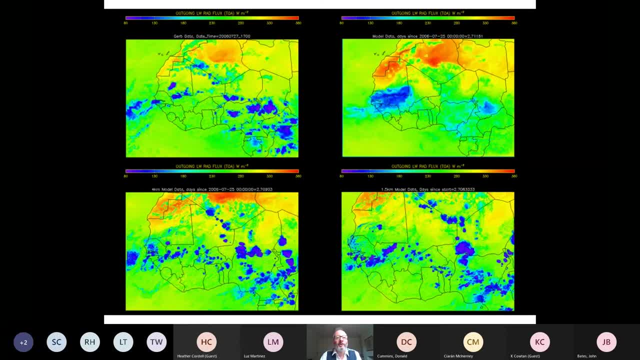 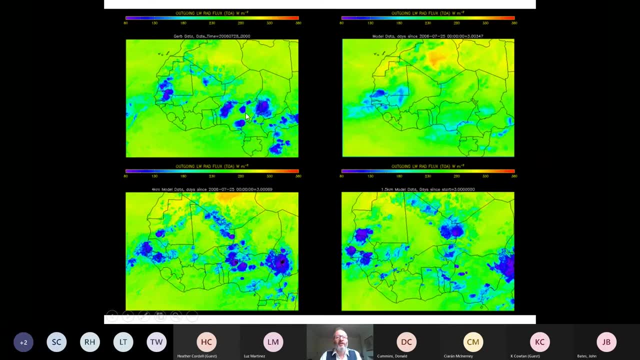 You see a strong daily cycle here. So this is about three in the afternoon when lots of little storms pop up in the afternoon. You can see a lot of organisation, So you can see they organise into lines And as you go into the night the time is just in the top index, if you can read that. 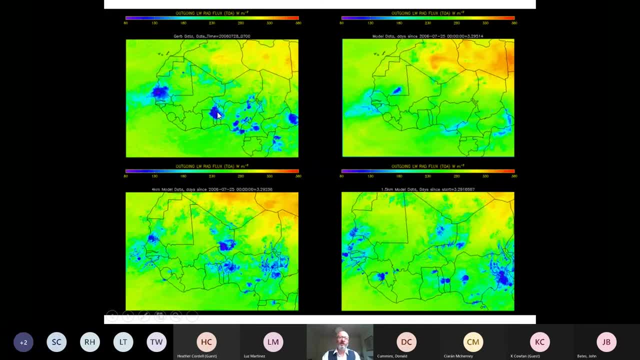 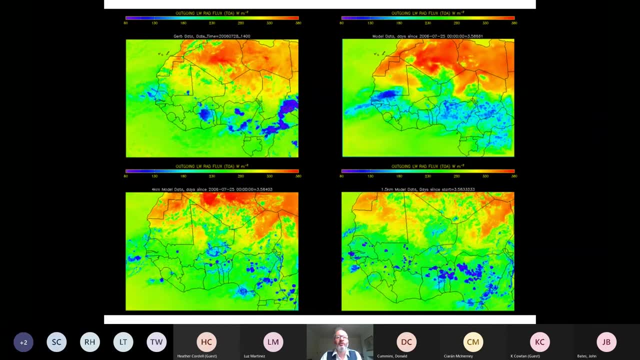 but it's just three in the morning, So overnight then you're left with just big, big storms moving around on their own big organised systems, Whereas when you can see you're coming to the next afternoon- so 11,, 12 o'clock, 13 and 15, they usually go bang. So here, 1500,. 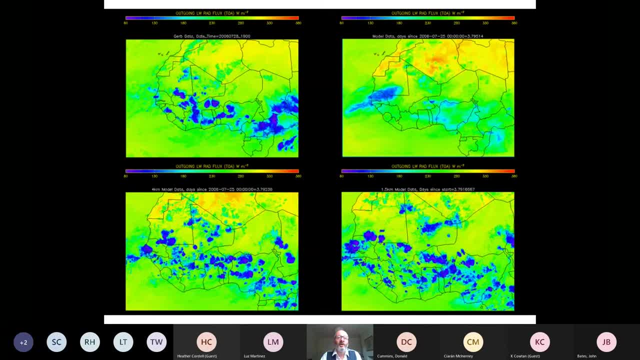 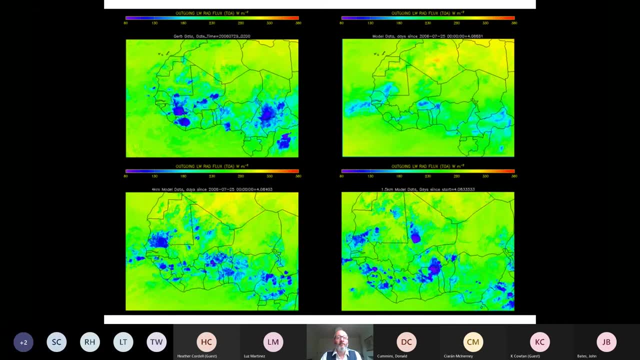 they're starting to appear again And again. they're organised in lines And then, as you go into the evening and night, they cluster into big, big systems. So this is just to give you a feel. I'll jump out of this now. We could watch this for the whole half an hour if you wanted. 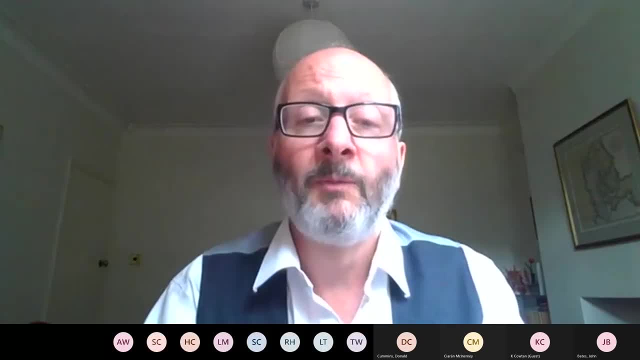 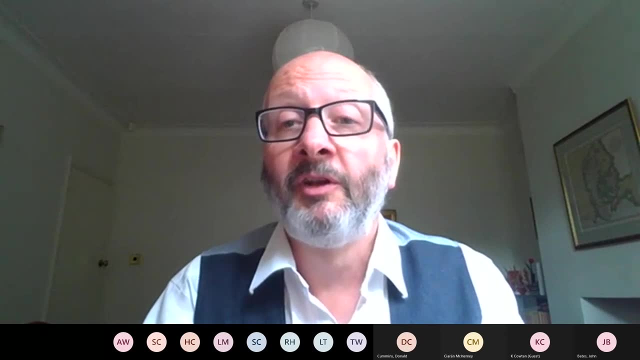 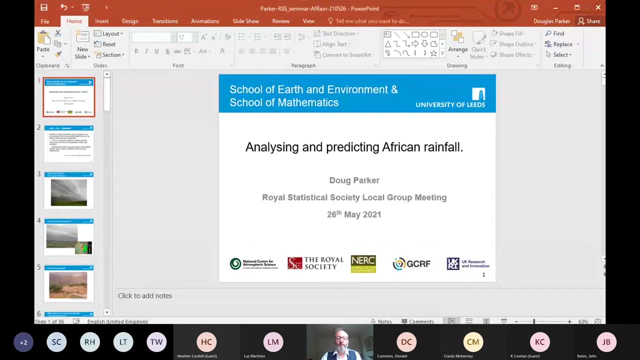 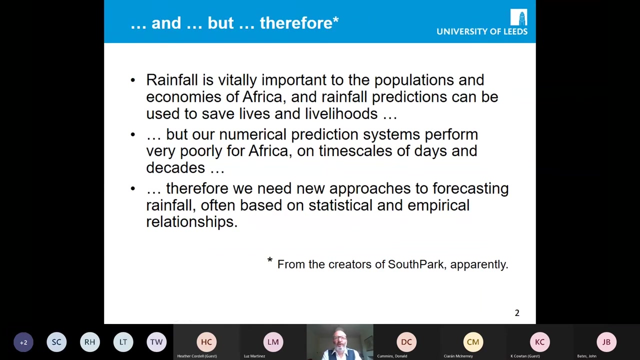 but that was just, as I say, to give you a feel for what rainfall looks like from space In this part of the world, And I'll go into the presentation now if I can find it. So I discovered this concept actually this week. I think it's kind of hokum, but this and 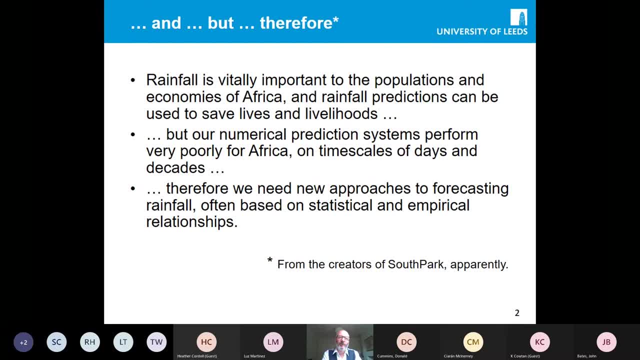 but therefore ABT approach. I think it's kind of hokum, because I think we already knew this, everybody knew this already, but it's kind of sounds to be popular jargon at the moment, So I thought I'd try it out. So the idea is, if you're telling a story, then you have to have 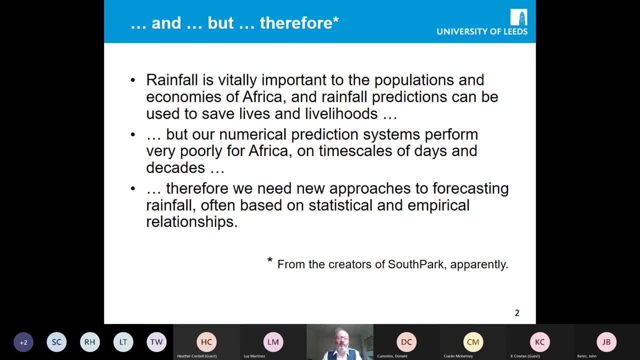 this ABT. So you have to have an and which is all the facts. So rainfall is vitally important for the populations and economies of Africa. So I think you can all understand that. Everybody can understand that rainfall can be very intense in Africa, but equally they're very dry regions. 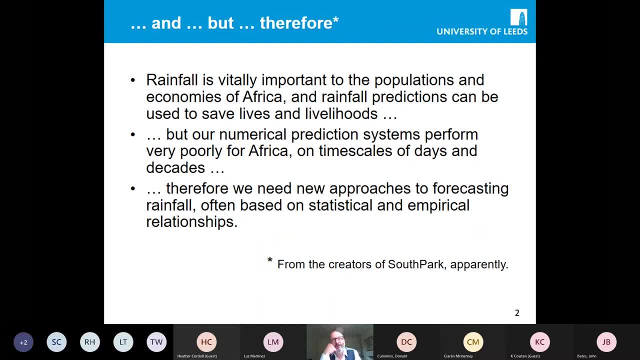 that depend critically on the rain. A lot of people in Africa are dependent on agriculture, So there's a lot of subsistence farming and the economies are sensitive to rainfall in many ways, And if you can predict rainfall, then you can save lives from you know, from natural disasters. 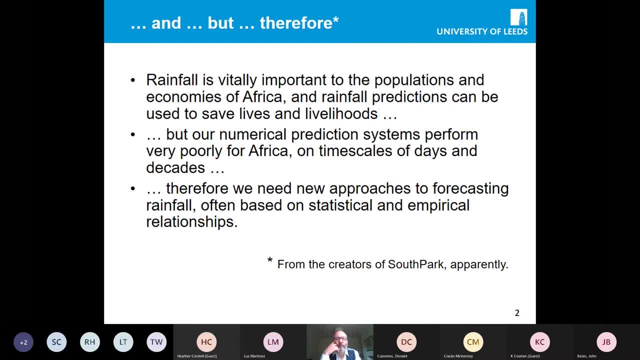 both for drought and for floods and intense storms, and protect livelihoods. you know, people lose their, their crops if there's drought or if there's flooding. they can lose their animals, they can lose their lives, of course. So good predictions can enable people to 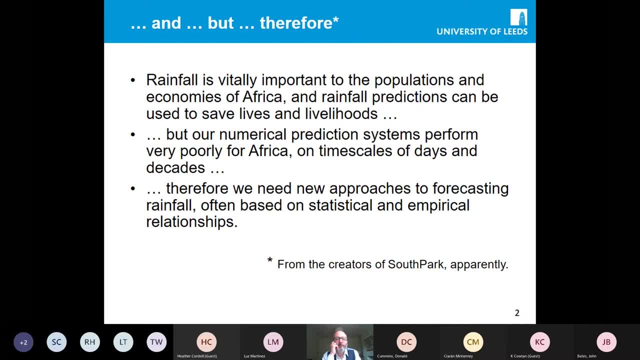 respond and live more comfortably. So the but is that our predictive systems, our models, both for climate and for weather, on short timescales, even on timescale of the day, are very poor, And I'll show you some evidence of that. And and the, therefore, is that we need to do things better. 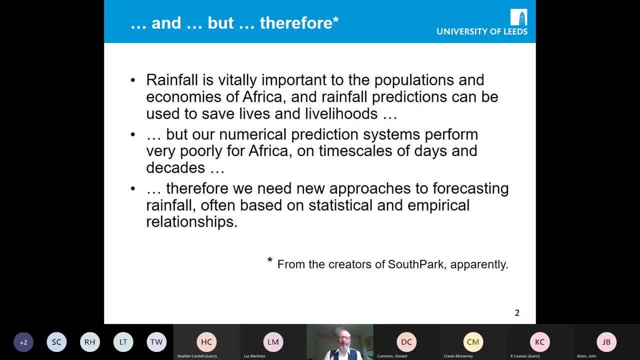 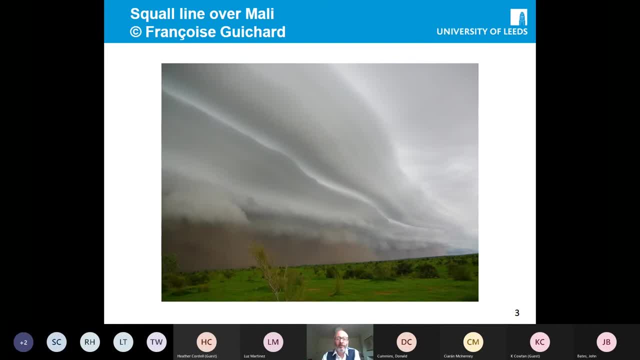 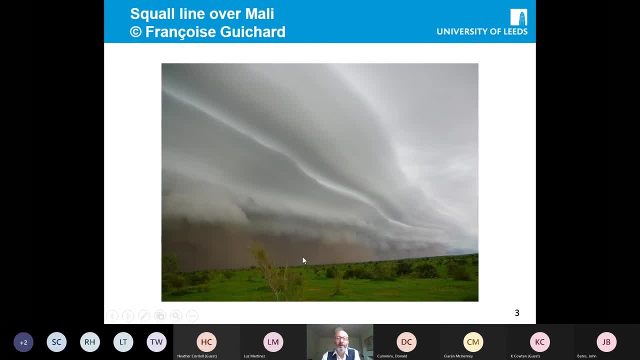 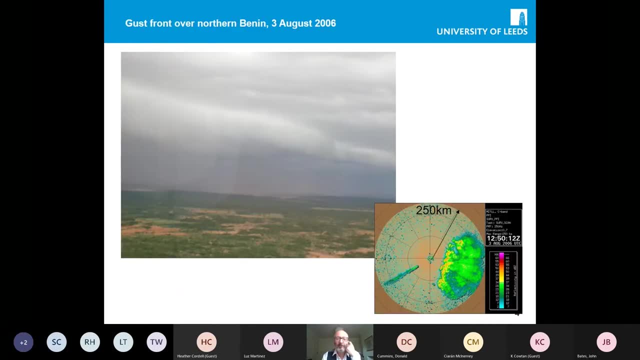 So very dramatic cloud fields and you can see dust being left by that, lifted by the high winds under the cloud there, the cloud edge. Here's one that I took. it's not such a good picture, But this was from a research aircraft actually. So very exciting research flight that we made into. 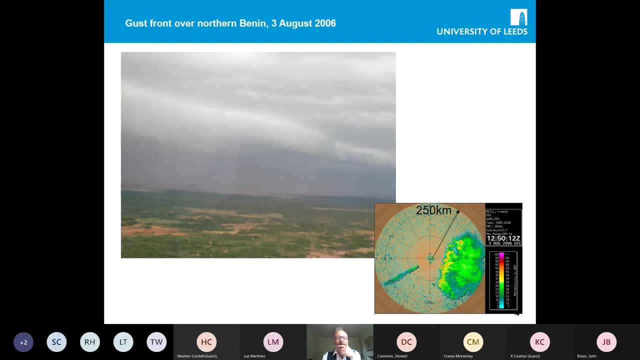 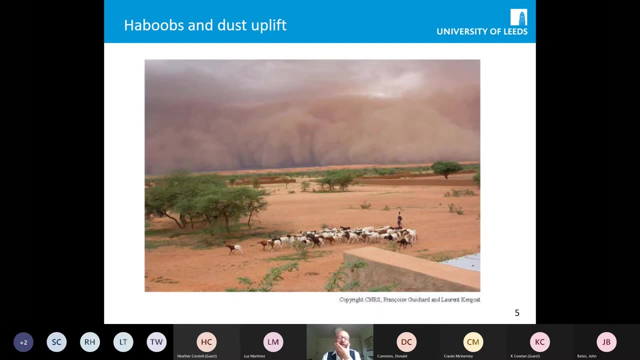 one of these storms over Benin. So again there's some evidence of the dust being being lifted just ahead of the rainfall. in this kind of region here, These storms, they do produce high winds at the surface. Those winds can lift dust. 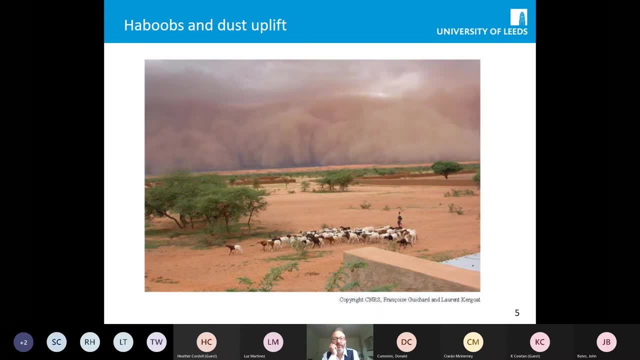 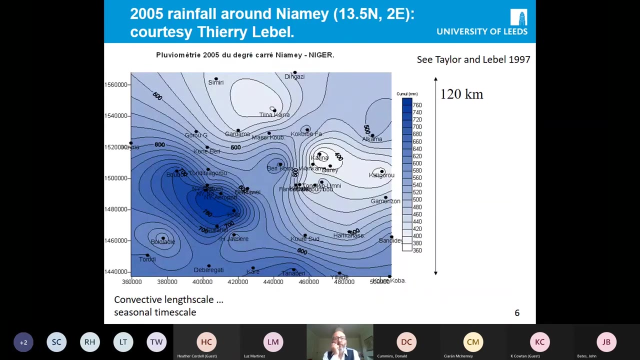 And that cold, dusty air can travel long distances over the desert. So again, thousands of kilometers. So this is the primary cause of these dust storms which are called haboobs in the North African region. So rainfall can be very variable. So these storms that deliver in this region of West Africa, and in the Sahel, the really intense thunderstorms deliver 90% of the rainfall. They come from the most intense systems, So around Niamey, which is the capital of Niger. in the Sahel, then, 90% of the rain comes from probably about 10 or 12 events in the summer, in the monsoon season. So you get these. 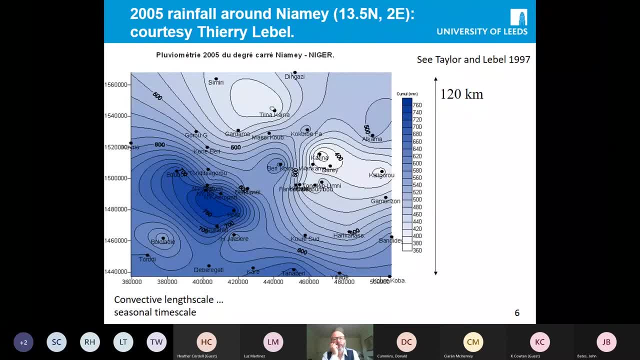 very intense thunderstorm systems And the characteristic of those is that the rainfall is very variable in space, So it's got enormous spatial variability. So it's kind of interesting looking at this map of the. this is the map of the annual rainfall, in fact, for one year around Niamey. 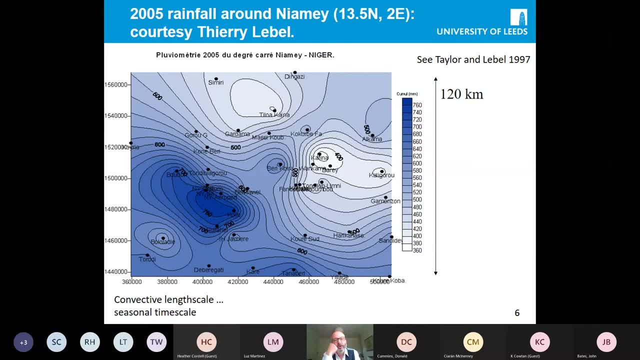 And it's very variable because of the behavior of these storms. So when you think about averaging things globally- I mean I was interested in the first talk- then actually you've got to deal with the fact that you may be sampling across very high heterogeneity on the smaller scales. So the point: 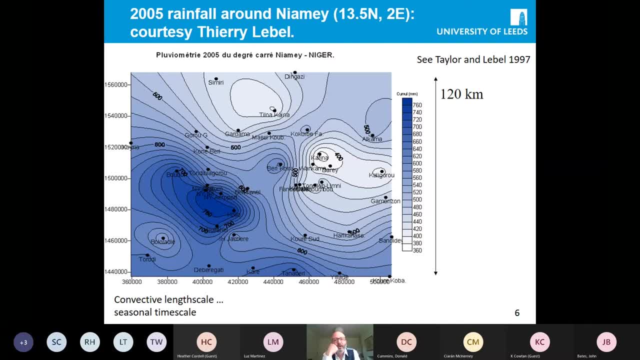 is to show that over 120, this is a one degree square, in fact, around Niamey, And the dots here are rain gauges. These are real measurements. There's very high variability Over a scale of even 10 kilometers. you get a factor of two difference in the rainfall commonly, And that's over the. 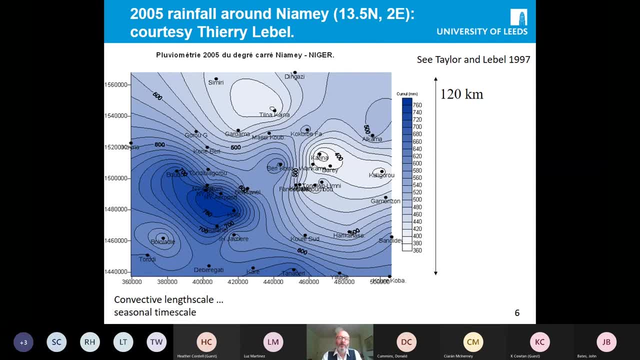 season, And this is an effect of many storms. One of the implications of this plot- and something we don't fully understand yet, or we don't really understand at all yet- is why this heterogeneity is so strong when this occurs over a number of storms. 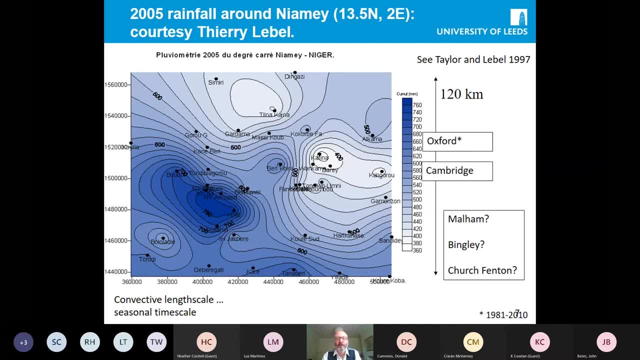 You know, maybe 10 or 20 storms and that we still don't understand that. It's quite interesting to put this into context: actually this rainfall. So I have a good friend, Andreas Fink, that I've traveled with in Africa and he's a real 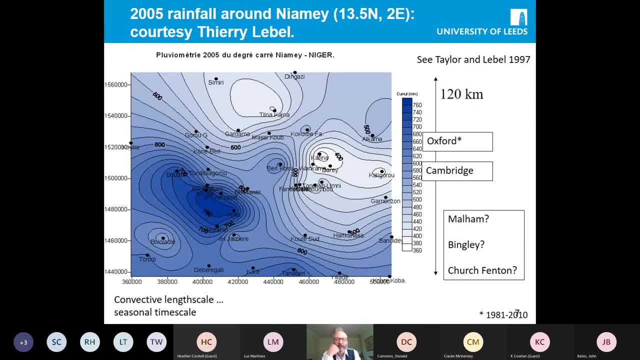 lover of the climate statistics And so if he visits any station, his kind of test of whether they are a good station or not, if they're a good operator, is to ask them their annual rainfall. You know, in conversation he drops it in. 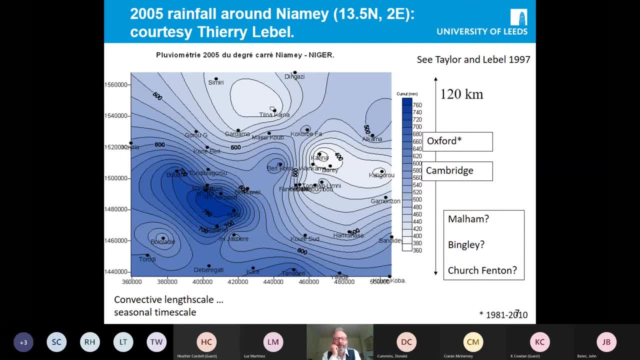 what's your annual rainfall, And if they know about it and have something to say about it, then that's a kind of somebody who's really interested in their data, And sometimes they have no idea, of course. But then he came to visit me in Leeds and I 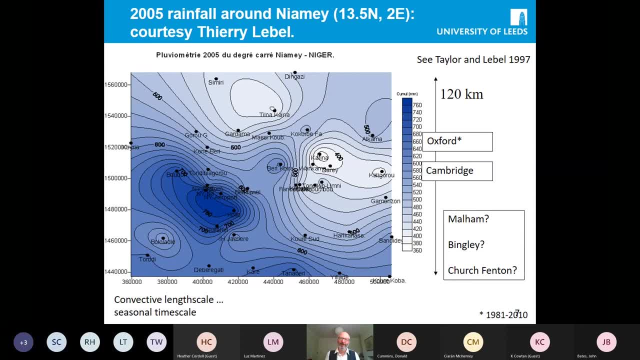 suddenly realized when I was going to pick him up from the train he was going to ask me about the annual rainfall in Leeds. So I had a massive panic and I had to quickly look it up before he arrived. So I do know what it is in Leeds now. So I thought this would be a good test for my audience here. 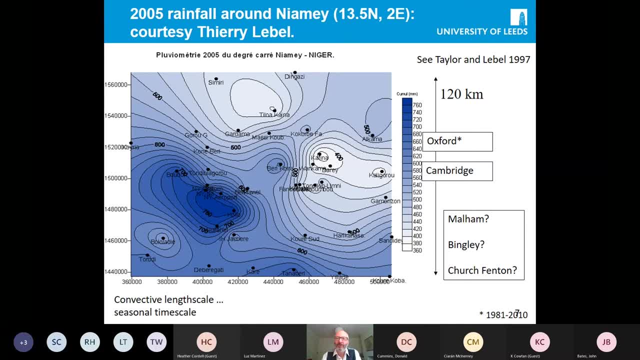 I'll put Oxford and Cambridge on here, just as you know competitor universities for ours. But in fact there isn't a Met Office station in Leeds but Mal and Bingley and Church Fenton are there. So maybe this is a kind of a question for my audience is to see if you know what these are. 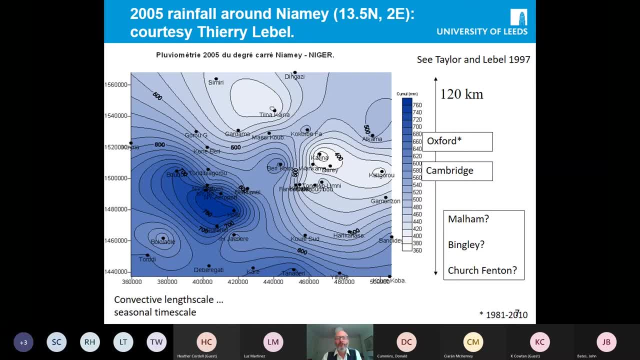 And I'll leave that with you for the time being. So, of course, Oxford and Cambridge. you know UK stations. I've got a similar amount of rainfall to Niamey, But if I showed you a picture of Niamey it looks, you know it's a very alien. 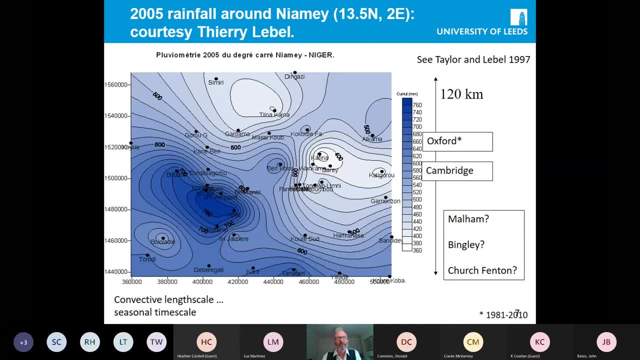 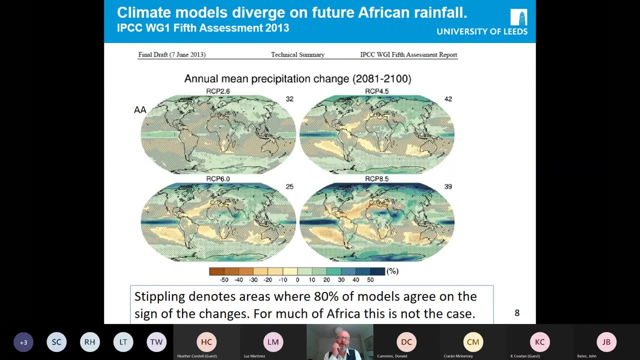 environment. to us, It's very, very dry in the winter, So most of their rain comes in a handful of events which are really, really intense in a fixed window in the summer months of the year. So an important thing to be aware of is that you know other authors, other presenters. 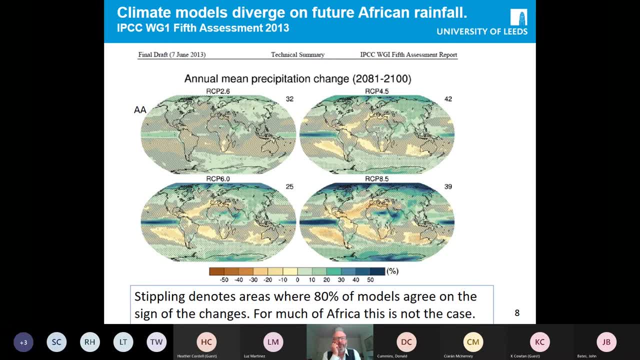 today have been talking about climate models and talking about temperature in particular. But when you look at rainfall, climate models are all over the place. So with temperature, they really follow each other. they track each other very nicely. With rainfall, they are all over the place, So 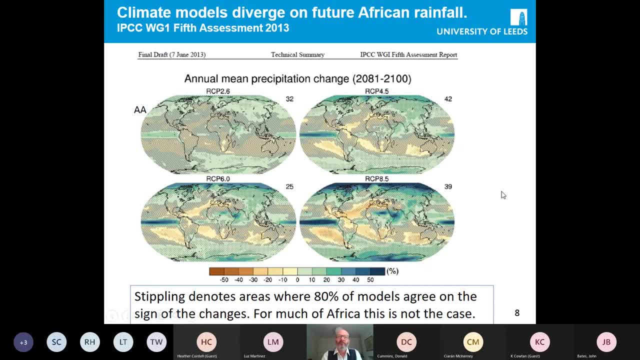 this plot is actually from old IPCC reports from 2013.. But things haven't changed substantially. the message is still the same. There are four plots here showing the end of the century projection for the change in annual mean precipitation There's different. each map is a different emission scenario- RCP. 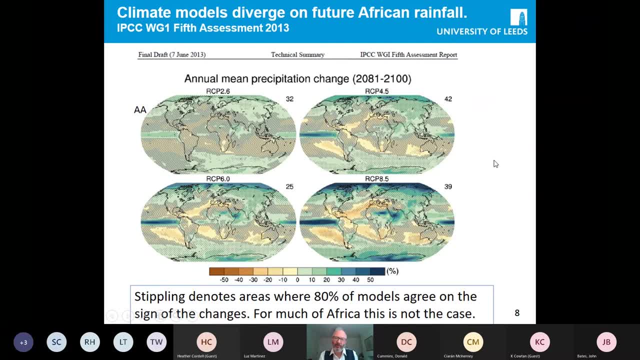 So the bottom right one is the worst case in terms of emissions. The forcings are the strongest anthropogenic forcings And the key point in this plot is the stippling. So this is sort of stippling on the overlying. the colors denotes areas where 80 percent of the models agree on the sign of the changes. 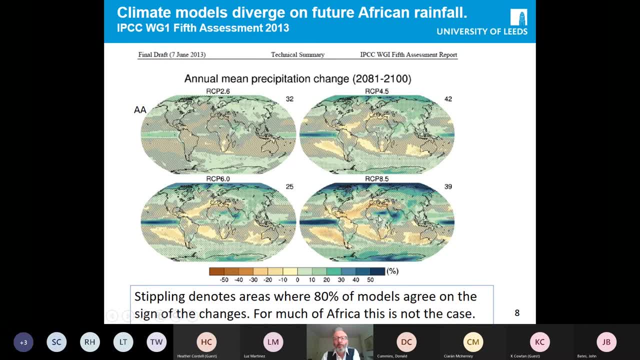 And the sort of shocking part here is that over large parts of tropical continents- you know the Amazon Basin, tropical Africa, India and Southeast Asia- you know models don't agree on the sign of the changes in annual rainfall. So this is really, you know, not a good situation in terms of given that rainfall is possibly the most important thing. 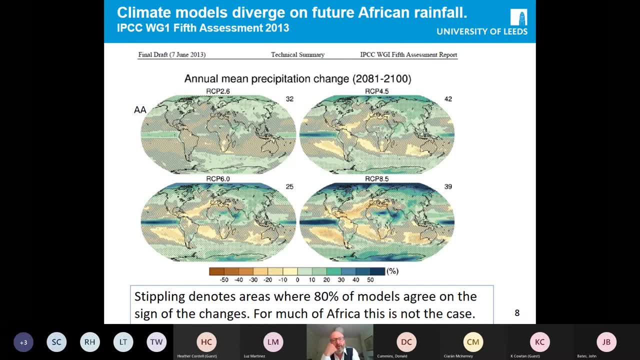 People want to know about for their crops and their livelihoods, And yet we can't give guidance about whether it's going to get more or less in the future. So that's a real problem And it's kind of a wake up call for the research community to try and do this better. 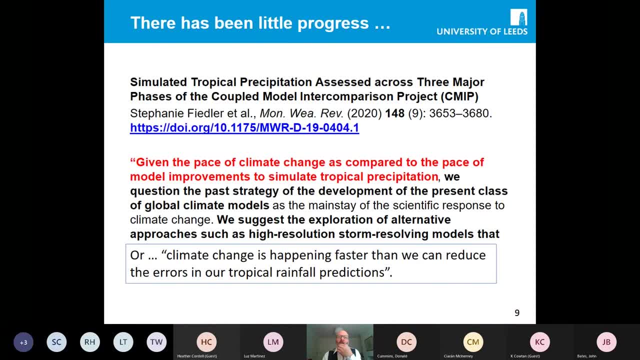 But it's really difficult to simulate. So that was 2013 report. I mean, there's been little progress, So this paper was came out last year. There's a lot of words here, but in the box I've kind of summarized what these points are. 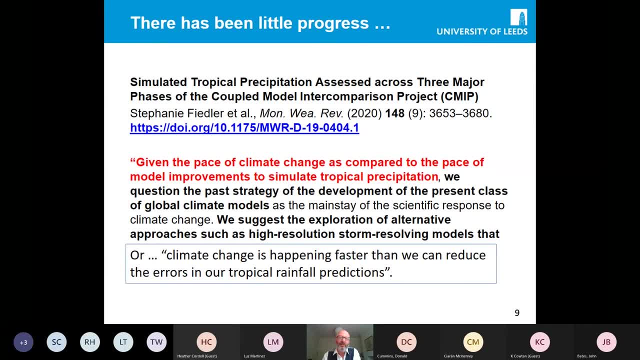 I mean climate change. It's actually happening observably faster than we're reducing. there is in our predictions for rainfall. So you know, we we're actually in a situation where we're just monitoring and observing what's happening. We don't really know the sign of changes. 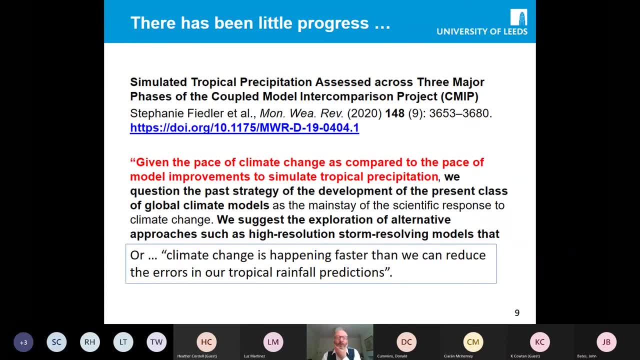 So we need to do better. So I'm just trying to describe, you know, some things we know about or we're kind of working on to to at least give more useful information to people. So we're faced with these very poor climate prediction systems. 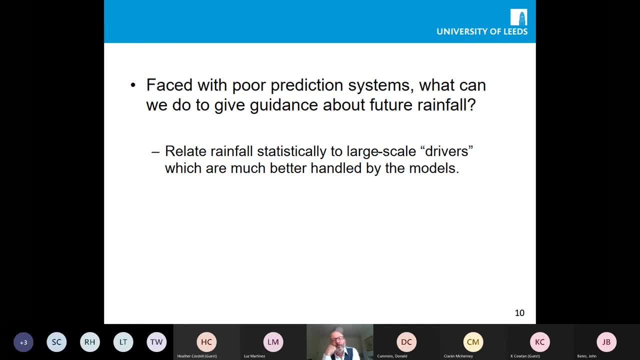 So what can we do to give guidance about future rainfall? And I think one way of thinking is that we don't have confidence in the rainfall in the models But we do have much more confidence in, say, the temperatures and the large scale circulation changes in models, because models tend to be good at those aspects. 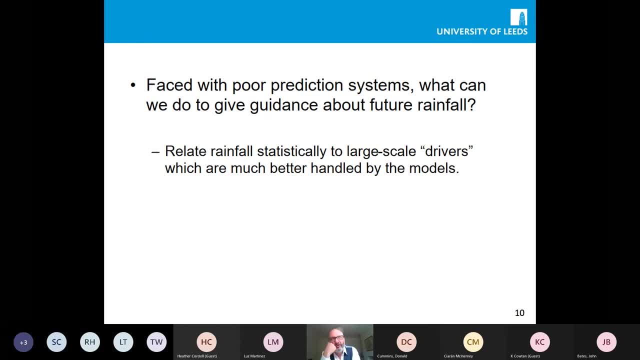 They tend to be good at solving dynamical equations. So if we can get those dynamical regime changes Right And temperature changes, maybe we can relate the rainfall statistically to those changes which are better handled by the models and then then use this to give guidance. 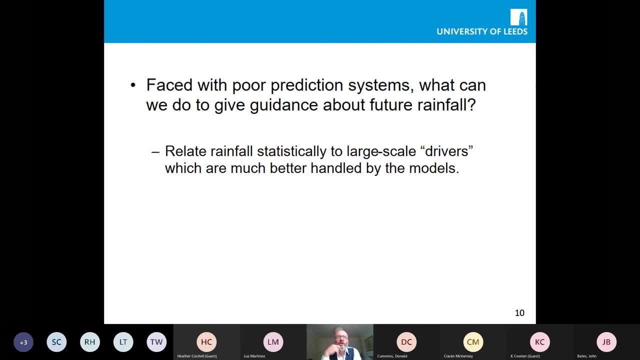 And that seems to be giving us some useful ways forward that I'll talk about. And I'm going to talk about the climate change context of the sort of decades in the future, But people are also applying this on shorter timescales, say monthly timescales. 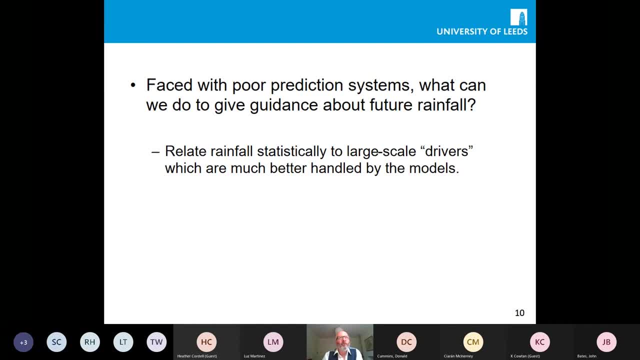 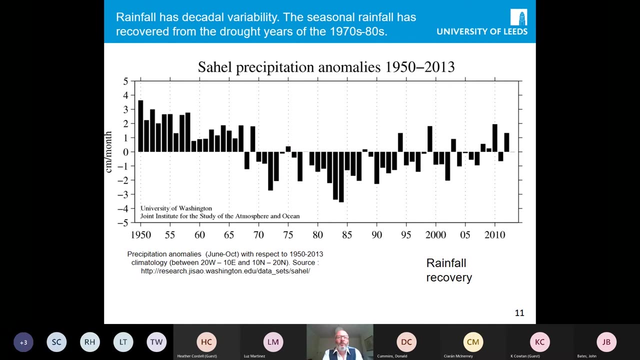 So four week forecasts and this approach of actually Predicting the rainfall statistically on the basis of what the model thinks the circulation will be in four weeks time, seems to be very promising. So I said I was focusing really on the West African region and particularly the Sahel. 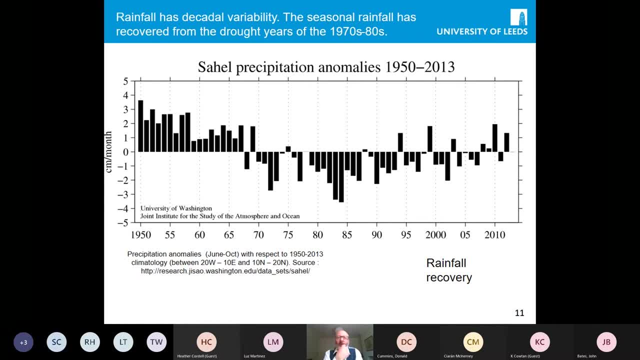 So the Sahel is this band just to the south of the Sahara. A lot of people live here, Millions of people live here, in fact, because because it is agriculturally productive, But but because it's on the margin of the Sahara, it's also very sensitive. 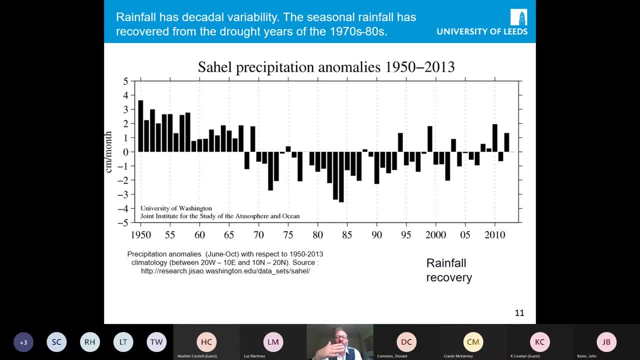 So a small. There's a strong climatic gradients of small changes from year to year have a big impact on people, on the rainfall. So the Sahel suffered a significant long term drought in the 70s and 80s in particular, and those of a certain age will remember the Live Aid concert in the 82 or 83.. 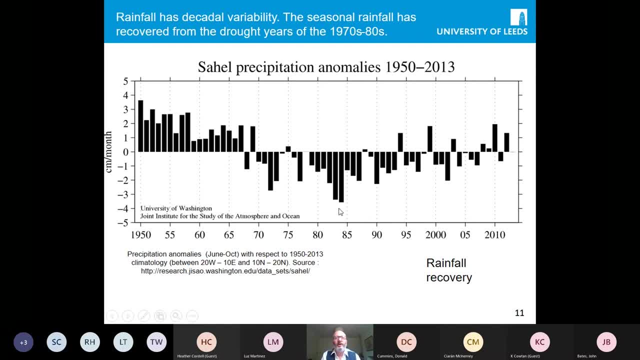 And that corresponded to significant Sahelian drought that you can see on this, on this graph, affecting East Africa as well. So, in fact, the history of this is quite, you know, is interesting because because in the days of independence of African countries from their colonial masters, the in the sort of 50s and 60s, then there's a lot of optimism in Africa, a lot of spending and rainfall was good in Sahel. 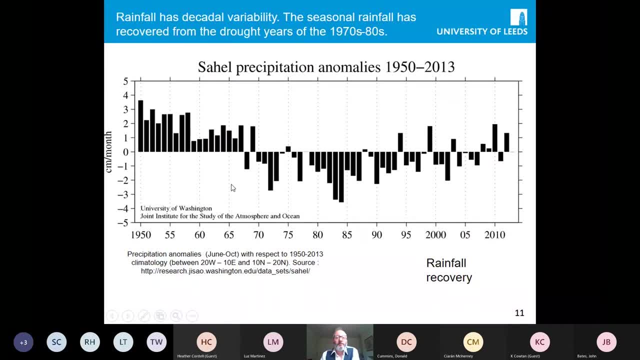 But then, if I go back, the suddenly come the 70s, we have the oil crisis. oil prices went up, A lot of countries were in debt and the rainfall plummeted and the rainfall remained low. And when I started studying This in the late 90s, the big debate was whether this was a permanent change due to global climate change or whether it was due to interannual variable- sorry, a decadal variability. long term natural variability. 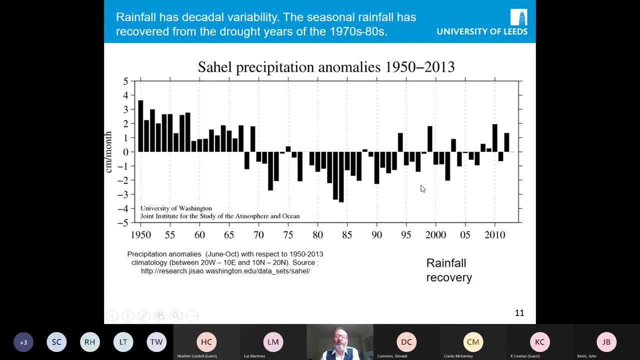 And I think the understanding now is that actually this, this mean rainfall change, has been to do with internal variability. So we don't see this as being a signal of long term global climate change. because the rainfall is somewhat recovered, So you can see, since, say, 2000,. the rainfall is oscillating around some kind of 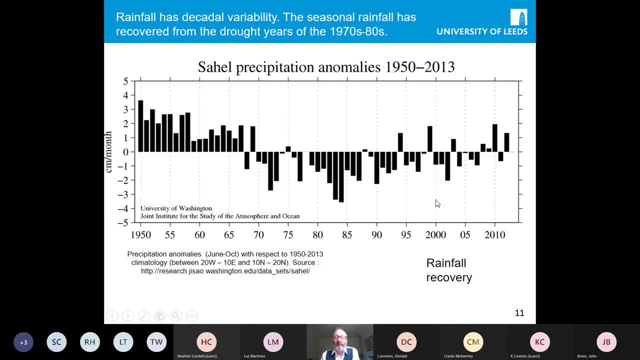 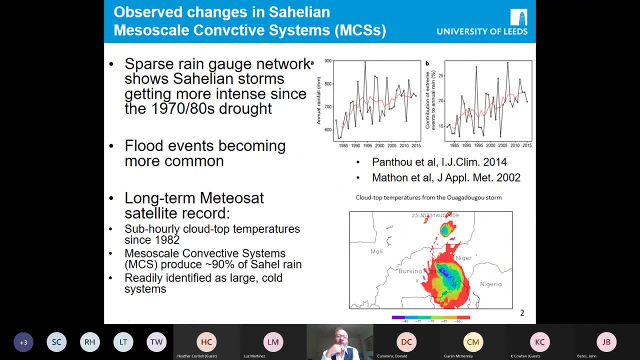 Long term mean, But the situation is more complicated. I'll show more about that. So if you look in more detail at the rainfall- and this is what this, this was done by colleagues in Grenoble in statistics community there, So Jeremy Pontu in particular, this climate paper, the really nice work showing that, although the rainfall, the mean rainfall, has come back to something like 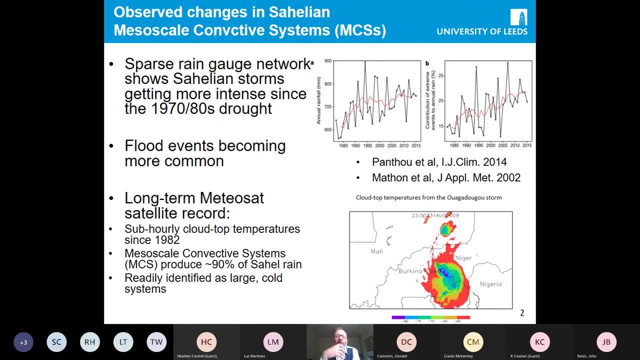 A long term mean and something more consistent with the rainfall in the fifties. In fact, there's a greater contribution of extreme rain to that that rainfall. So, although the mean has come back, the distribution of the rain has shifted to one where there are more intense storms and, associated with that, there are longer gaps between them. 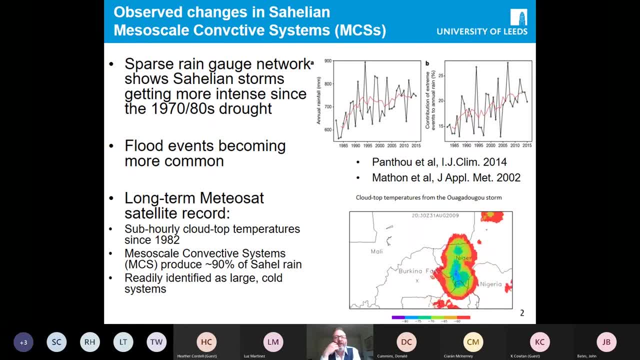 So the statistical distribution of the rainfall has changed. So flood events? Well, flood events Are seen to be more common, but that is associated with this shift in the mean. So so just to show what that is, the annual rainfall is the left hand plot in the top here. 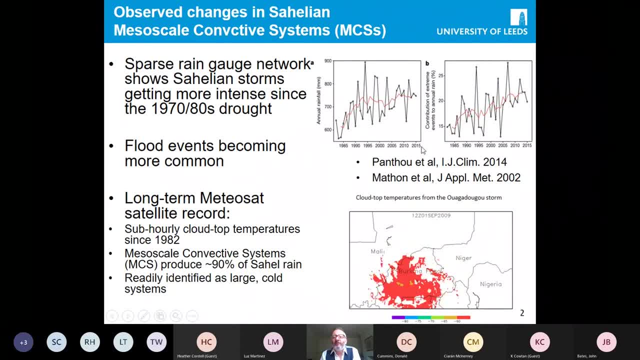 Sorry, just to explain it by year: since 1980,, I think since 2017.. And but the contribution of extreme events to that is the right hand plot, going up from 15 to 20 or more. So what I'm going to show now is some some extension of that work. that work was based on rain gauge data. 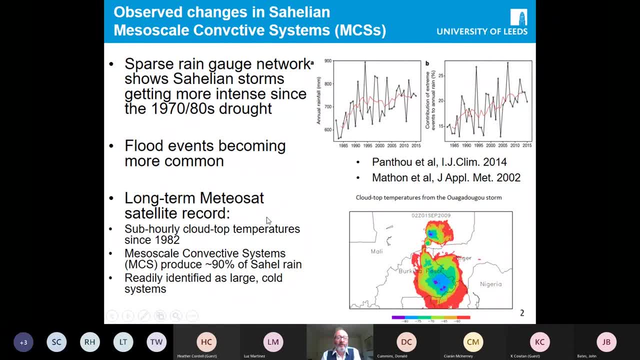 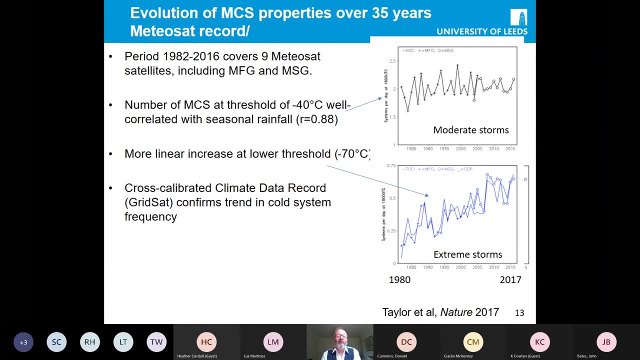 So extension of that to look. So what I'm going to show now is looking at satellite data from the Meteosat record that goes back to 1982, so nearly 40 years now. so again looking at these really intense systems, and there's a movie, if you can see it, one coming across here. so this is work that's primarily done by Chris Taylor, CEH, Central Ecology and Hydrology in Wallingford. 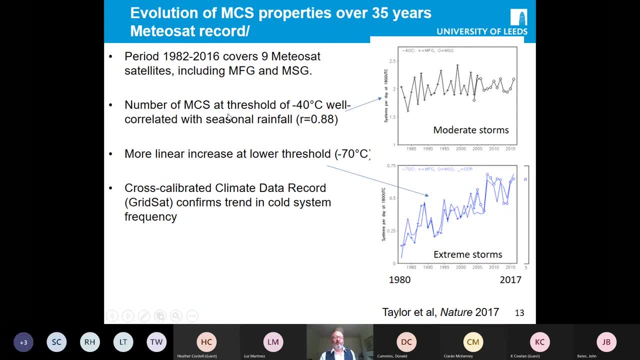 So what he did was to analyse these storms and again look at the trends of these. So over the satellite record he looked at the ones with the Cloud top temperatures of minus 40 degrees C. so these are sort of moderate. in the UK these will be the most intense storms you know we can imagine, but in this region these are the moderate ones and in fact if you look at this it's not showing exactly here, but the correlation with seasonal rainfall is is relatively high and and there's there's no obvious long term trend in these storms. 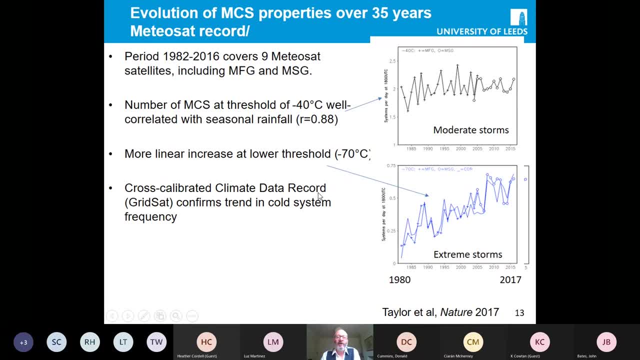 But if you look at the extreme storms that go to minus 70 degrees C- so these are really high in the troposphere, Very, very intense Precipitation, a lot of lightning- then actually the frequency of these is tripled. 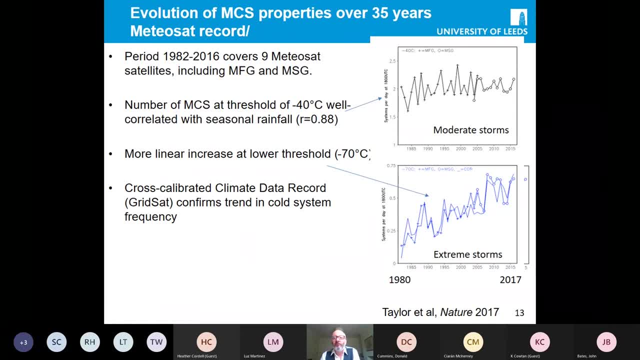 So this was the headline for this paper. the frequency has gone up from, you know, point two or something- systems per day- up to point six or so. So really significant increase in these very intense systems as the mean rainfall has come back to normal. 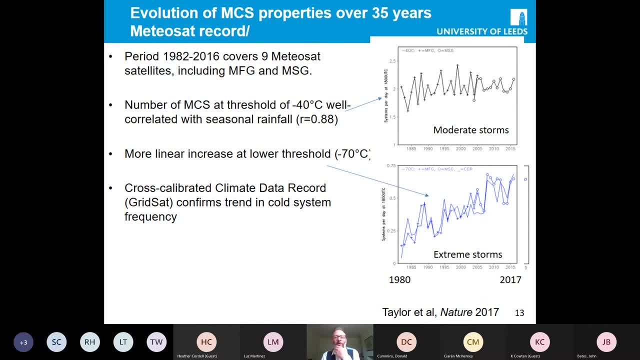 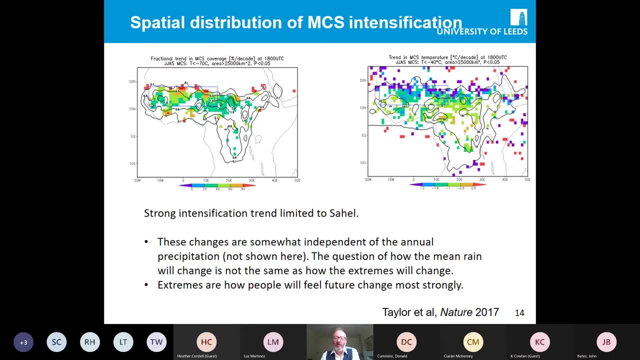 So in many ways the mean rainfall coming back has been very good for the local populations, But but it's coming, It's going to come with it with this increase in very dangerous storms. We can look at the map of these systems and the map sort of if you look at the top left here, this is the the map of the trend. 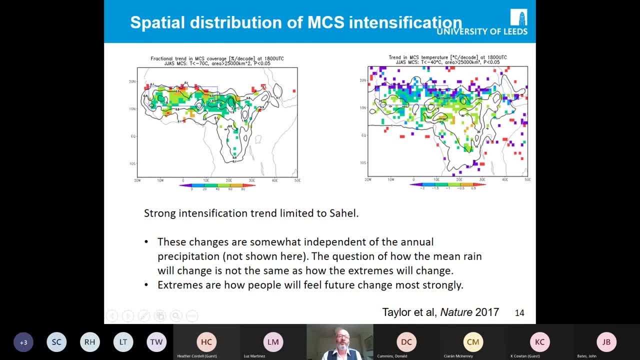 So where the trend is significant it's colored. So we see this is really confined to the Sahel. This map almost defines the Sahel zone. There may be some patches elsewhere in Africa that may have some significance, But really it's this. 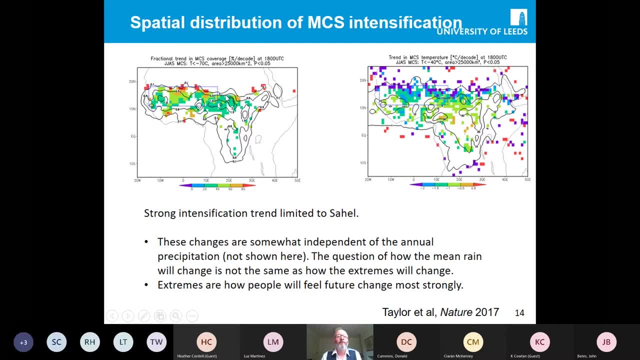 This belt running south of the Sahara and not shown here. As I mentioned, these changes are somewhat independent of the annual precipitation, So the change of the extremes are not seemingly related to the mean in a given year there, But but the increasing trend is is the dominant observation. 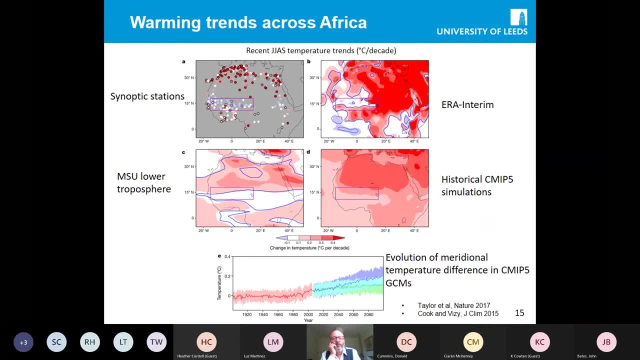 So what Chris was able to do In investigating this more deeply was because he had the satellite data and he had this consistent record over 35 years at the time. then he was able to relate this to measures of the drivers. So the larger scale situation associated with these intense storms. 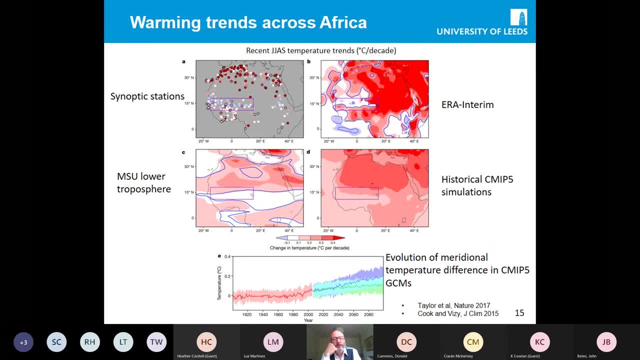 So here's another illustration of the challenges of of understanding. So this is a temperature, So I was so interested to see the first talk in relation to understanding temperature. So So Chris's approach to trying to understand this complex Problem was just to show you four different approaches of understanding temperature. 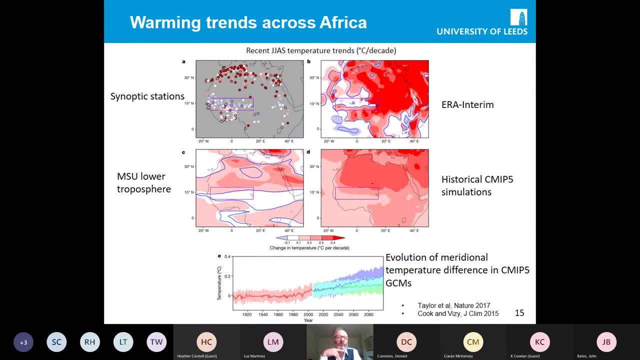 So these are the warming trends, degrees C per decade from four different measures. So the surface stations are shown in the top left era. interim is the reanalysis. So that's what we mentioned in discussion with Kevin. Then historical model simulations: seem at five simulations. 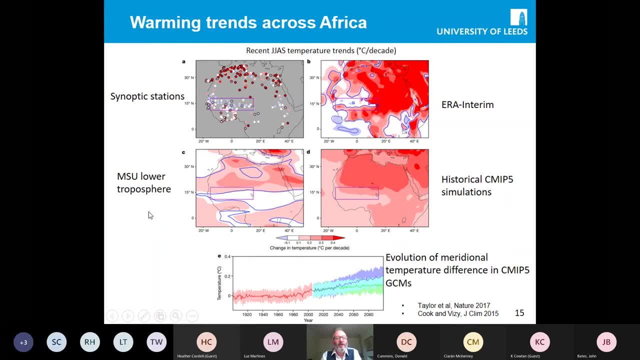 This is the climate models which we talked about just in the last talk, And then the satellite measure in the bottom left. So The Generally consistent conclusion from these is that Sahara has warmed a lot, and probably warmer than everywhere else. I think you also saw this in one of the movies that Kevin showed in the first talk that the deserts around the globe 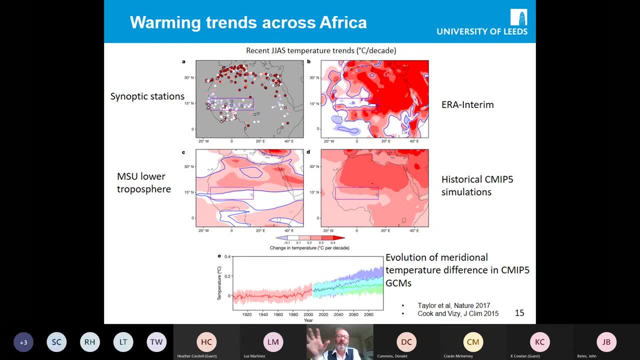 In fact it's observed- and there's a good physical explanation for this- that the deserts are warming and will warm faster than other regions because of the sensitivity to water vapor in the radiative forcing. So the desert is apparently warmed faster than other regions. 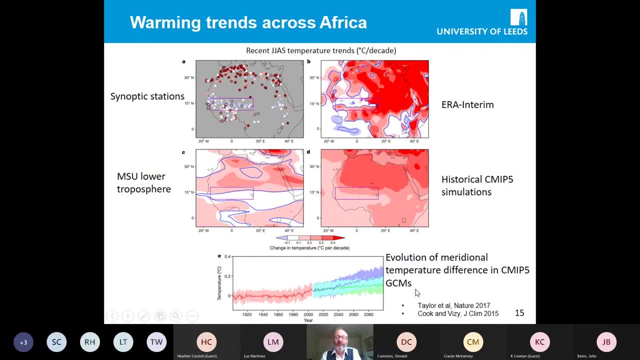 And then the climate model projections in the bottom panel show this continuing. So the temperature- meridional temperature difference- is projected to increase, And the other thing to read from this, though, is this Sahal Zone on the edge of the Sahara. 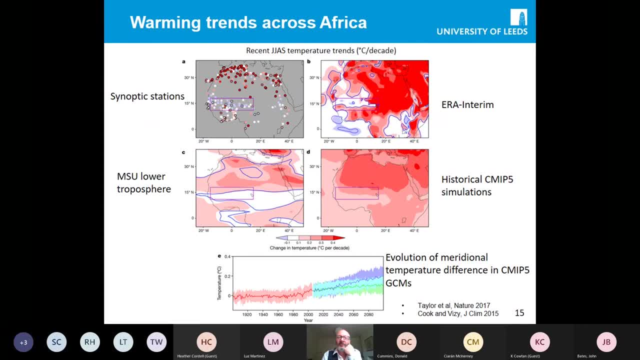 So the purple box here doesn't have a very obvious increase in temperature over this record. It certainly appears to be. it's almost at a minimum. So it appears that the There's not a clear increase in temperature, in temperature And also it's not shown here, but the humidity is not clearly increasing in this. 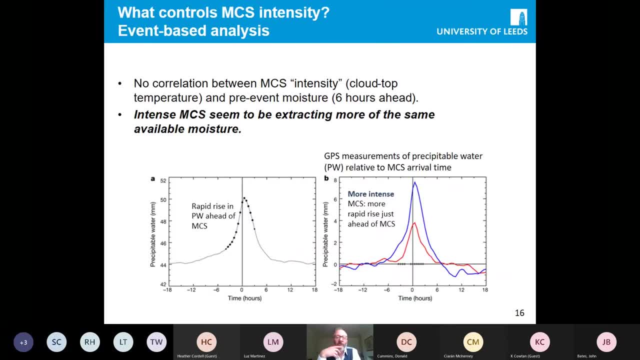 region. So we looked at the humidity more closely And these are observations, in fact, storm by storm. So these are from GPS measurements. So GPS measurements, with an observing station at the surface you can measure the column water, so precipitable water, So PW is precipitate, Oh, 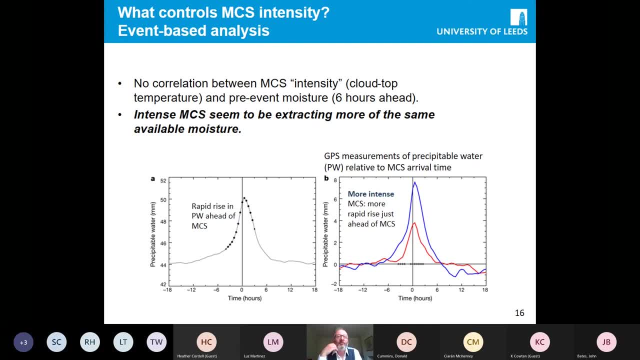 I need to explain my acronyms. I'm sorry. Just somebody shout out if I haven't explained something. some meteorological jargon. But MCS is mesoscale convective system, So that is the big organized storms. So looking at many of these storms at the surface of the GPS station, 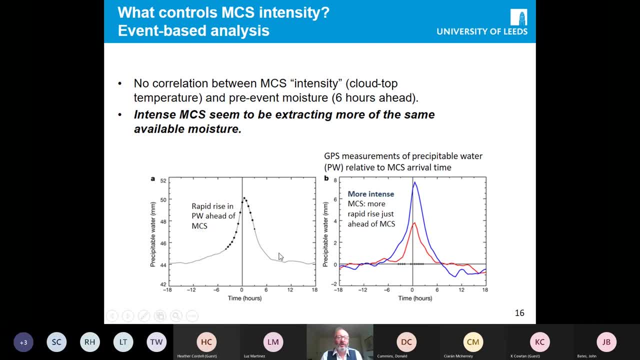 you find that as a storm arises you get a big increase in the column water, the precipitable water. So it's something like six, so maybe 15%. But then if you compare the most intense in the right-hand plot and the least intense storms, the most intense are the blue and the least are the 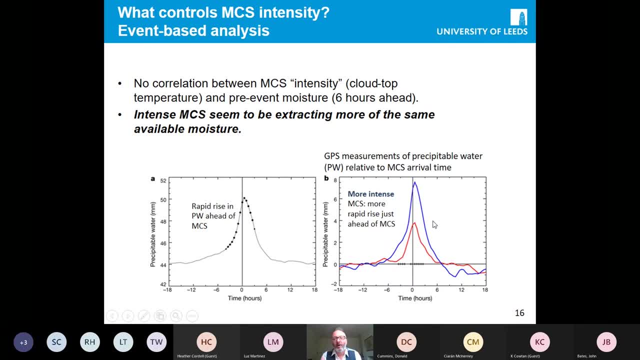 red, you find that the most intense have a much bigger increase in their column moisture as they occur. But if you look more than six hours ahead, there's no particular evidence of that. So this suggests that the storms are not more intense because they have a more intense environment. 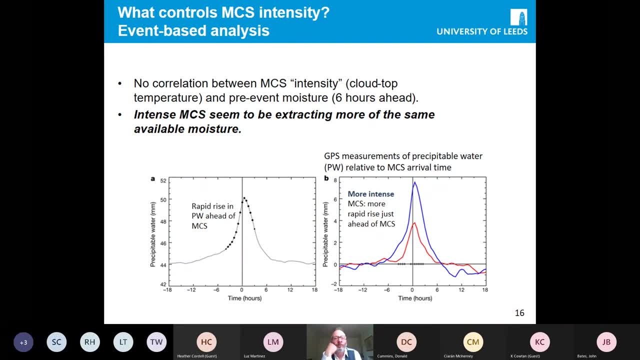 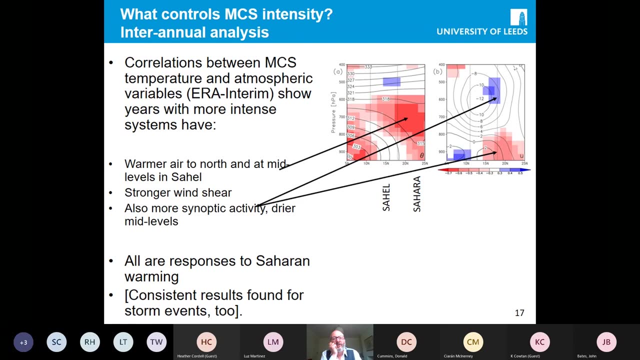 but more intense because they're somehow milking more moisture out of that environment. So the intense storms are extracting more and more moisture out of that environment. The same available moisture is an inference from this. But if you look at what is associated with the intensity, well, the first thing that we saw in 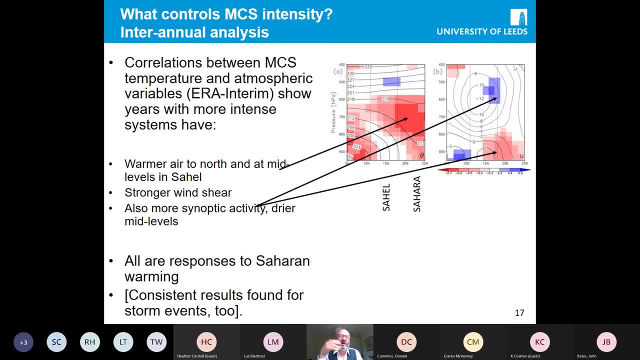 the trend was that the temperature difference from the Sahara to the south is a strong relationship- is also increased And, to go into the meteorology of this region, in fact the temperature difference from south to north, from essentially the Guinea coast and the ocean, which is cool, into the Sahara, which is hot. 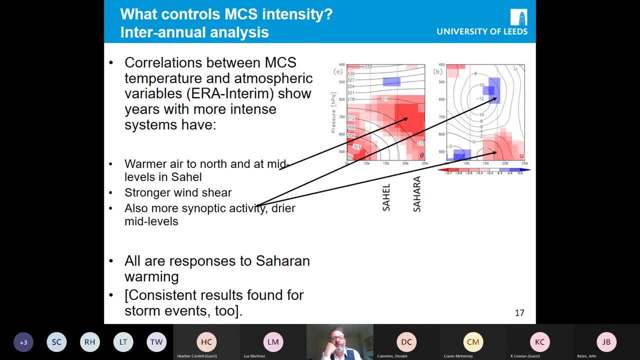 that temperature gradient is associated with a jet from the east. It's called the African easterly jet. So the plot on the right. sorry, I should have explained my axes. I'm used to a meteorological audience. So the y-axis on both these panels is pressure decreasing upwards. So 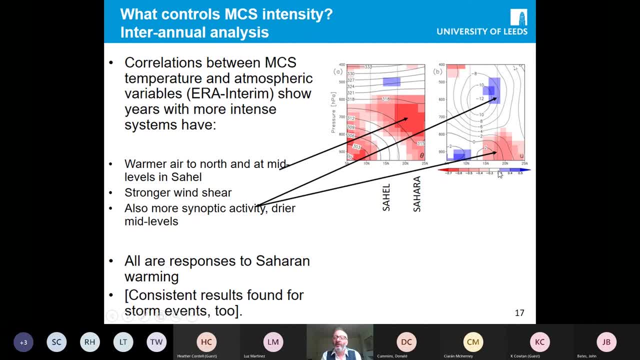 that's basically height, is the y-axis And the x-axis here is latitude going from 5 to 25 north. So the right-hand of these plots, the y-axis here, is latitude going from 5 to 25 north. 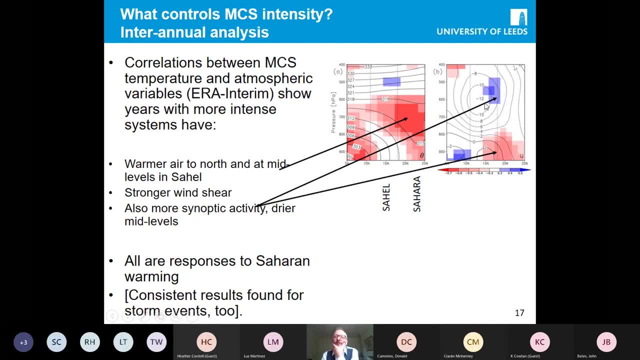 The contours are the African easterly jet. So it's blowing into the page, into the board, at a height of about 4 kilometers, a value of minus 12 there. So there's a jet flowing into the board here. So that's the sort of West African equivalent of our jet stream. Our jet stream is: 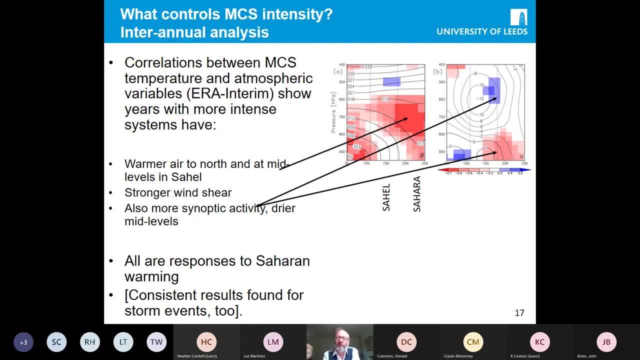 higher up, but it exists for the same region. Ours comes from the west because it's cold in the north And in this region it's hot in the north, so you get a jet from the east. So what we see in terms of the trend is an increase in the. 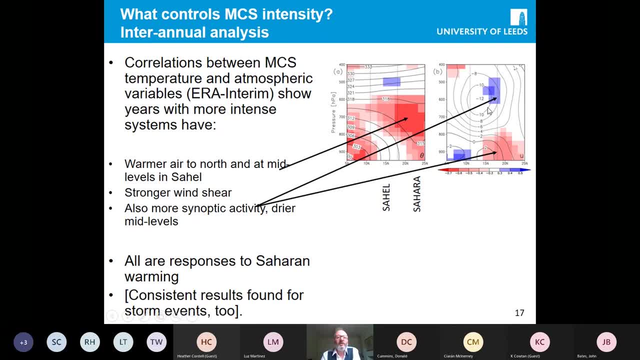 jet and a shift of this to the north. So the correlations point by point between the MCS temperatures, so the coldness and the intensity of the storms and the atmospheric variables, has got these signs. So we see an increasing of the easterlies where this blue is in the top right. 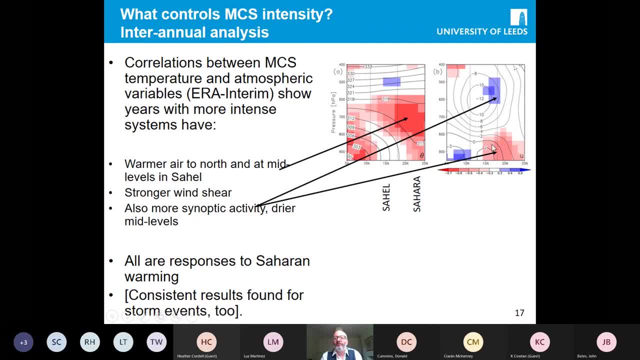 increasing the jet and moving to the north and then increasing the westerlies at low levels So that together increases the difference in the wind. That's the wind shear. So we're seeing a stronger wind shear. We're also in the left-hand panel. we're seeing warmer and in fact 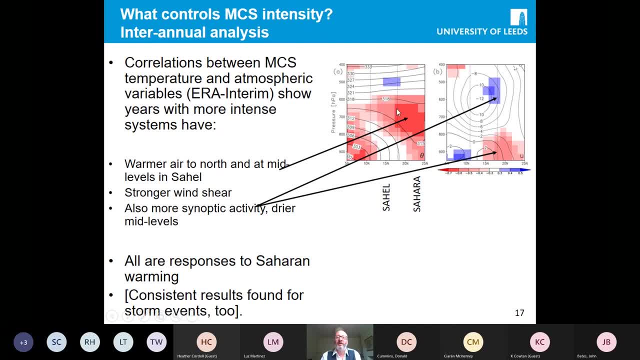 drier air- The dryness is not shown- but warmer air at mid-levels here. So both of these are consistent in the understanding of how these storms organize. This wind shear is known from many, many studies, say in the USA, around the world. It's something which intensifies and 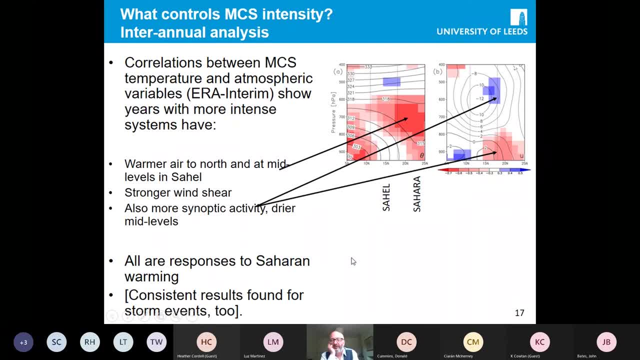 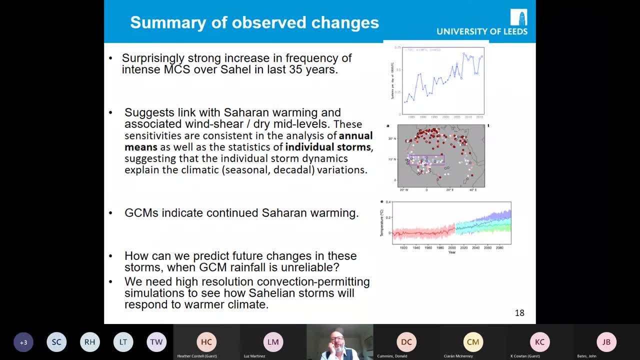 organizes storms. So the conclusion from all this, from the observations of this region, is that the storms are intensifying or have intensified in this threefold increase in the most extreme storms, as a result not of the temperature and humidity increasing locally, but as a result of: 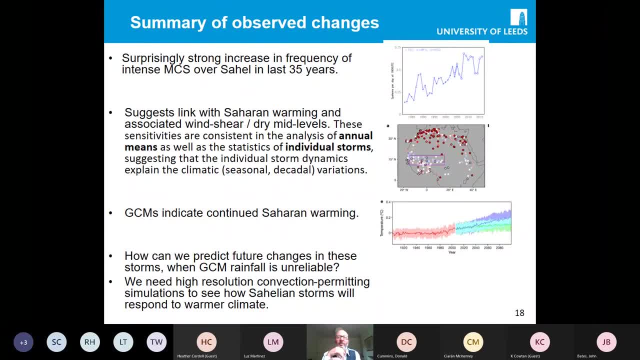 the dynamics changing, the wind, shear increasing and possibly the mid-level temperature and dryness getting more dry. So essentially, the message we have is that the storms are getting more intense because they are becoming dynamically more effective And then dynamically they're able to take more moisture out of the same supply. So it's an 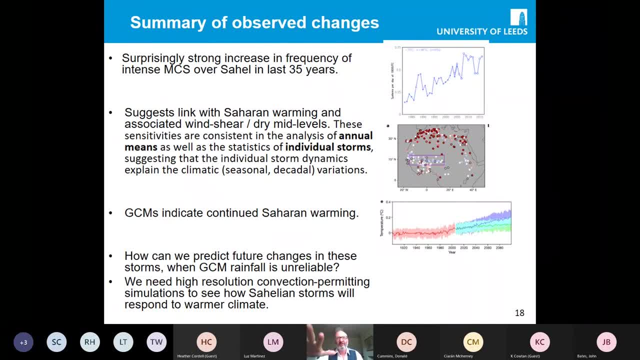 interesting case where the effect of climate change on the large scale creates this large-scale gradient, changes the large-scale flow and that makes the storms dynamically more active and in turn generates more rainfall- not by just simply increasing more moisture, So increasing moisture. So this is quite different to the simplest thought picture we have of how. 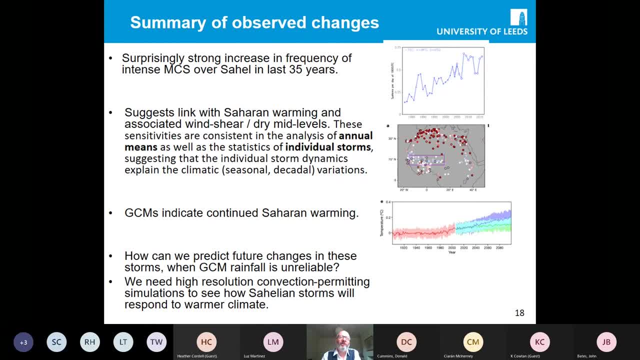 rainfall changes globally, Which is a sensible one, is that if you increase the moisture available globally, then rainfall increases because there's more moisture available, And that overall is true, But in this part of the world, the rainfall, the moisture hasn't changed. But what has changed is the storms have got more intense. 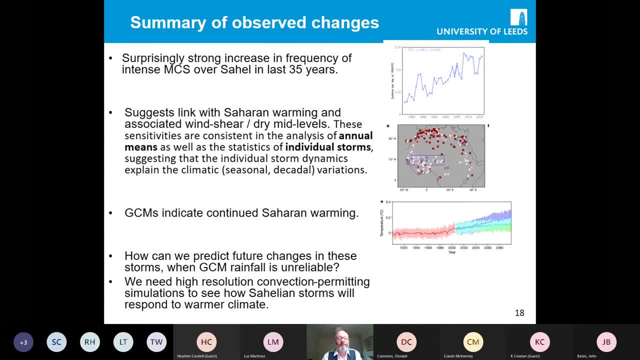 and therefore they extract more moisture from the same environment. So there's a problem in the bottom two bullets here. So how can we use this kind of information to predict future rainfall? Because the GCM, the model rainfall, is unreliable. So the principle is, if we can look at the drivers. 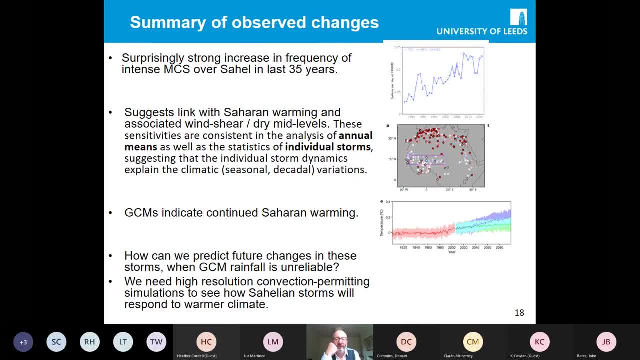 we've got a driver here- which is the temperature gradient from the Sahara to the south, and the wind shear. So our premise is that we could use that as a proxy for the rainfall, And so what we're going to use is very high-resolution. 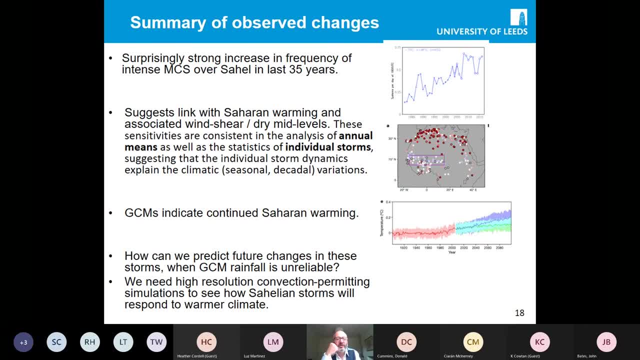 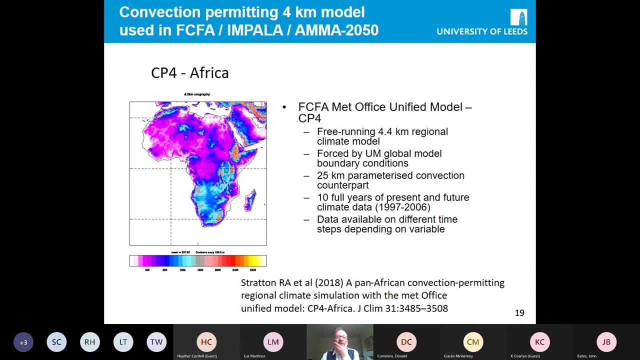 model simulations where we do have confidence in the rainfall prediction to see how the storms will change in a warmer climate. So we do have these simulations for Africa, And this was from a project called Future Climate for Africa, And the Met Office ran a sensationally high-resolution. 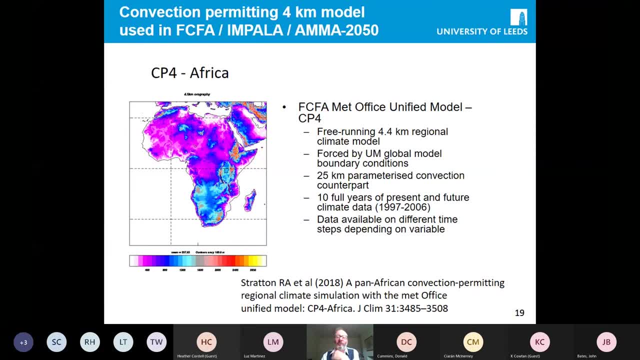 climate simulation for Africa at a resolution of four kilometers. So this is now enough to represent the biggest storms properly in the model, And we find that the model representation is transformed. So the models are represented much, much better. We can't run this globally. 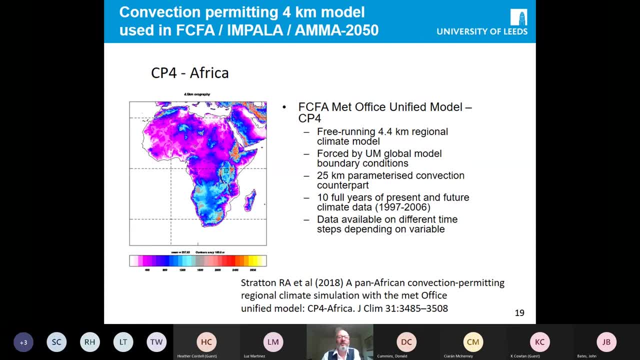 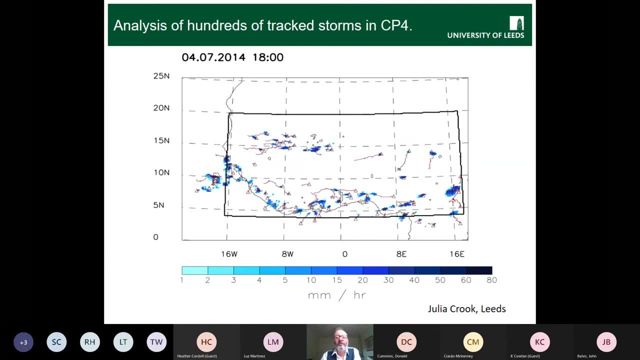 because we can't afford it. So we can't do this for a climate simulation, but we can do it for a regional area And we can look at these drivers. So in the model these are the size of the storms, So the tracking of these is automated. 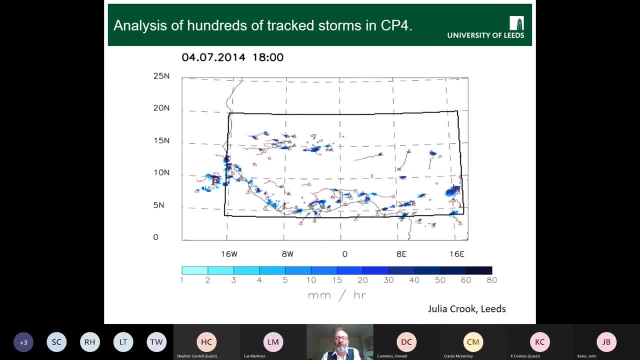 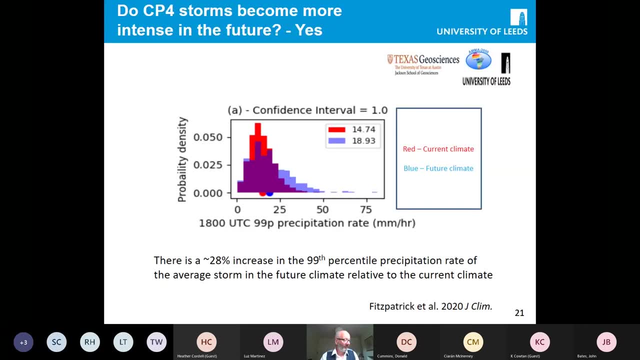 So the storms are identified as objects in rainfall or in cold cloud and then tracked And we can look at the properties of those statistically And just look at my watch In the model. the model is very expensive So we can't run it for long periods of time But we do. 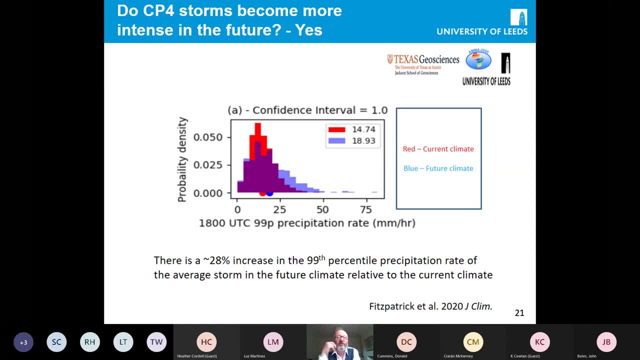 have a 10-year current climate period and a 10-year future climate at the end of the century. So do they become more intense in the future? And the answer is yes. So we do see a significant increase in the intensity of the storms. So that's in this distribution. So within each storm we find 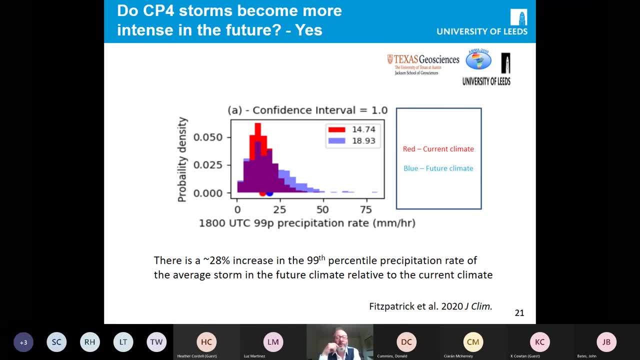 the peak of the rainfall, That's the 99th percentile within that storm, And then plot the distribution, the PDF, of those values for current and future climate And we find an increase in the peak storm intensity distributions And the tail here, of course, in terms of intensity. 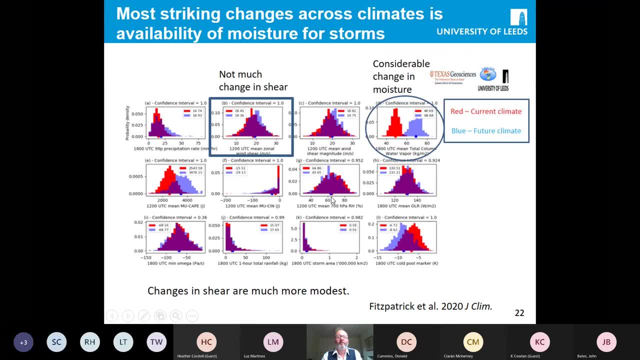 is what's important, the really intense ones, And then we can look at the drivers of these And then we come up to a kind of a challenge to our understanding, Because actually, when we look at this future change going 100 years into the future, or actually 80 years into. 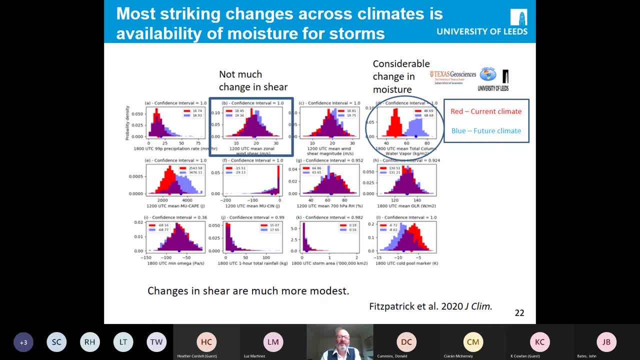 the future. now we find that there isn't much change in the shear. So while there is an increase in the shear, but it's not very much, It's going here from the mean of 18.43, second to a mean of 19.36.. So there is an increase in the shear which will be consistent through the model I just showed. 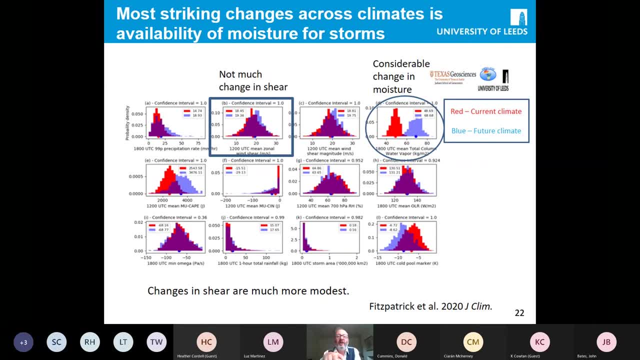 you and through our understanding of the past data with intensifying rain. But when we go to the future we find that the moisture distribution is totally transformed. So we have distributions that barely overlap, So because the temperature has increased so much in the model simulation, then we have a 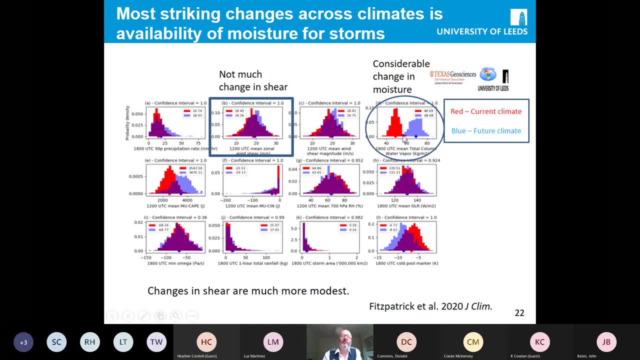 really different. So this is what we didn't see in the observations. We didn't see a significant change in humidity over the past 35 years. But going forward to the end of this century, we see this enormously in the projections And we have some confidence in that. 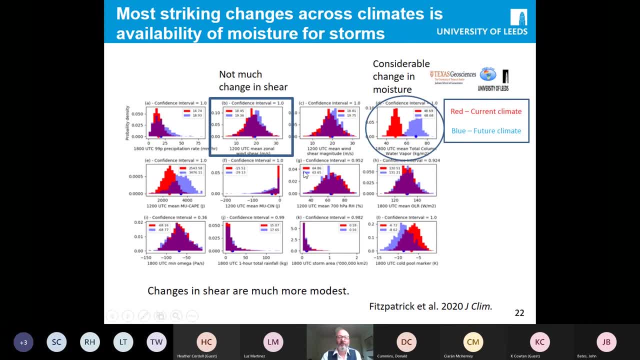 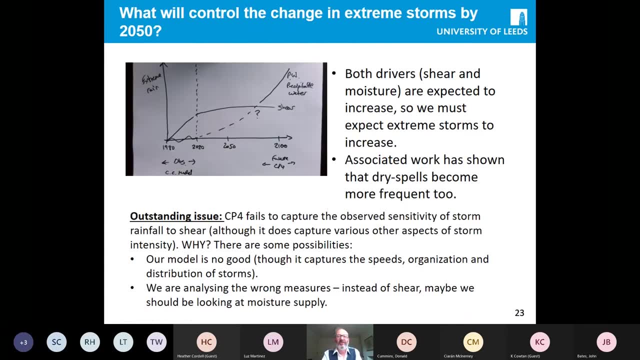 because it's one of these large scale measures that the models are good at generating. So, in fact, we have a sort of a. this is the point we've reached at the moment, I think. to try and encapsulate where we stand, We see two really important drivers of the intensity of rain. 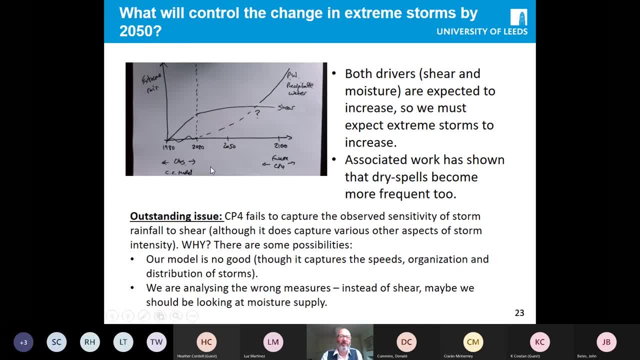 We see shear is and if I put this in the sketch which we've used in our projects to some extent, if you look at the observational period from 1980 to 2020, then the shear is increased and the precipitate of water is not changing. So that's the point we've reached at the moment, I think. 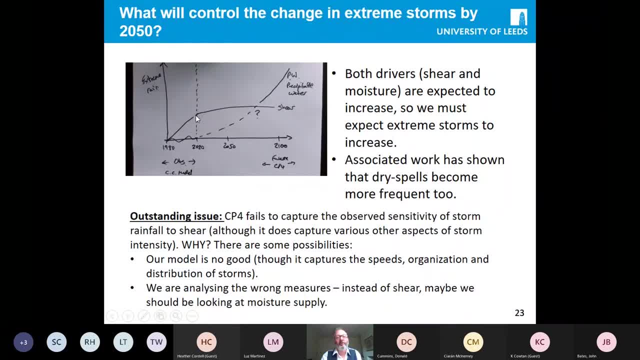 And the more we look at the future, the more we see shear change very much. So over this period we've seen storm intensity dominated by this. But when we look to the future then we don't see shear increasing so much. But precipitate of water takes off and follows a steeply increasing curve. 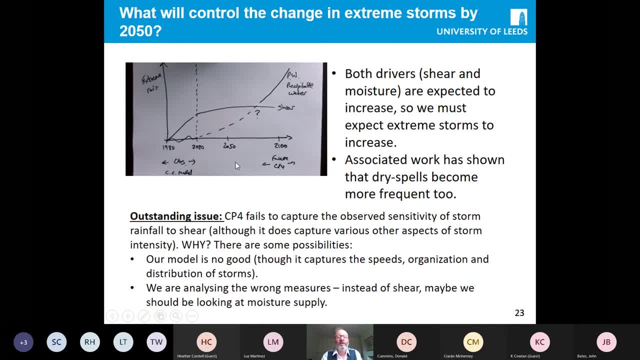 and it is a very nonlinear function of temperature. So which of these dominates the extreme rain? Well, when we look at our simulations for 2100, our future simulation- then the precipitate of water dominates the changes. But if we were to look at an intermediate date, 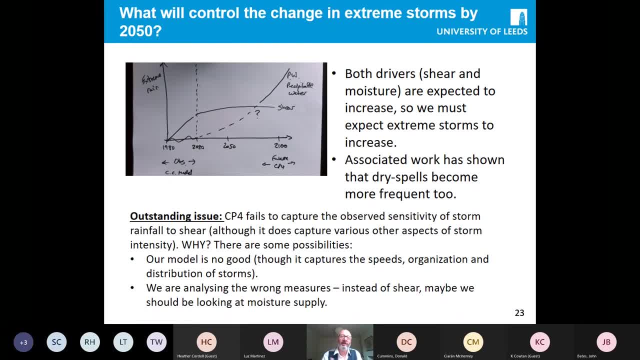 like 2050? we don't know yet because we don't have simulations there, and and so this is the point we're at, i think, in terms of our work- is to try to to understand how these two play out in. in the meantime, the one thing we can say with these is they both go in the same direction, so so it's not. 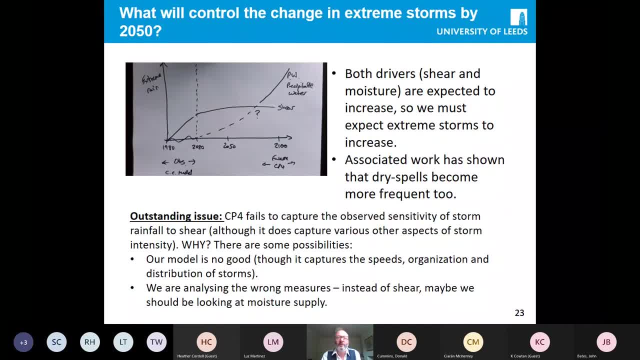 like these two effects are competing and we're unsure what the sign is. we're really quite, we're quite uh clear that storm intensities have increased significantly. well, when i say significantly here, i don't mean statistically significant, i mean significantly in terms of the impact on people. 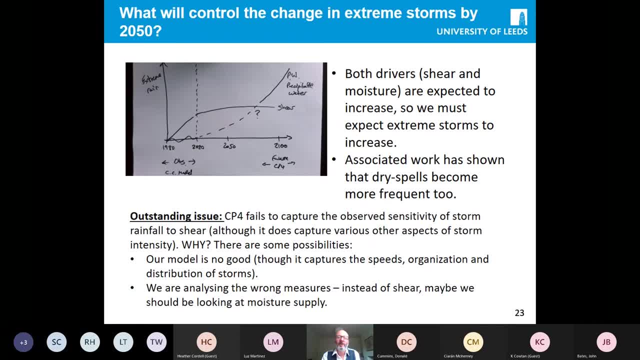 you know, in in a, um, a way which is significant to people, um they over the last 40 years, but but um, and we, the drivers that we understand uh, are both consistent, the both of these drivers are consistent with this increase, uh continuing um, uh in a in a, you know, a uh important way. 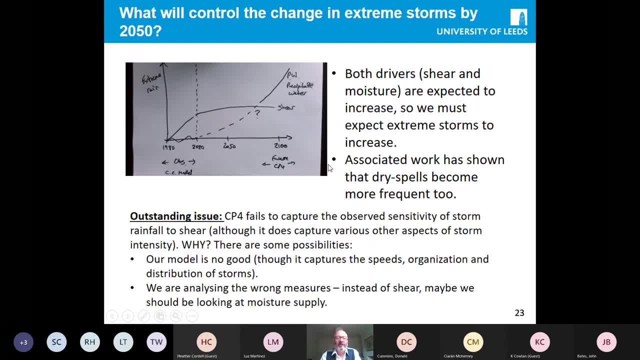 uh, there's a, There's a challenge here in this fantastic model that we have. It gets so many things of the storms much better, but it doesn't capture the driver, the shear driver, very well. This is a kind of a technicality, I suppose, in terms of my conclusion. 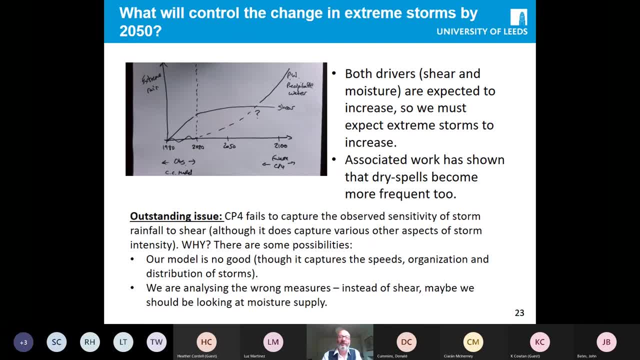 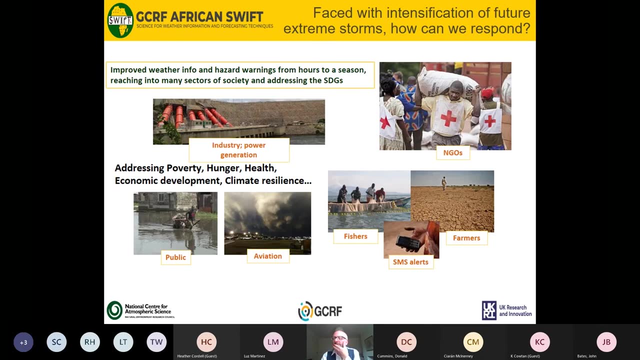 It doesn't affect the conclusion, But in terms of taking this, it doesn't affect the conclusion because the shear isn't changing much, But it is a headache here And so we are looking into understanding that in our work now. So I said in my abstract: 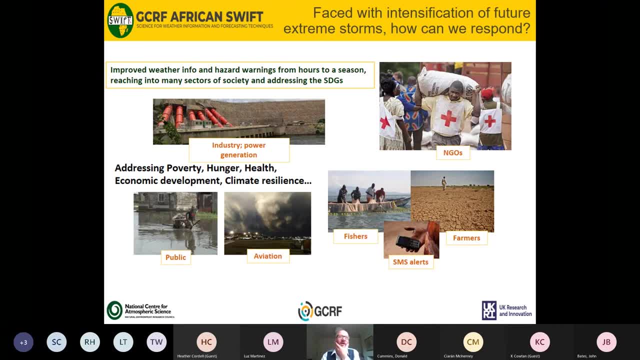 I wanted to talk about extreme timescales of prediction, So I've talked there about decadal and to the end of the century projection, But again, when we're giving guidance to people in the region, we say that the storms have increased in the Sahel. 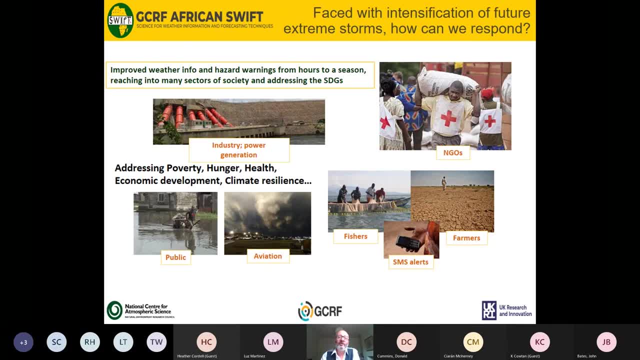 and we're expecting intensification of future storms, And we're expecting that across Africa, because when it's dominated by the humidity, then that is just a. It's something that's not really so dependent on geography. So we need to do something now. 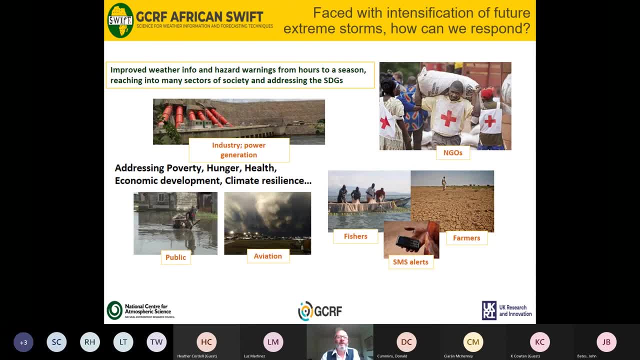 And climate change, in this sense, is not hypothetical, It's a reality at the moment. We were talking about 25 years ago, hypothetically, but now, 25 years on, here we are. We're in the middle of it, So we have to do something about it. 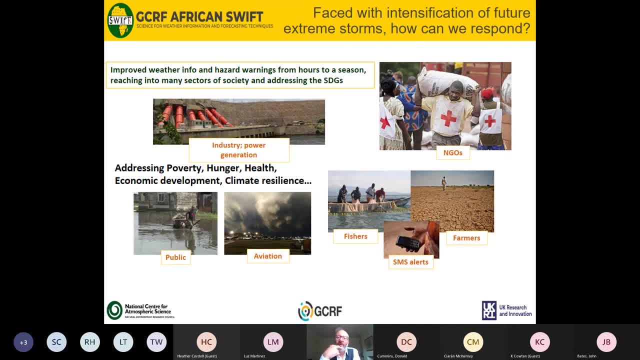 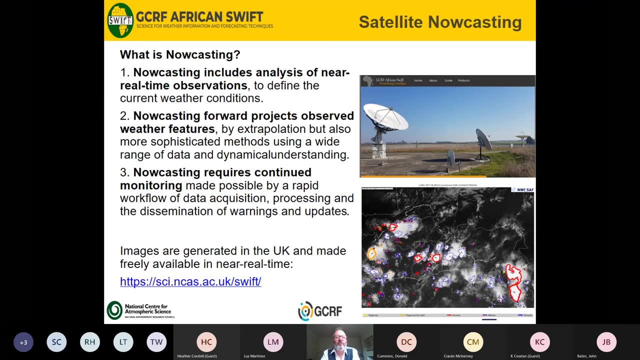 And a lot of that is about increasing people's resilience, And so this project, African Swift, which is one of the GCR projects, is looking at Improving forecasting and information for people on a range of timescales, But I'm going to talk about the extremely short timescale. 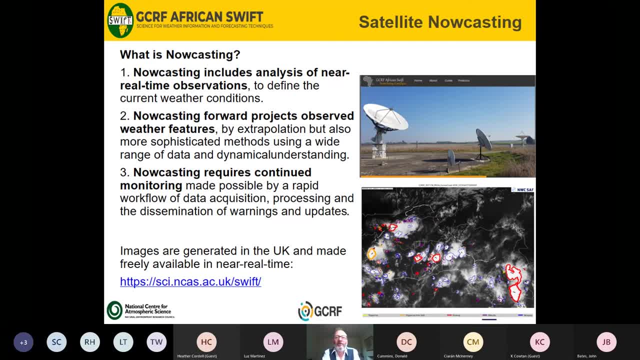 which is now casting. So I'm going to go to absolutely the opposite end of the spectrum of time. So now casting- I mean now casting- is something that's been invented in the US and UK, probably in the 70s, And in the USA it's a big thing in terms of tornado alerts. 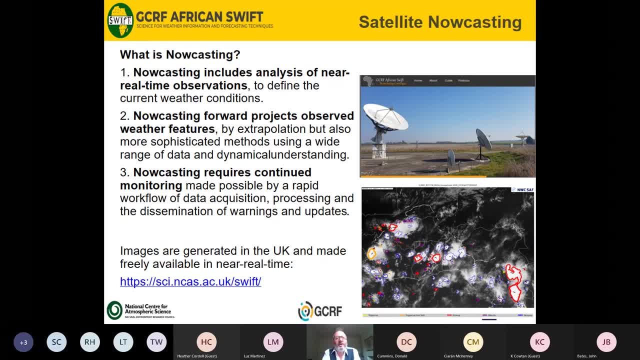 So the principle is that if your weather forecasts are not Not very good- and I missed a slide here, actually I had a slide which justifies this- Just as the climate models of rainfall are very poor, the weather forecasts are extremely poor too. 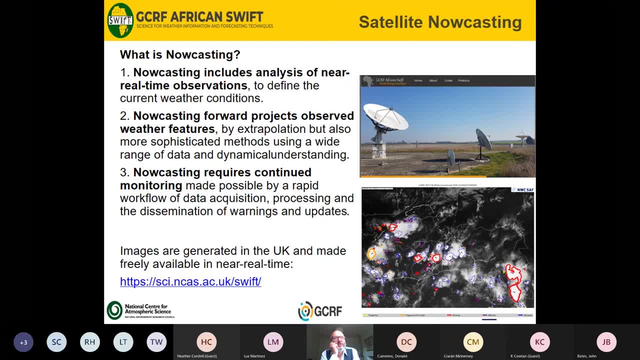 So a 24-hour weather forecast for Africa is no better than climatology. It's unfortunate I somehow lost- I deleted a slide by accident- But there's a paper that I can give you, the reference from 2020, showing this what people have known. 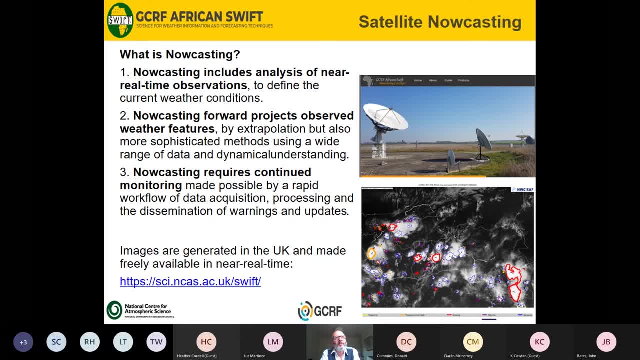 And for a long time. I suppose that, in fact, the 24-hour forecasts, even bias-corrected ensemble forecasts, for most of our tropical Africa are not really better than climatology, which is to say that you'd be just as well saying the rain is tomorrow. 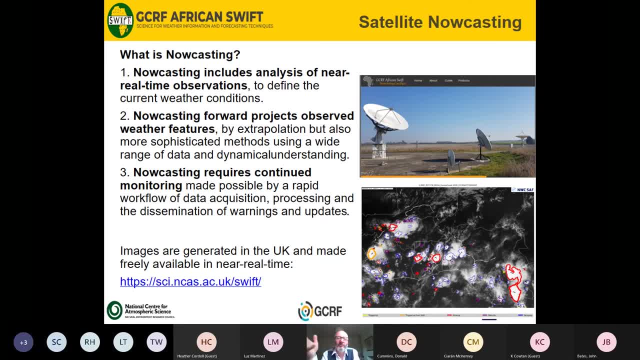 just using the average statistics for climatologically for May- late May- as actually using a weather forecast. So in that environment we wake up in the morning. we don't have a reliable forecast today. We need to know What's happening now and we use the information about now. 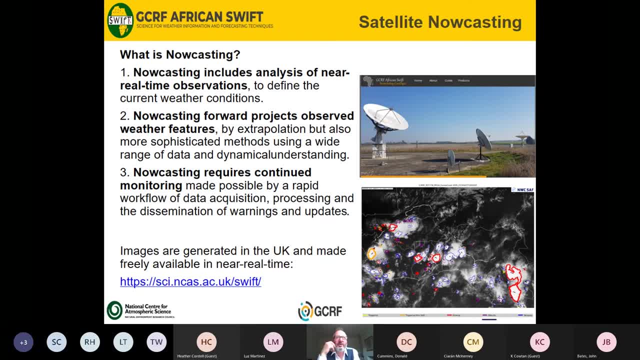 So, as I said, in the States this is the bedrock of tornado prediction. You see storms happening now and you look at the characteristics of those, whether they are likely to be tornadic, and then you send alerts on the basis of that. 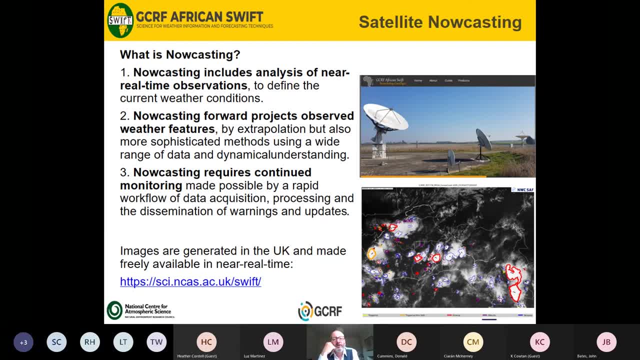 and you monitor them and you project them forward in time as much as you can. So net casting includes these attributes. It hasn't been used in Africa much at all, particularly tropical Africa, partly because radars- and there's some pictures of those on the right- 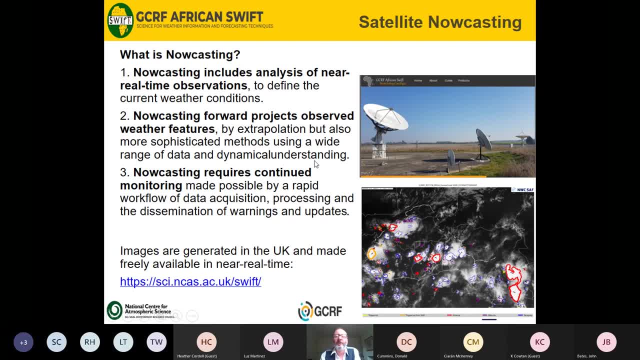 are hard to. Well, they're not all radars in that picture, but there is a radar. They're hard to. So technically, the technology is hard to operate. So in fact, throughout the developing world it's kind of marginal where the countries have the technological know-how to maintain radars. 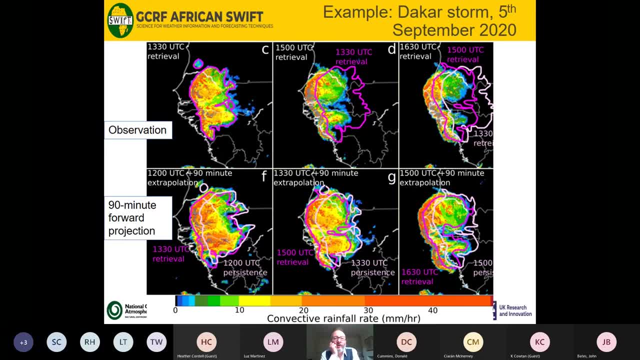 But we have a really good satellite data. So in the SWIFT project we are using satellite data to now cast storms, And in fact we're using algorithms that have been around for 10 years at least, So we're just employing existing know-how. 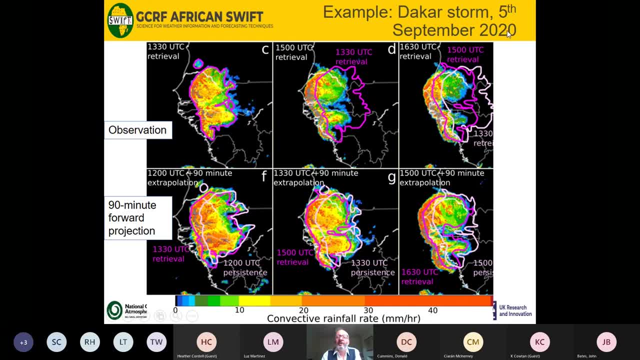 But an example of this is this big storm which caused a lot of damage in Dakar. It absolutely caused devastation in Dakar. So Dakar is the city in the absolute western tip of Africa. here earlier, well less than a year ago- 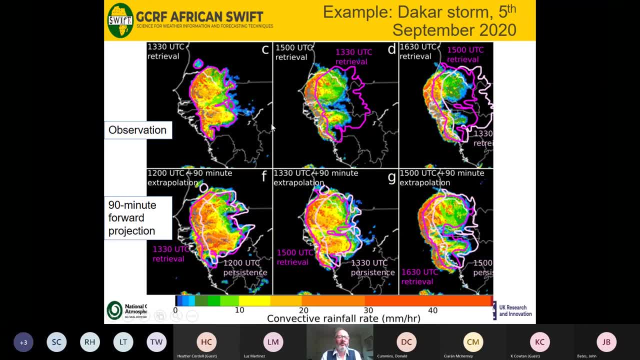 And the point is these very big storms that I showed you in that first movie, a lot of those- last for many hours And in fact they move at a steady speed. You know they're quite well-organized and coherent, So you can see this case going from. 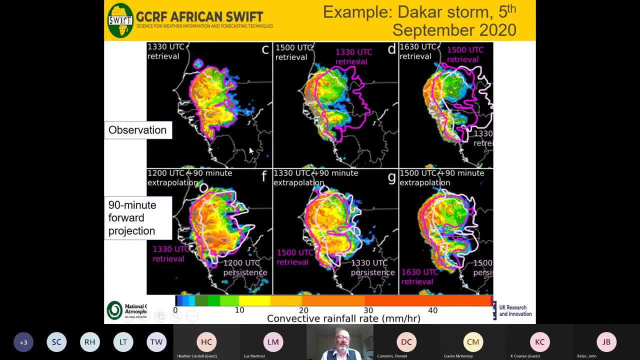 It goes left to right, it goes forward in time And actually what a now casting system can do is just forward project these And of course, many of us do this by eye. If we look at radar data- you know I look at the rainfall radar data- 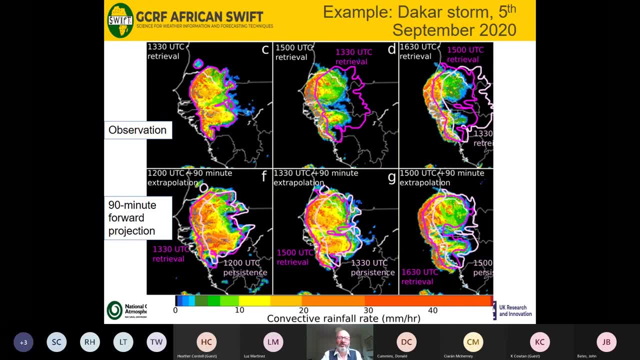 if I'm cycling home from work, just to decide if I can dodge a shower, you know. And so this is what this system is doing computationally. So the bottom row is just a forward. I say just, it's an algorithm which is projecting the top row forward. 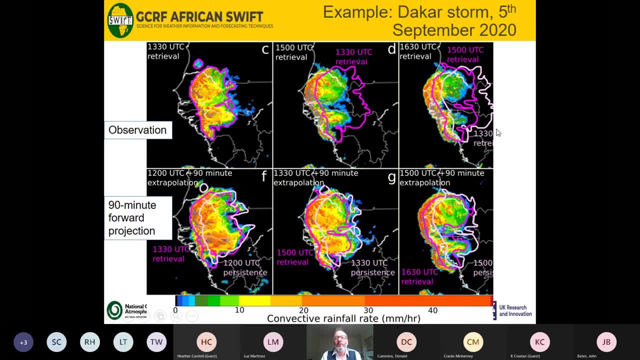 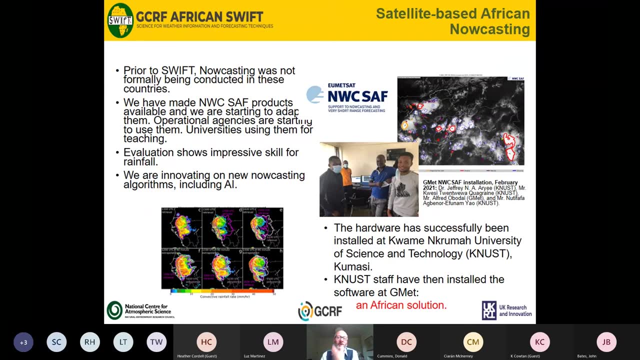 And they're shown. It's the same validation time, So the storm moves steadily across the ocean and an algorithm is able to capture that quite accurately with useful accuracy. So we are implementing this and we've got this solution going- We're running out of leads at the moment- and got it available on a web page. 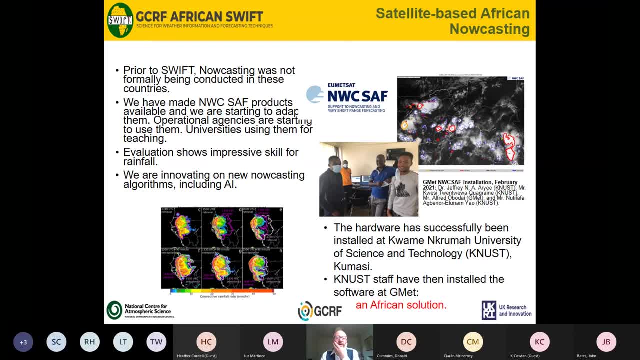 So our African partner institutions are starting to use it. But in parallel with that we're getting the system set up within Africa And we're particularly encouraging university operational partnerships here, because the universities actually hold a lot of know-how, particularly when it comes to technology. 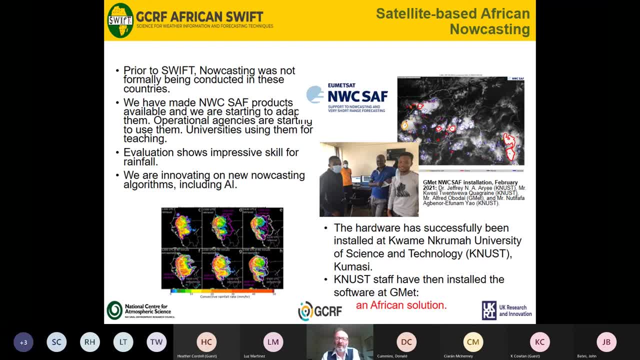 You know they've got lots of young people who are good with computers and you know like fiddling with the internet and sorting out, you know, solutions. So in fact, partnership between the university and the operational centre can keep the operational centre, you know, sharp and up to date with the solutions. 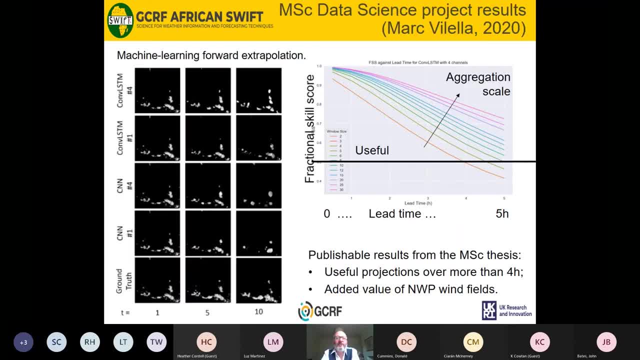 And we're going to move on And we're also doing research on this And actually there's just loads that can be done on this And you know we need more mathematicians and data scientists and statisticians to get interested in these kind of problems. 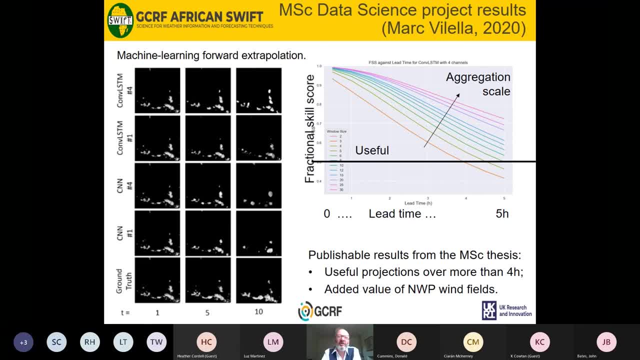 I have to say that you will be competing with Google. I didn't put a slide in about this, but Google published something recently and they're working on this problem too, So we can't compete with Google's computational firepower. I don't think. 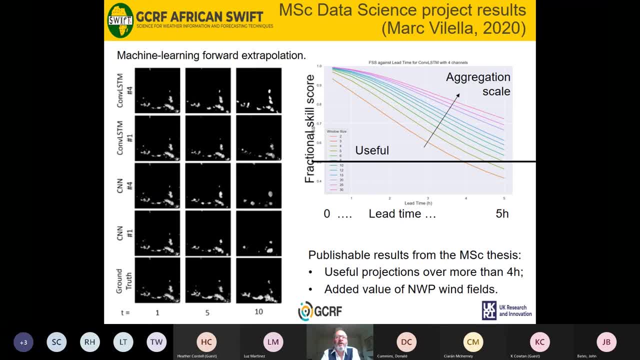 But hopefully we can compete with them intellectually. So there's actually a master's student I had last year and in a ten-week project he did this really nice example where he looked at a number of machine learning algorithms And there's this array of solutions here that the first one is well, 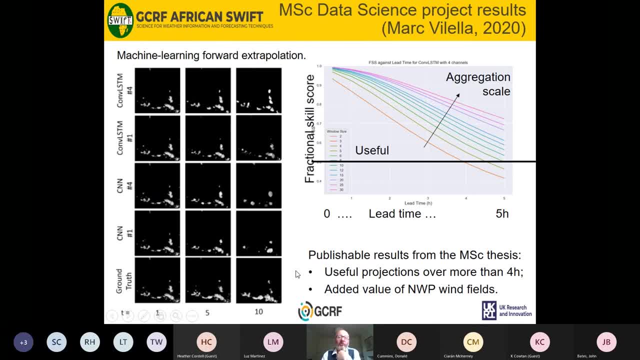 one time step is the left-hand column and then ten time steps is on the right. So that's a five-hour forward projection, And his best algorithm is the top one, which produces something which, well, I'll say it's pretty good, and I'll try to quantify that by saying that we can see certain, you know. 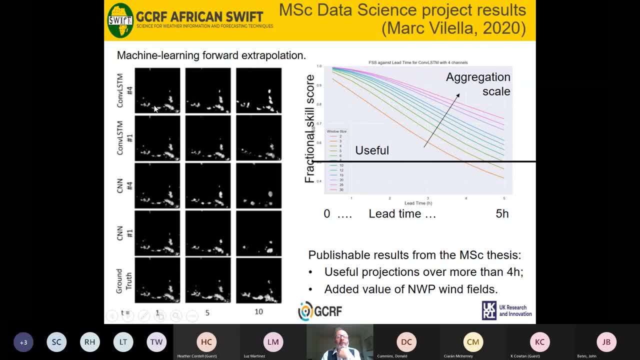 you can see certain items and features in this which are captured faithfully, whereas other algorithms maybe blur them out or lose some. So there's a lot that can be done And this stuff is useful and it can save people's lives. You know, with five hours warning people can corral their cattle. 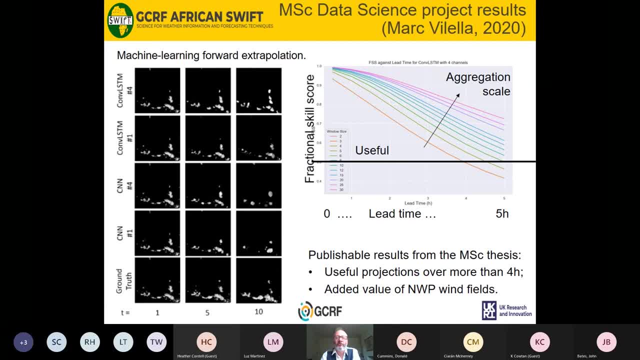 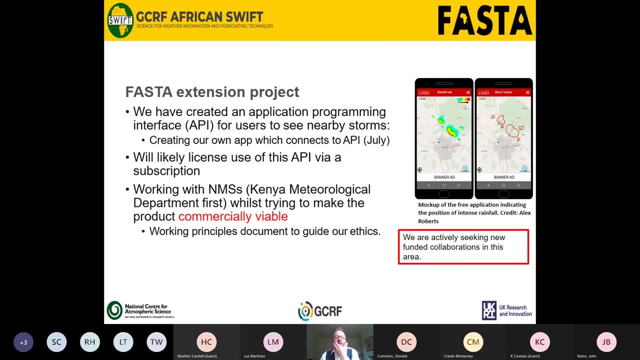 or they can protect their children or whatever, or all sorts of things they can do. So just to say that it's all within our reach And there's a lot we can do. At the moment we're also trying to get this into mobile phones. 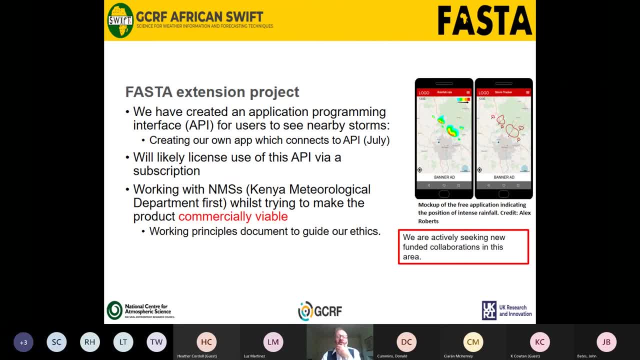 So we've written an API and we're trying to get an app together, which hopefully will be done in a couple of months. We're working at the moment with the Kenya Meteorological Department and trying to make this commercially viable, in the sense that we ought to be able to get funding. 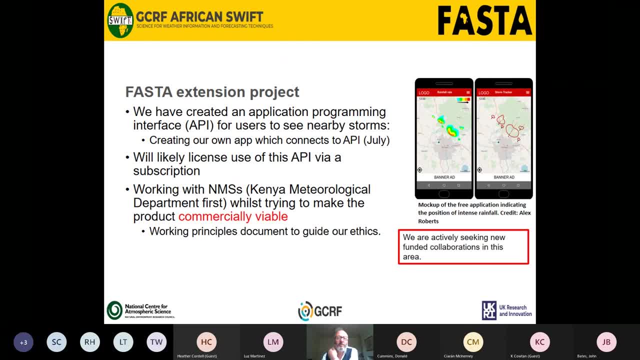 from commercial or private sector organizations, for example tea producers And who are interested in protecting their supply chain, So we can get information to economic concerns that can benefit from this. So hopefully- well, this is early days, But hopefully- we can start to get commercial income from this. 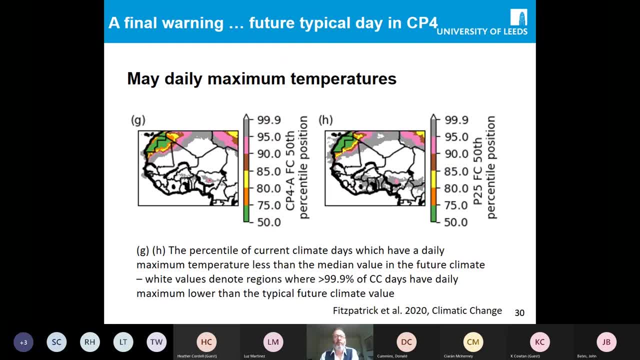 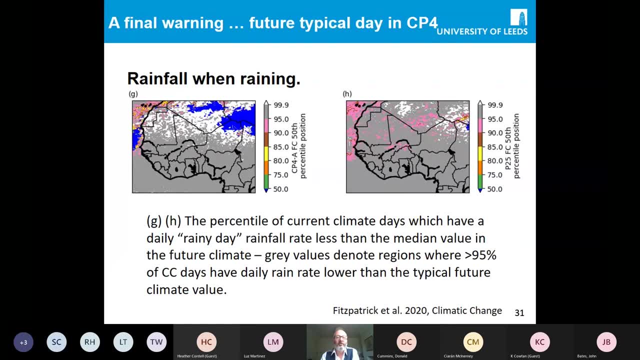 So, just looking at the clock, I had some, you know. maybe I'll just move on. Maybe I'll just show the last version. I'm talking about rainfall. This is going back to the climate models. This is a way of looking at the rainfall. 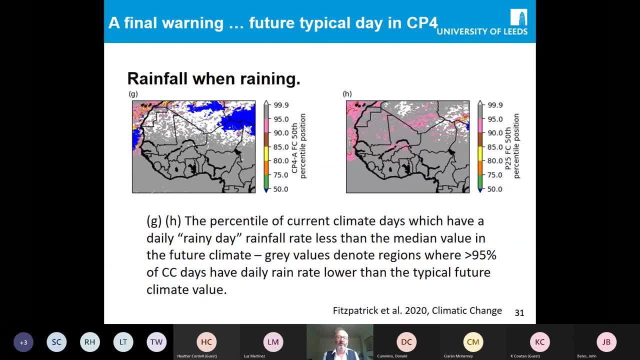 You know people, people are concerned about increasing temperatures, but they often can't translate it into their own environment And actually what matters in these marginal climates are the extremes. So this is a way of looking at those, And there's two models here. 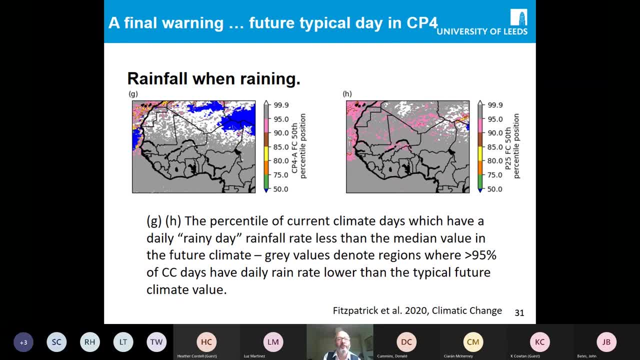 And the left hand one is the CP4 model, the state of the art model, So we can focus on that, And what this shows is the percentile of the- let's think it's the percentile of the future climate distribution at which. 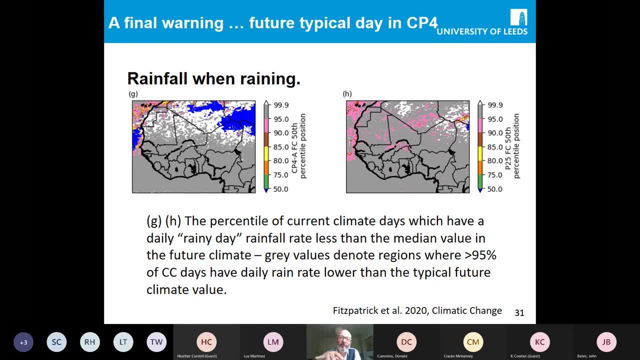 no, sorry, it's the percentile of the current climate distribution at which the median of the future climate sits. So where this is grey, this says that the future climate median sits above the 95th percentile of the current climate. So it's a way, I mean, that takes a bit of explaining and it's quite technical. 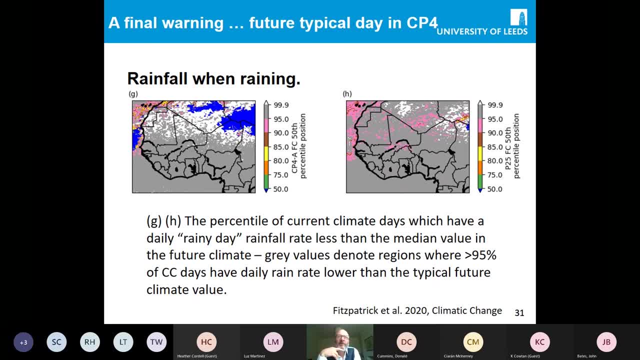 But actually you can translate this to a lot. many people are saying that you know the future climate norm. the median day, the normal day, is really your extreme in your current climate, So extremes are going to become the norm is a way of translating that plot. 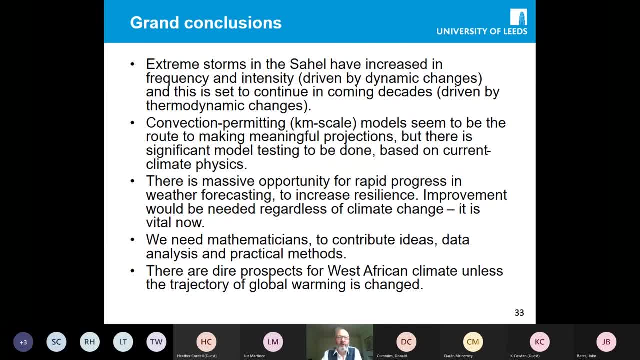 I'll jump over that, So OK, so I'll come to conclusions. I'm just repeating the things I've said. I mean, extreme storms have increased in frequency and intensity. We've got these kilometer scale models which can really help in understanding this. 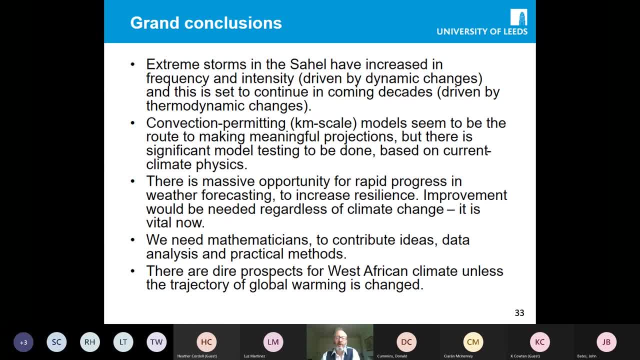 But they also have drawbacks still, And so there's a lot of work to do on that In the current environment. then we need weather forecasting. We're facing the reality of these increasing storms, And there's a lot to be done, but also massive opportunity for doing. 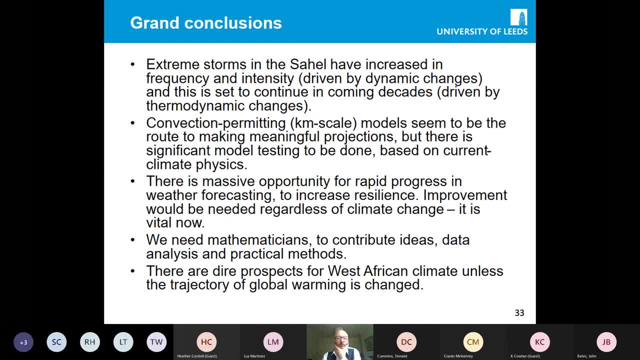 you know, doing the obvious things and doing the simple things now. And the last point was about the dire prospects. So at some point there will be, you know, a lot of intense storms and the norm of the future will be the extreme of now. 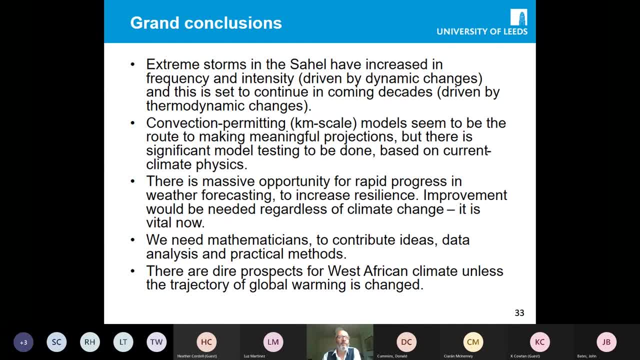 And I think the world has to face up to that. I've got plots I didn't show for temperature and humidity which are equally frightening, And this kind of thing keeps me awake at night, to be honest. So you know it's something the world needs to take very seriously. 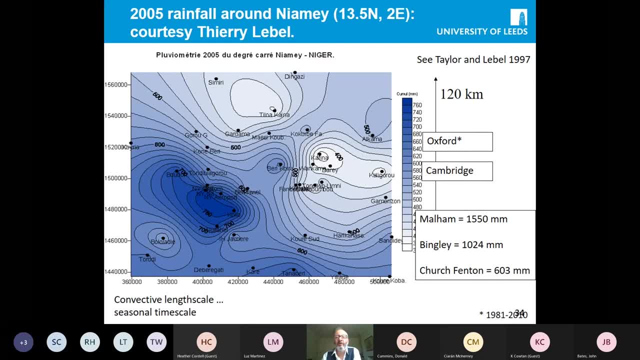 So I will close that? No, I won't. Actually I've got one more slide, which is the rainfall. So I don't know if you all knew this, but actually there's a very strong rainfall gradient across our region, So actually Malham, if you compare Malham and Church Fenton. 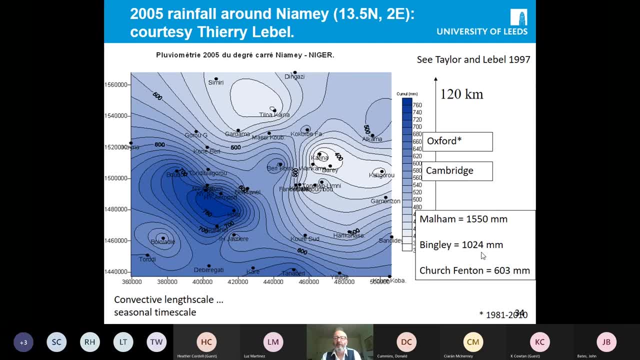 so Church Fenton in the Vale of York has less than half of Malham and sort of nearly half of Bingley. So actually when Andreas Fink comes to town, when he comes to visit you know, when he asks you about the rainfall in this region. 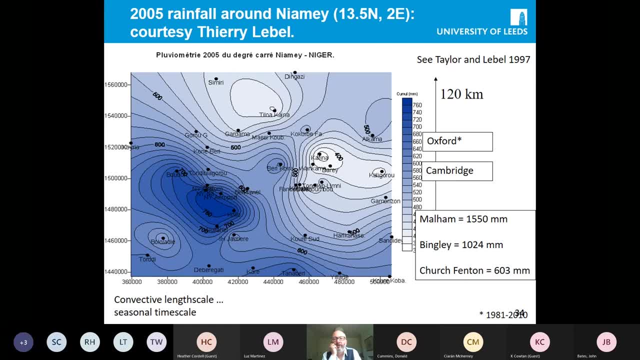 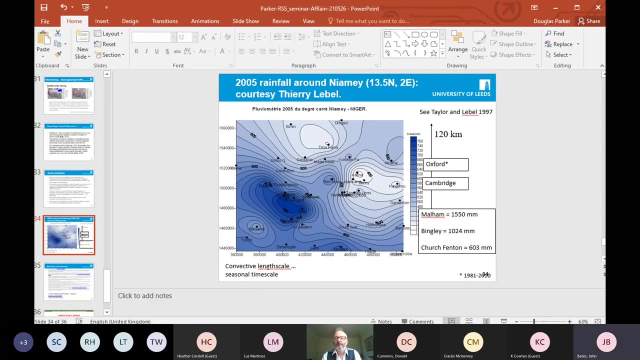 then it's really got an interesting gradient And actually it's probably got a lot of very local variability in that. So you can give him an interesting answer And then I'll close here. That is absolutely brilliant, Thank you. Thank you, Douglas. 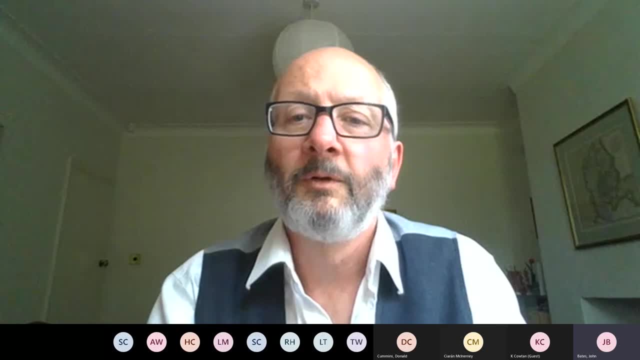 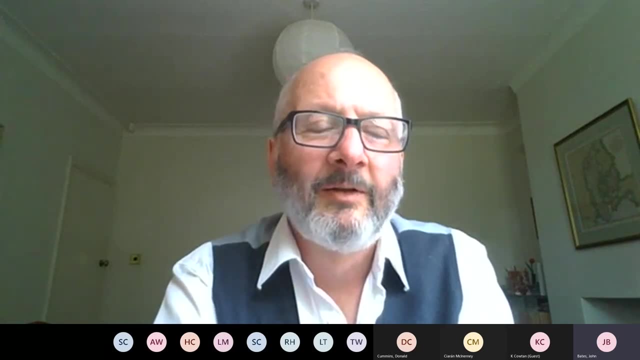 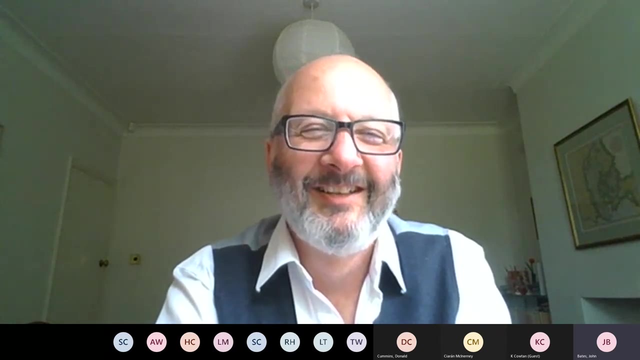 And to the applause team as well. There we go. I was all prepared to hazard a guess at the Leeds thing, which is because we're on what I think was the right side of the Pennines. Generally, we obviously get less rain than Manchester. 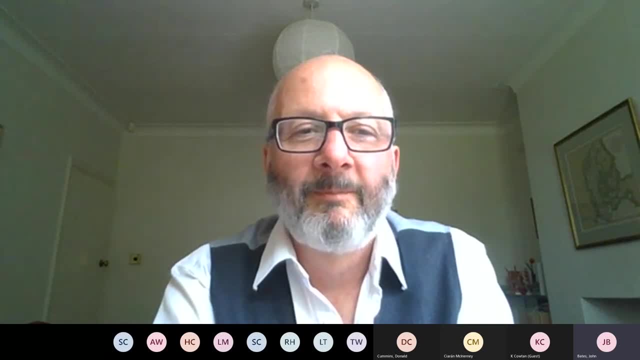 because the weather's moving that way. So my guess was going to be that we have less rain than Oxford or Cambridge. And no, it's not more sophisticated than that. I think it's somewhere between. You know, I didn't have a Leeds measure. 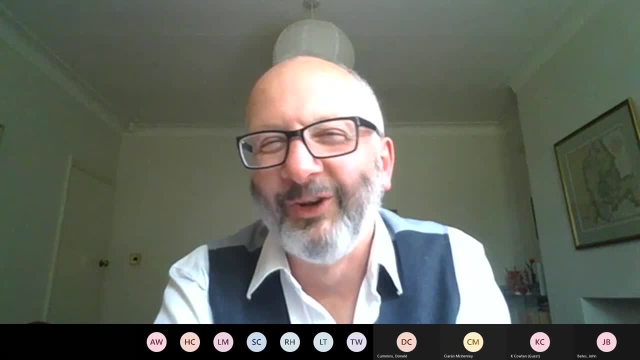 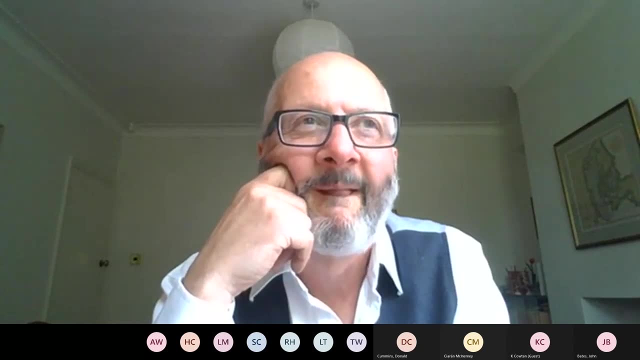 And on the internet I found 805 this afternoon. But basically it's in between Church Fenton and Bingley, So we're on a steep gradient, You know, as you go from Well, I mean Church Fenton and Bingley. 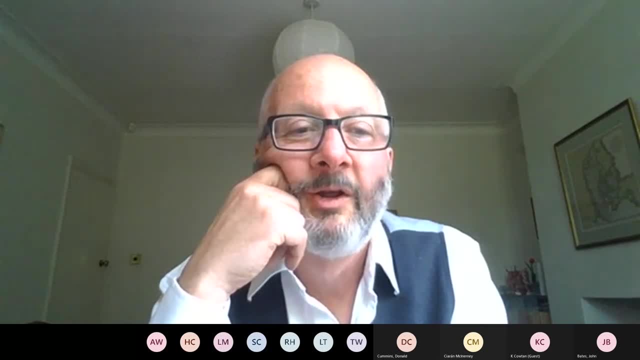 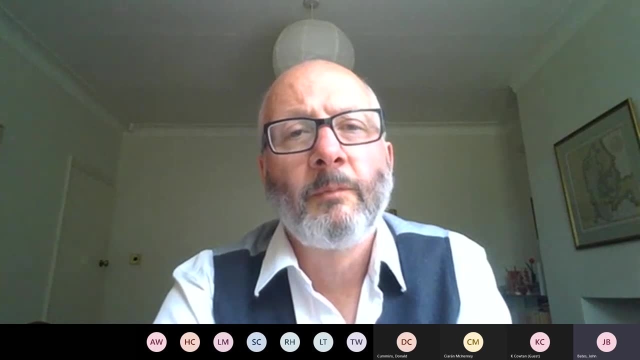 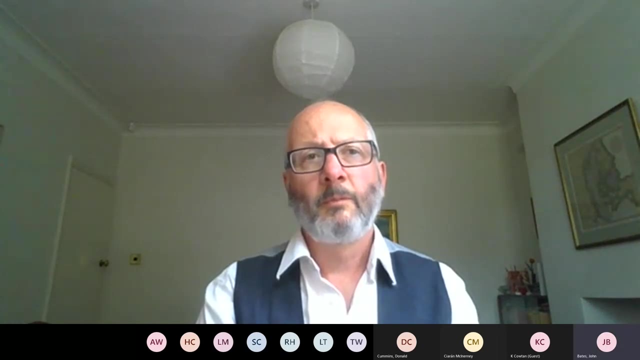 Bingley's probably only 30 miles or so, isn't it? And there's a big, big difference. Yeah, it's really interesting. I think that the I was just going to ask one question, My sense is a bit of a naive question. 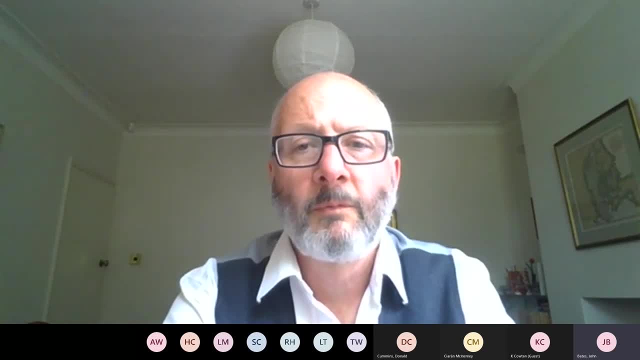 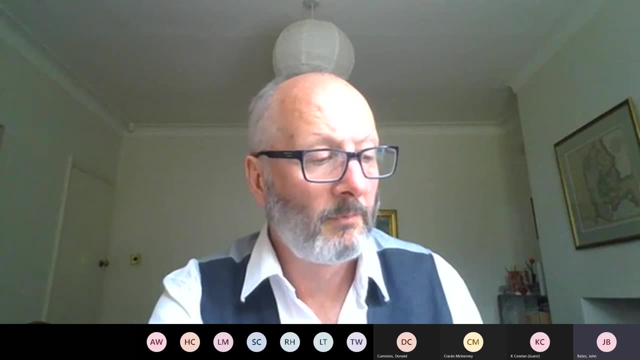 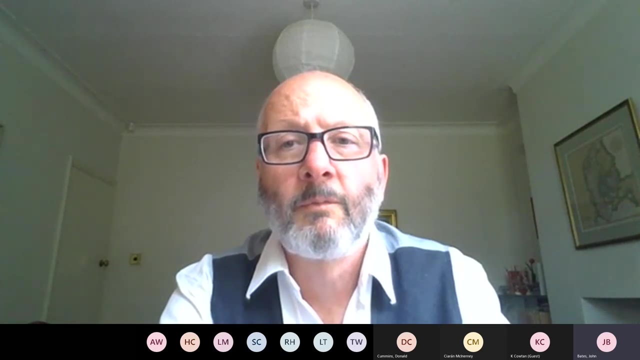 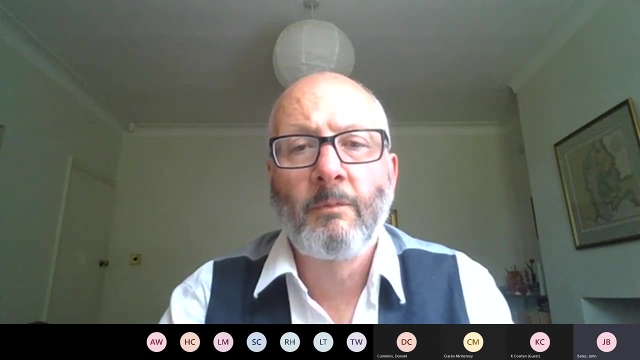 The situation in Africa is obviously heavily driven by the geography. So you've got the mass expanse of desert in the northeast corner And it's a vast sort of landmass without huge water sources. I just wondered how far you thought That this work is sort of translatable into another similar area. 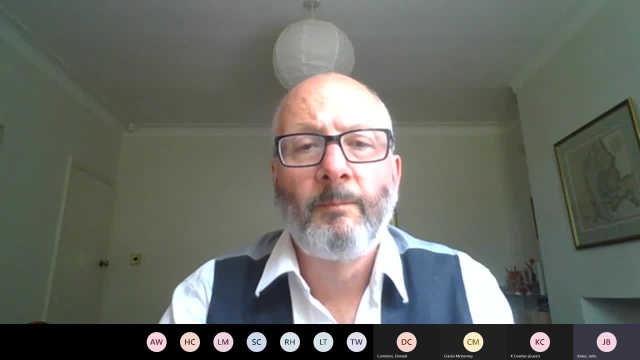 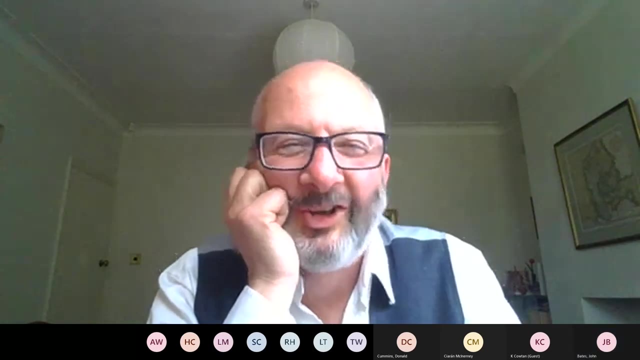 But maybe the southeastern corner of China, for example In the Gobi Desert, Or, in effect, we end up needing models for each different landmass. Yeah, that's a really good point. In fact, we have a proposal to NERC at the moment to ask exactly that question. 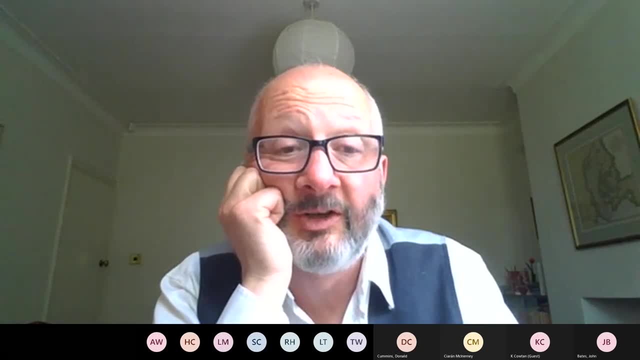 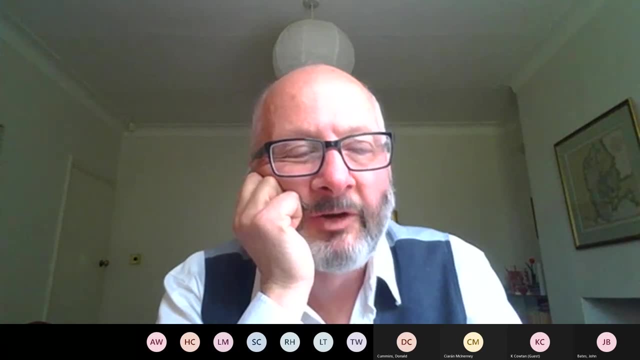 And to try and translate this. So in principle, we can use the satellite data globally, the different satellites, But we could do the same analysis globally. So we've got a proposal to do that. I think that the African rainfall, for some reason which is a bit of a mystery, 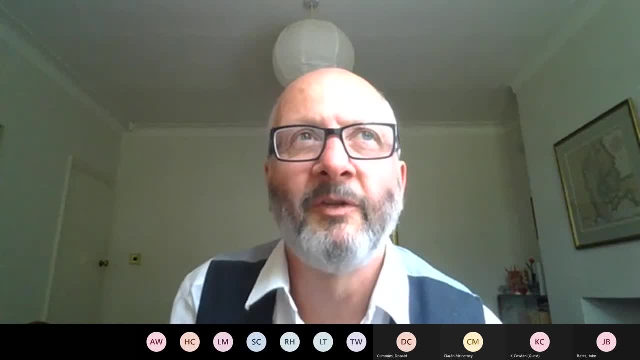 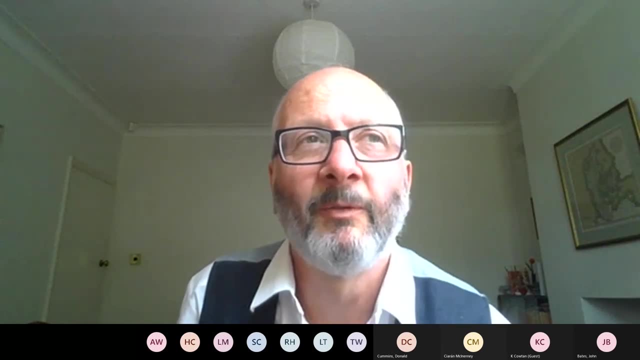 I mean, if I went back to one of those maps, it's predicted worse for tropical Africa than the other continents. So the other continents the daily rainfall is better predicted. We don't know why that is. I mean, what's special about Africa and the tropics? 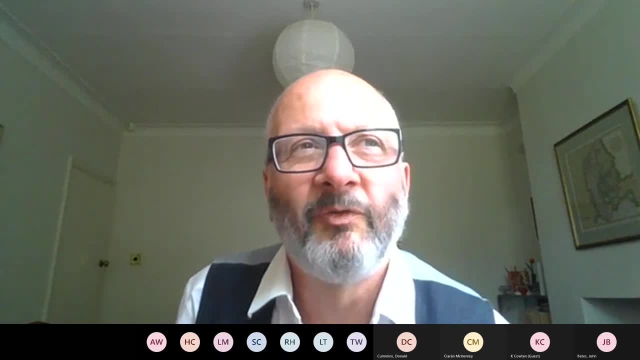 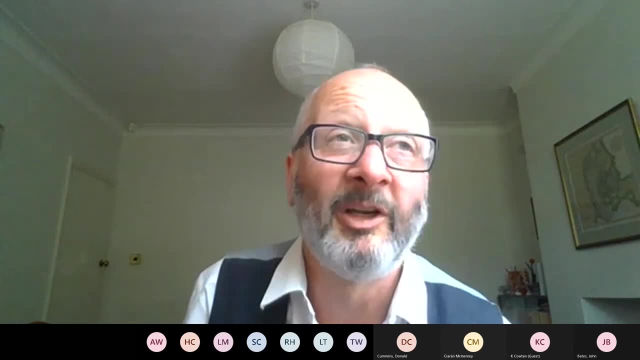 But we've got some guesses. But when it comes to the sort of seasonal rainfall, then it's very poor in many of these regions, In the monsoon regions. So Southeast Asia and India- I mean India is a real headache for the Met Office. 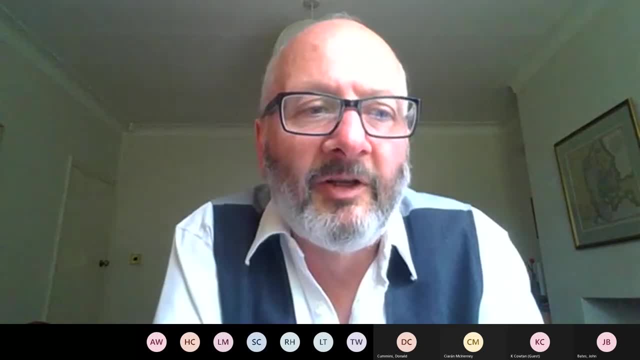 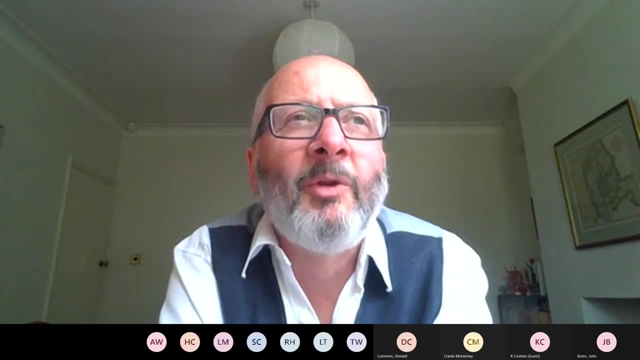 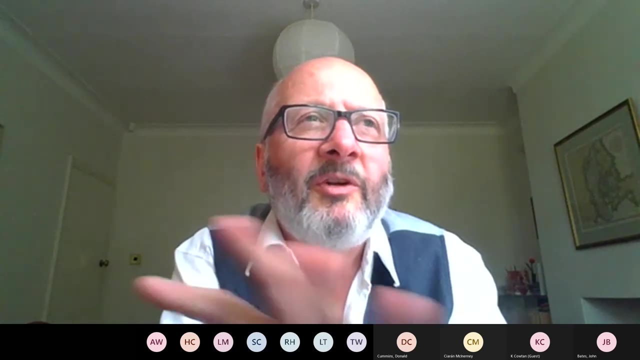 Indian rainfall production. So it's, yeah, I think the principles you know, or the principle thinking, should apply everywhere. But I mean there are certain differences too, And this part of the world has very low topography. So all these climatic gradients, you know, to the Sahara and the Sahel. 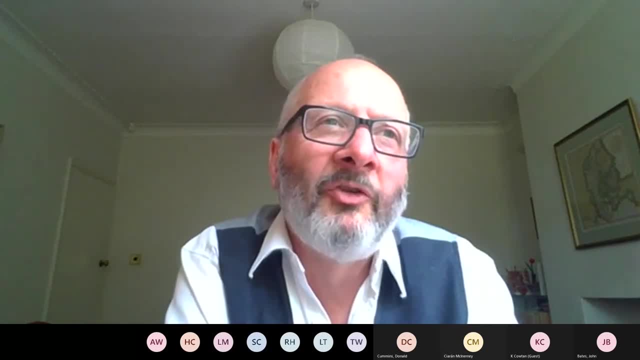 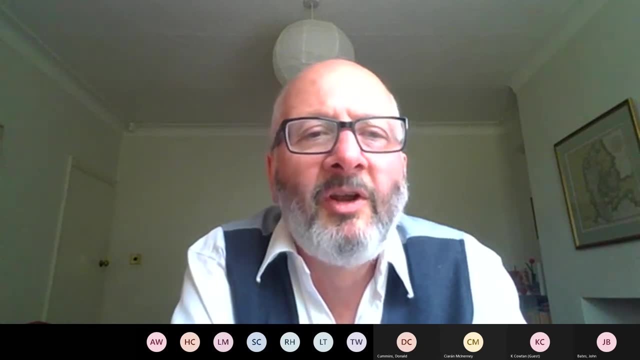 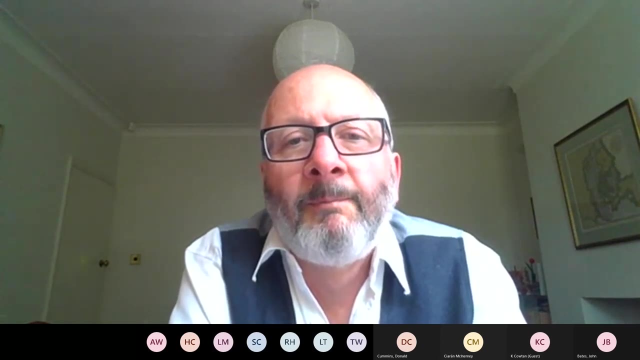 are to do with the climate system and not to do with topography, Whereas if you say, look at India, then the role of the Himalayas is very important And India and China And the coastlines are more complex. So I think there'll be similarities and differences as you look at other parts of the world. 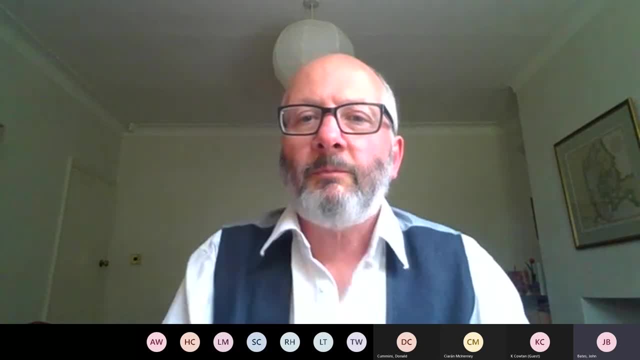 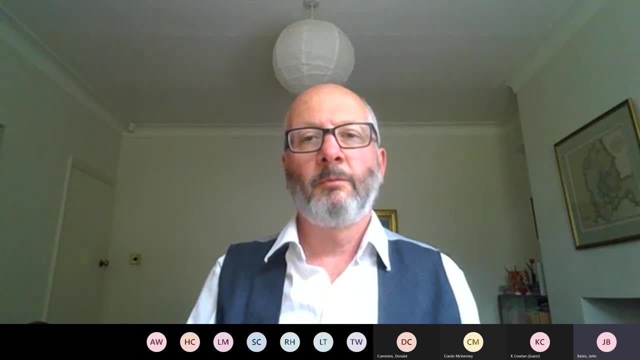 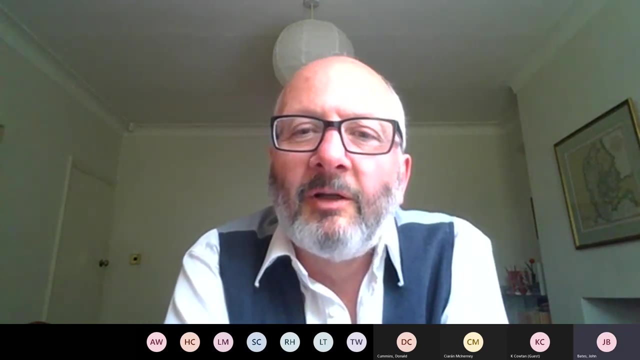 Yeah, that makes sense. So I've got a question from Laura: How you consider how extreme value theory could help demonstrate changes in extreme storms over the decades. Yeah, that is a good one as well. I have to say I'm not entirely knowledgeable at extreme value theory, although a little bit. 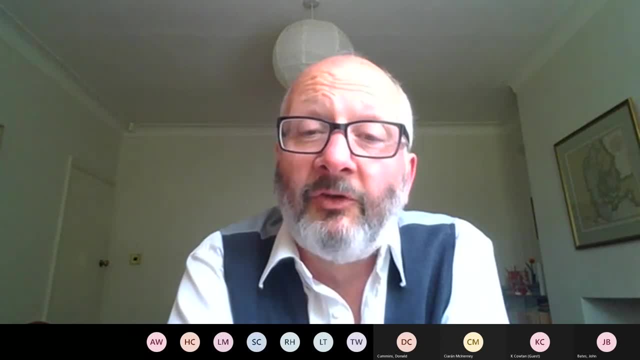 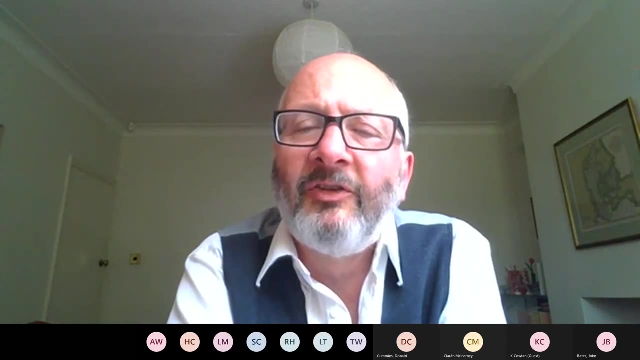 And in fact I had a student project for undergraduate students this year that I very much enjoyed with some very bright students. So one student actually did fit an extreme value, So it's the GEV distribution to some of the data. So she modeled the data with an autoregressive model and then fit a distribution to that. 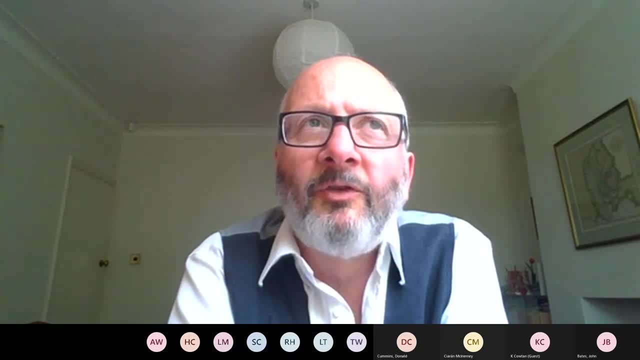 So that produced some- you know, some- interesting conclusions for one location. So, yes, certainly I think that's a good approach. There are lots of really, you know, there's loads of really interesting things to do, And I'm happy to collaborate with people. 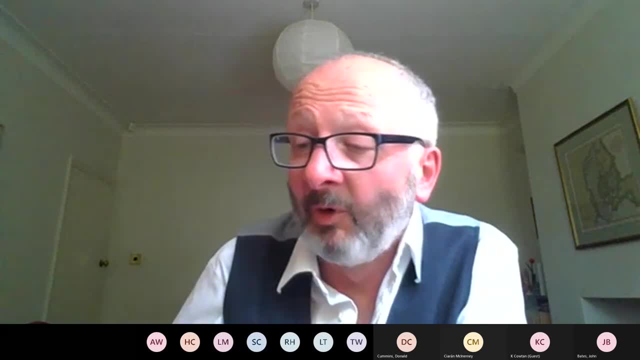 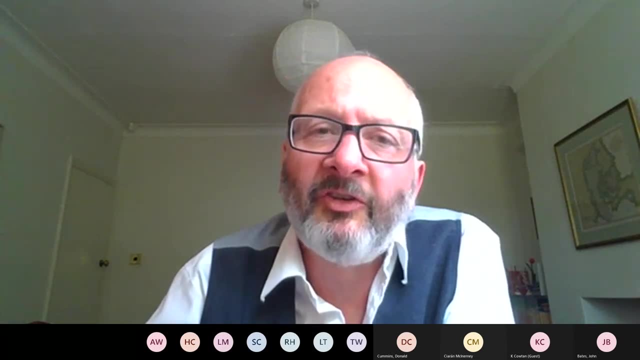 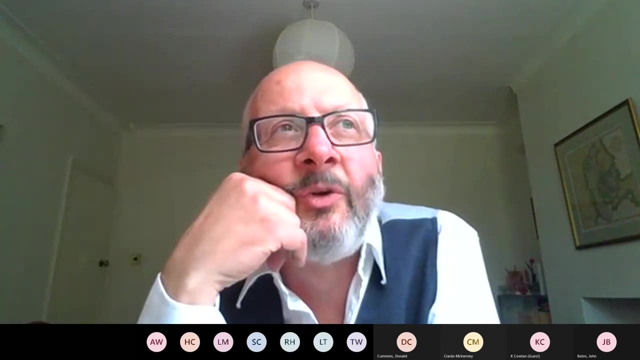 We've got this sensational data set in the CP4 model. We've been working with these people in Grenoble who are, you know, very good statisticians, And what they're doing is constructing sort of storm objects statistically in the data. So we know that the storm is composed of kind of coherent structures. 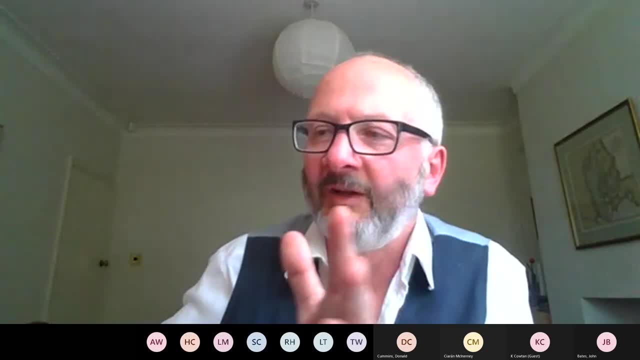 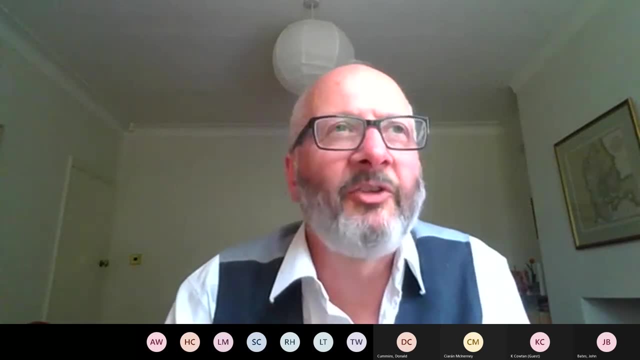 So it comes with a very intense burst of rain that lasts about half an hour, and then a period of rain that's longer, lasting for about five or six hours, And so the structure and shape of that affects the impact. so in hydrology, And then the sequences of storms matter for hydrology or for engineering, 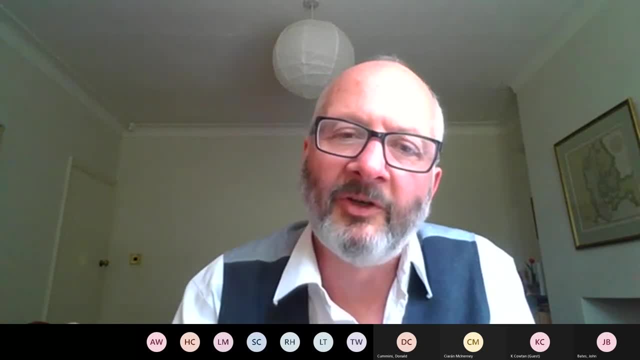 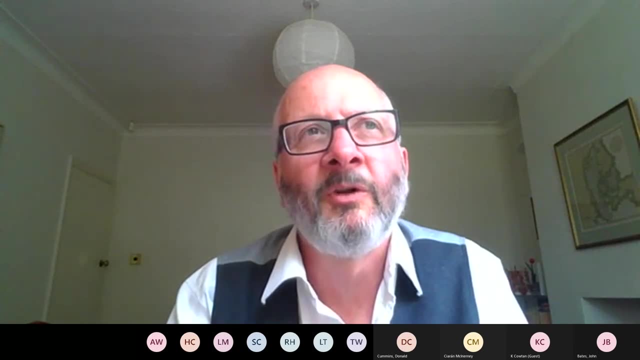 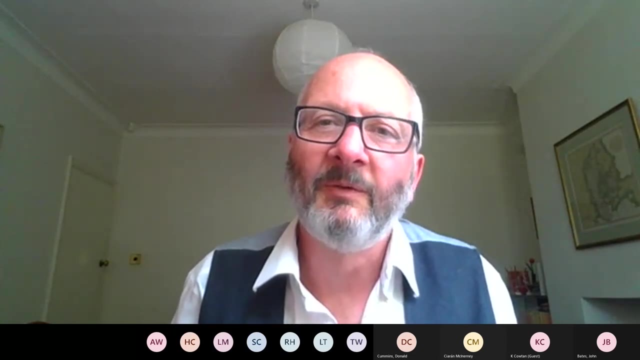 You know, if you get three storms in three days, then the surface gets saturated and you get flooding, whereas one storm on its own wouldn't necessarily cause flooding. So those details of the distributions are really critical. So I mean it's just to say that there's far more that matters than just the seasonal mean, even though that is important. 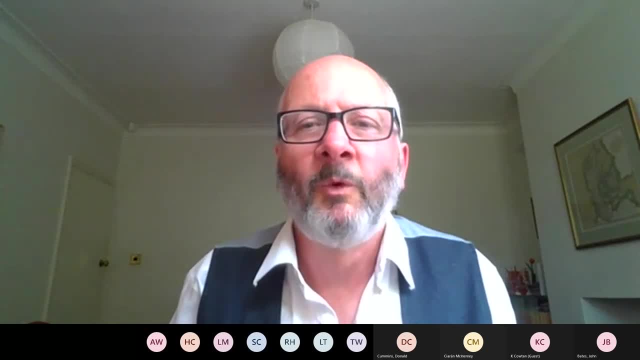 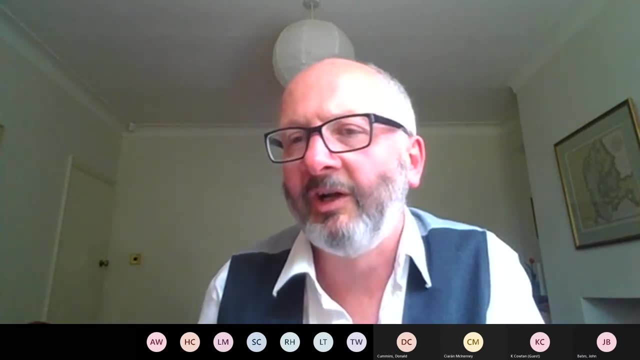 So there's a whole load of really interesting things to do with the data, And all those questions are conditioned, really by what the user needs to know. You know, engineers want to know frequency, duration and what is it? There's three things they want to know.